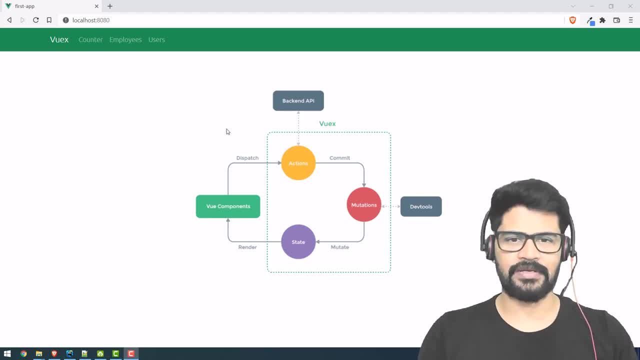 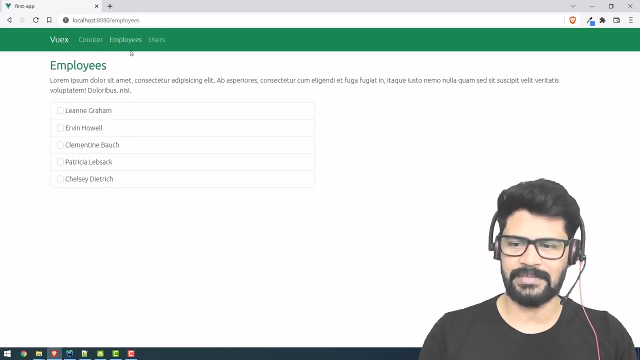 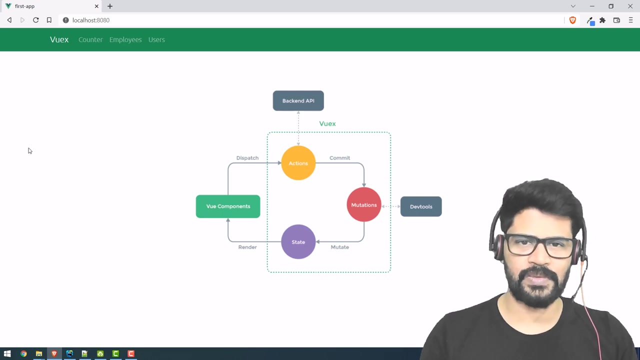 Hey guys, welcome back. This is another crash course on Vue X for Vue JS kind of applications. So Vue X is a library which we can use it for the state management for Vue JS based applications. Okay, so generally in last video we have understand about Redux toolkit. So that is the library we can use it for ReactJS application and this Vue X is specifically used for Vue JS applications. Okay, so same kind of state management. But here it is using a slight different architecture than your Redux toolkit. So here it is using Redux plus the flux architecture. Okay, so this is the architecture diagram of Vue X. But before we jump into this complete architecture diagram. So what I want to say is the last video we have made one example right with React and Redux toolkit. We made an example. The same example I have taken over here. Because three components we have. We have a counter component, employees component and users component for fetching data from server. So I have taken a same amount of component and same kind of architecture and same kind of routing system like the previous video of Redux toolkit. Because if I can tell you in a same example and same component. So you get have a clear idea. How can you make the things with Redux toolkit. 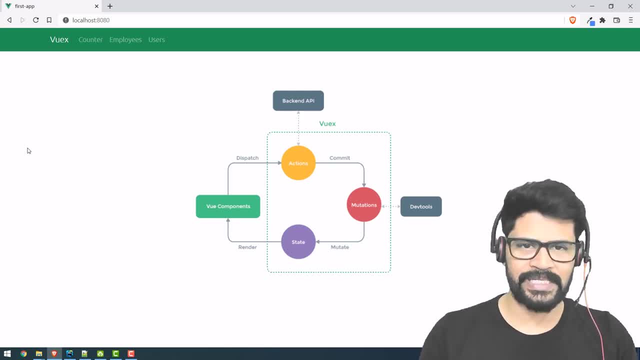 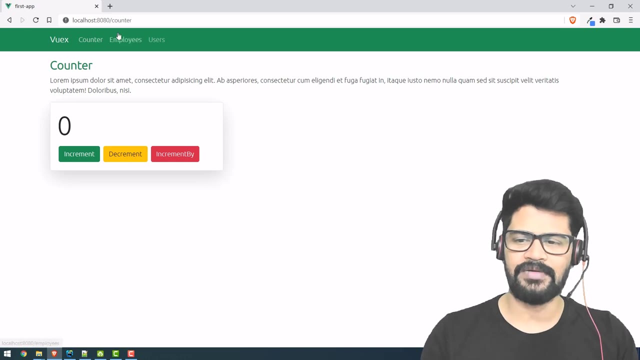 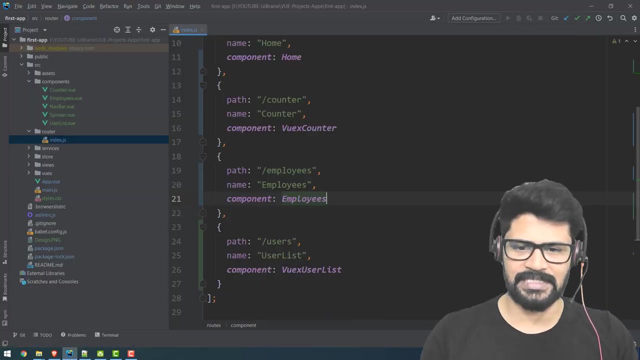 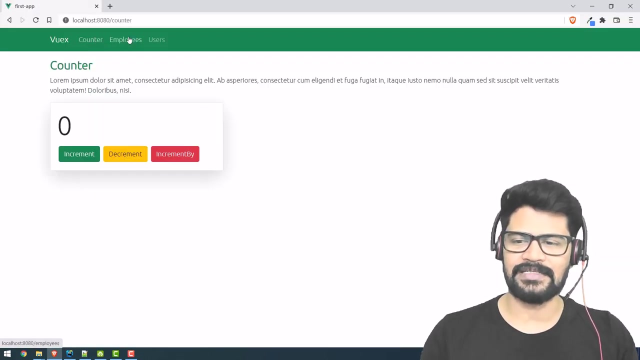 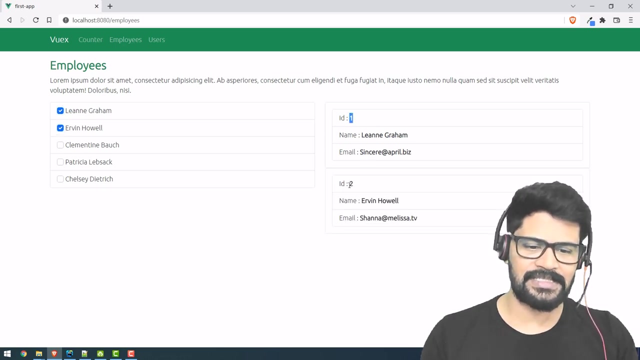 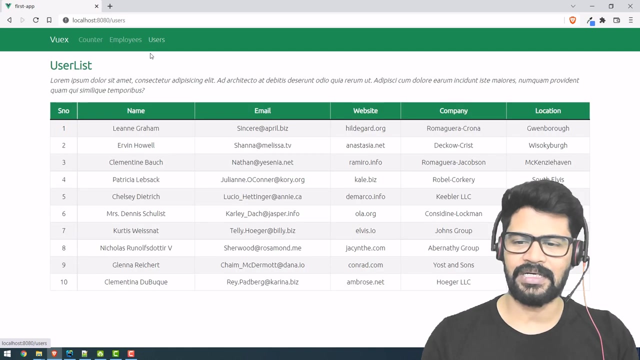 Vue JS and Vue X and also Redux toolkit with ReactJS. Okay, and coming videos we also see NGRX with Angular with the same kind of example. Okay, so now let's have a look here for counter. I'm not using. I think yeah, for employees. I'm not using Redux for counter. I'm using Redux. Okay, so let me check once. I guess. Yeah, counter. I'm using Vue X. Employees. No. Okay. So problem here. Same story which we have understand the last video of Redux. So for counter I have increment the counter. I can decrement or increment by also. Okay, so now the counter value is there. Some state data has changed. Now when I went to employees and came back still the counter value is there because the state is alive because the state is actually not coming from the counter component. It's actually coming from the Redux store. Okay, that's why it is still alive. It's still there even though you switch between multiple other components. Okay, but employees is not connected with the Vue X state management and this is locally maintained a state. So when it is locally maintained state, the problem will be. So when I select a two employees. Okay, so it was selected. So one and two and then I switched to another component and came back. It slaps because it is maintaining a local state. So now what we have to do is we have to convert it to a Vue X state management. Okay, so first what we have to do is we will make this whole application without Vue X and then I'll tell you how to configure a Vue X for the for this Vue JS application. Okay, and also I'll tell you how to fetch data from server. Okay, how to make your Vue JS application connect with server and also that including Vue X. Okay, so here we have a lot of concepts like actions, 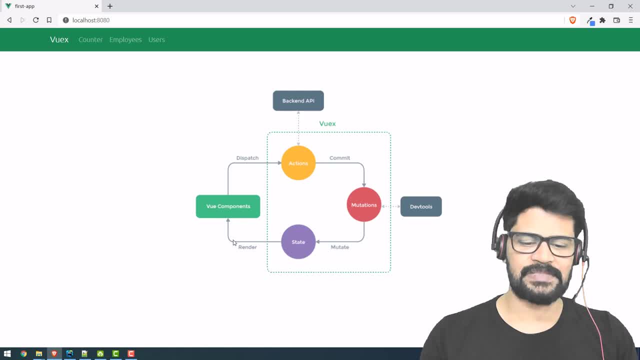 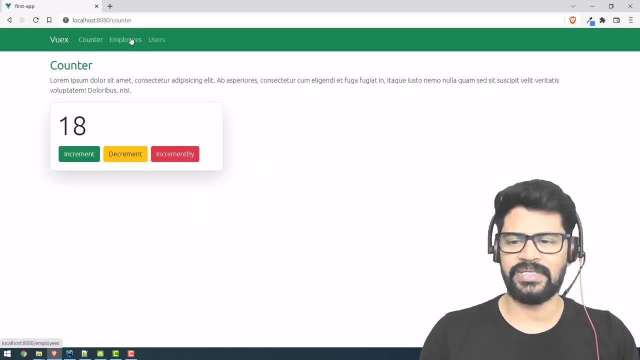 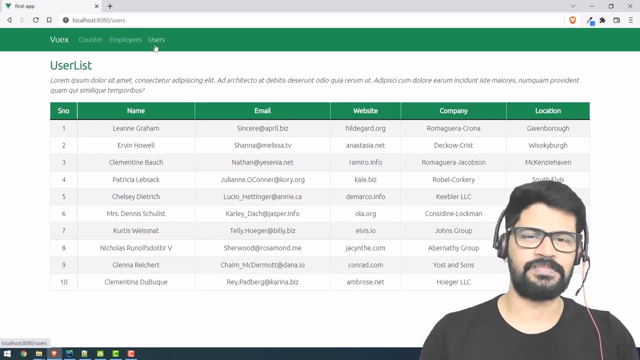 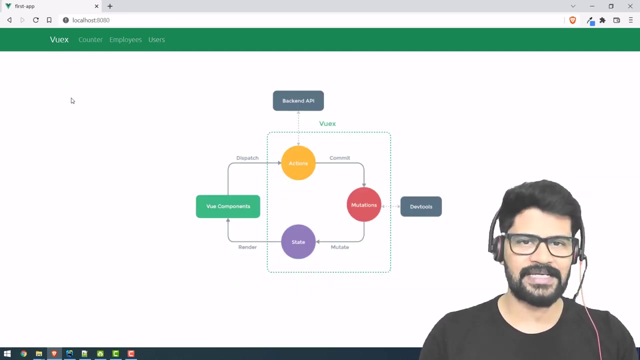 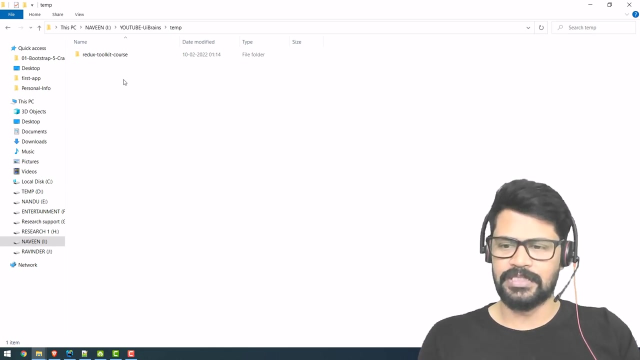 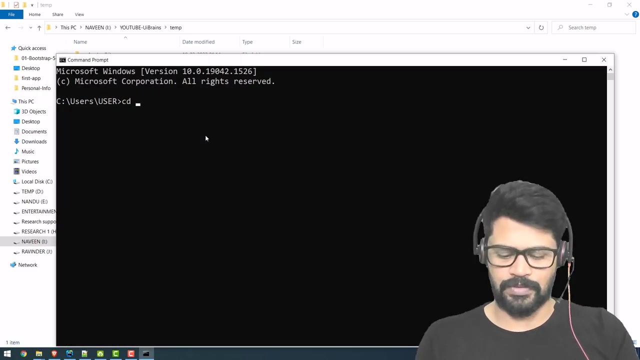 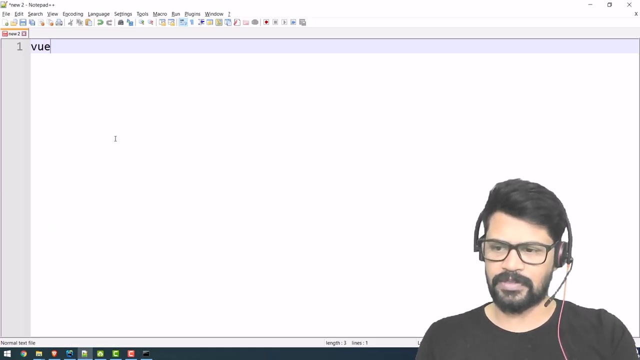 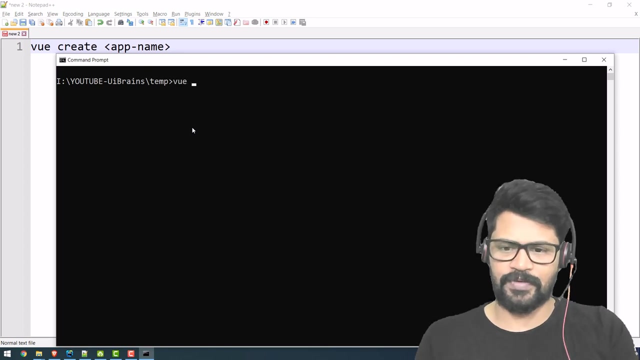 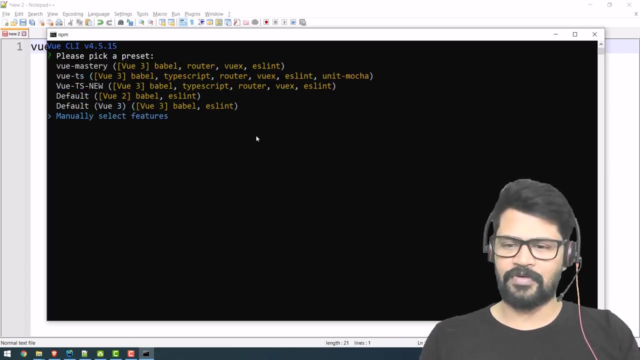 state mutations. Okay, and dispatch and all. So down the line, we'll see all these concepts and the complete flow. I also I'll explain with these three examples. Okay, for local state management, the form handling and also for fetching data from server. So please be with me for this entire video so that you will get a complete understanding of Vue X architecture for local state management as well as the state data which we can receive from the server. connections as well. Okay, so now let's start first, how to create this application. And then we'll start off with the local state management and then we'll convert convert to the Vue X. So let's start. All right. So now to create a project. So what I will do is I'll go to the folder and here I'm going to create a project. So I'll just take a copy of the path I open command prompt. In this I go to this location. I drive the command to create any Vue JS project is Vue create and your application name. Okay, application name. So I'll do like Vue create and our application name goes to be Vue X crash codes. Okay, and just enter. Okay, so you get these type of options, Vue mastery and all but if you don't get these options, don't worry, you can select the one manually select the features. So you can select for manual. And here I need a router, you can just give a space over there and Vue X. And yeah, that's all. Okay, so choose you can I'm just selected Babel, not TypeScript. I selected router configuration and also the Vue X configuration. 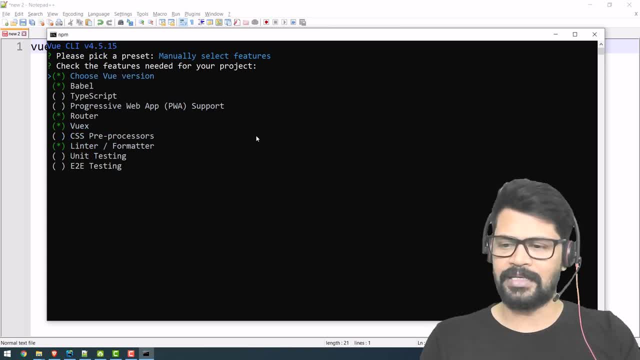 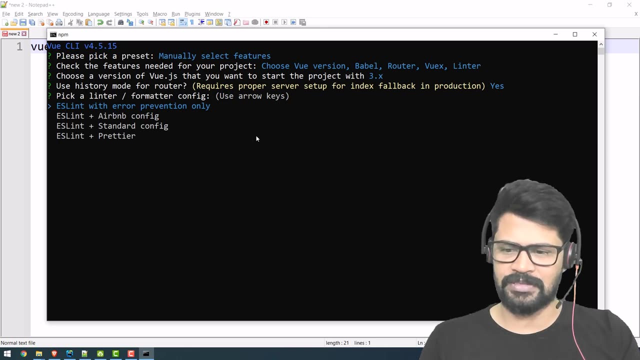 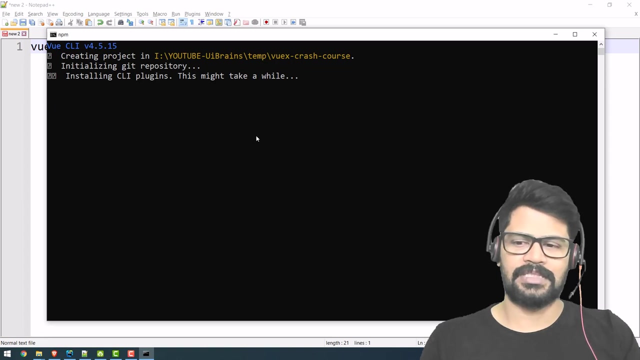 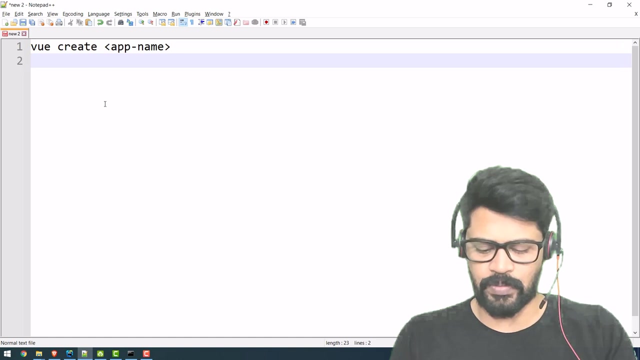 And that's all no unit testing nothing. And, and go back to the viewers Vue JS version. And you can select the three point X. And yeah, so use history mode for router. Just say why? Yes, linked with error prevention. Yes. Okay, yes, linked on save. Yes, dedicated configuration file. No, I select the package or JSON. You want to preset the future? No. Yes, enter. Okay, so depend on your selections, it will create the complete project structure for us. So which create a default folder structures routing configuration and Vue X configuration. So based on that will develop. Okay, so we have to wait for a few minutes. So we got the folder structure ready. And so now we have to install two packages. One is 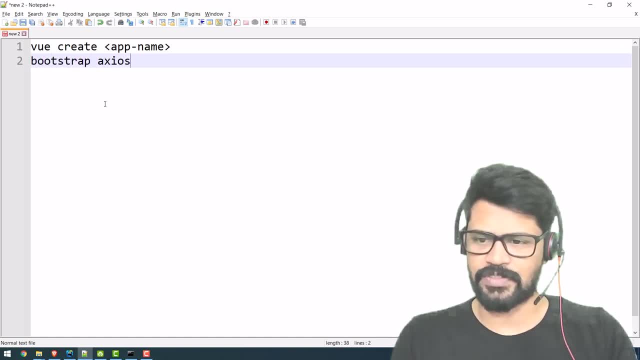 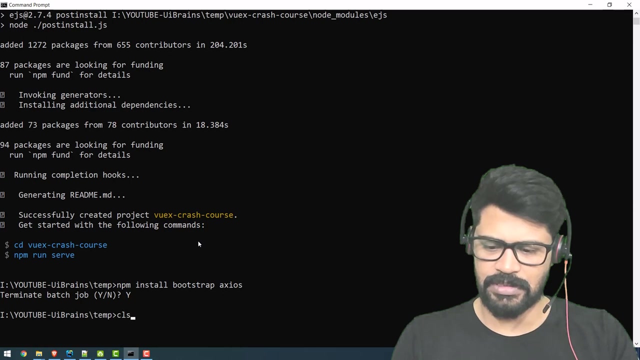 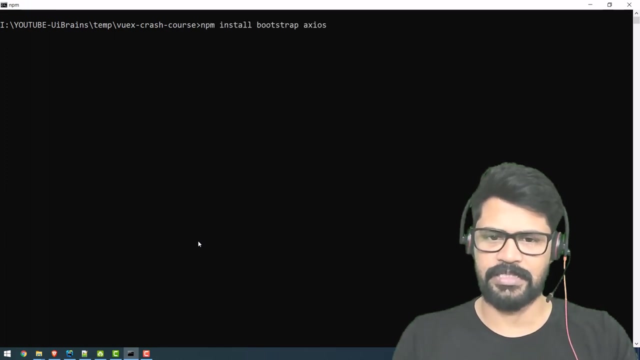 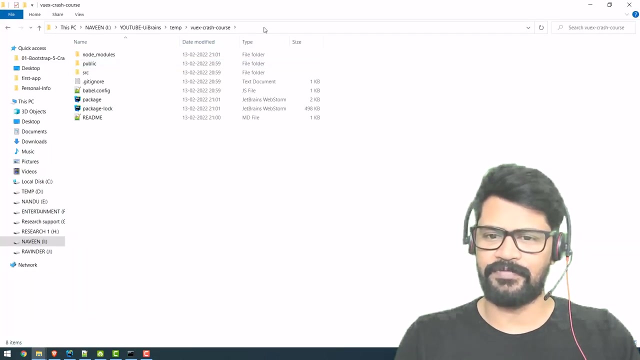 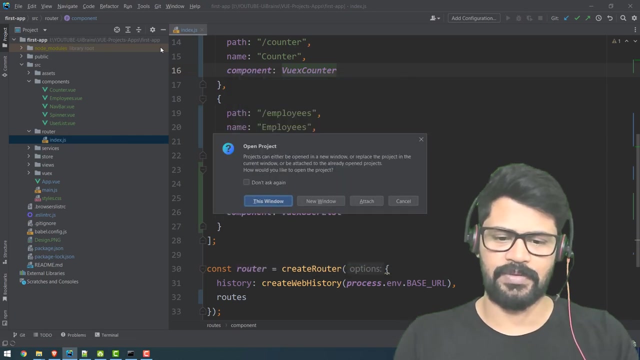 bootstrap. And also Axios. So bootstrap, because we will be using the front end libraries bootstrap and Axios for fetching data from server. Okay, so we don't need to install Vue X and all because based on the configuration, it was already done. Okay, while creating the project structure. So these two we have to install the say npm install, bootstrap and Axios. So let's copy this path back here, paste. Sorry, sorry, sorry. You need to go inside Vue crash course folder structure and then paste it enter. Okay, so it will download and install bootstrap. Okay, so it's done. So now let's jump into the folder structure. Yeah, Vue X crash course. Let's copy the path. Go to your editor, file open, paste. Okay, and okay. 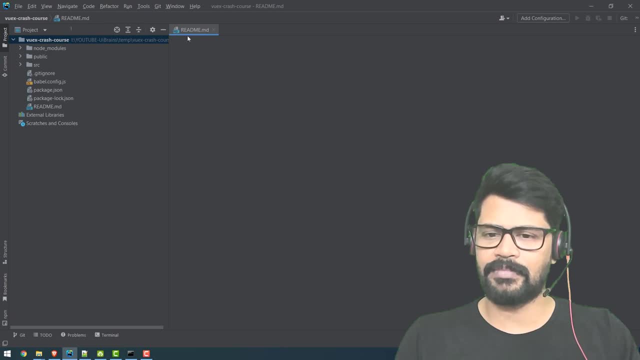 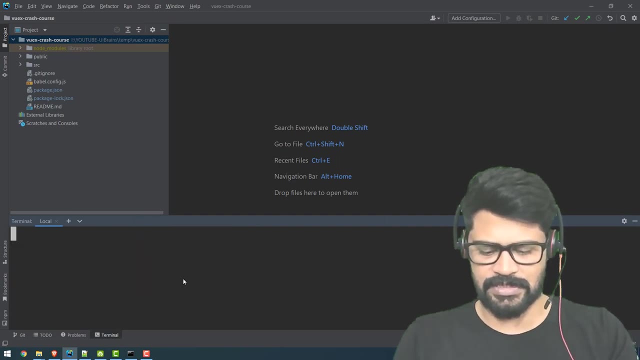 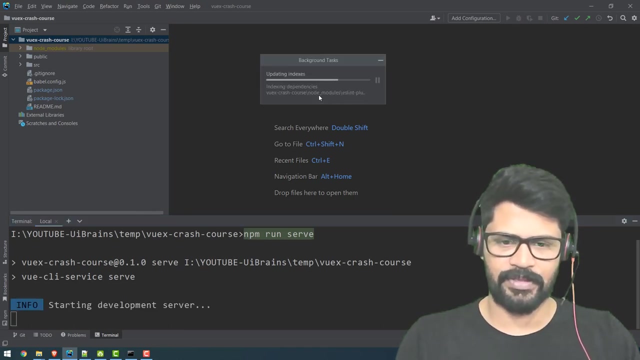 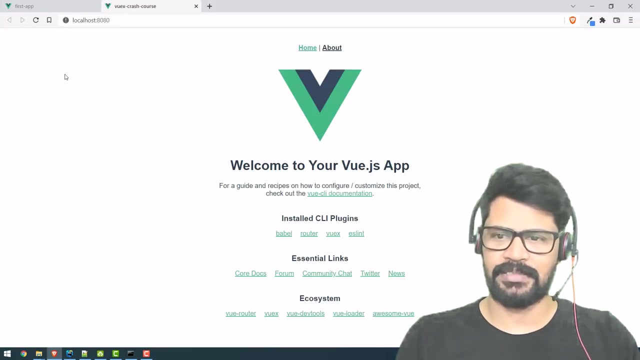 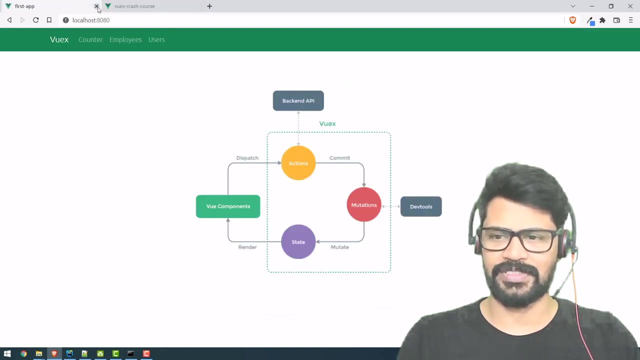 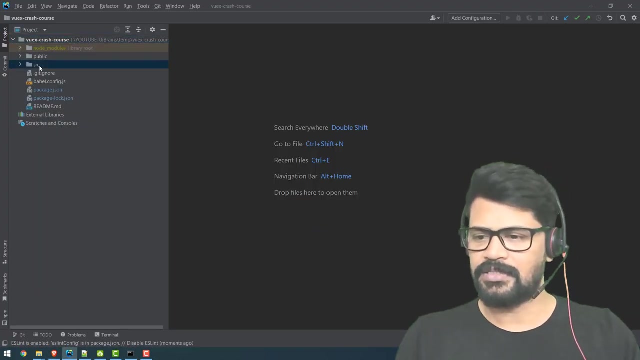 Okay, so now you got the project structure is ready. Now let me run the server once. Let me run the application first. npm runs is a command. So it runs on a port number 8080. So let's wait for it to start. I think it's still indexing. I think it's take some time. Indexing has to finish. And then click OK. start of your server okay starting okay started and this is my uh the default structure which contains already the routing system and all okay we need to make this application that's fine leave it okay and now first of all we need to clear the things which we don't need so first i go to src 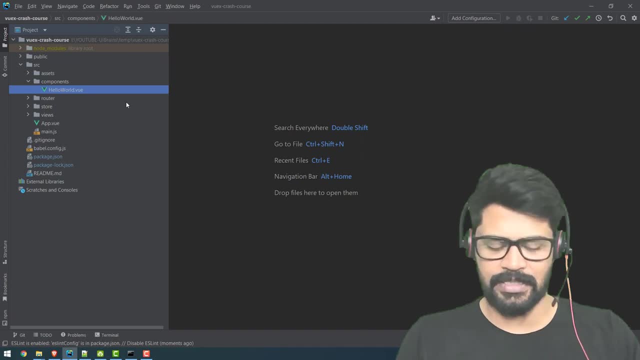 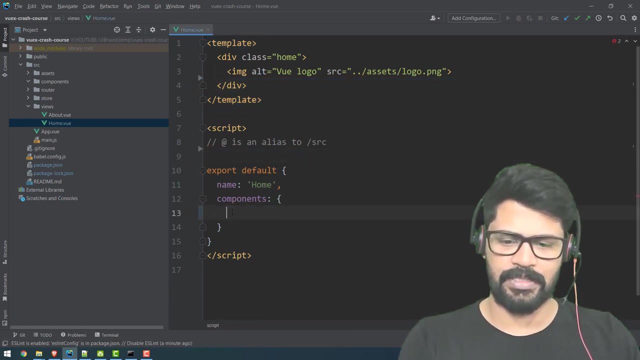 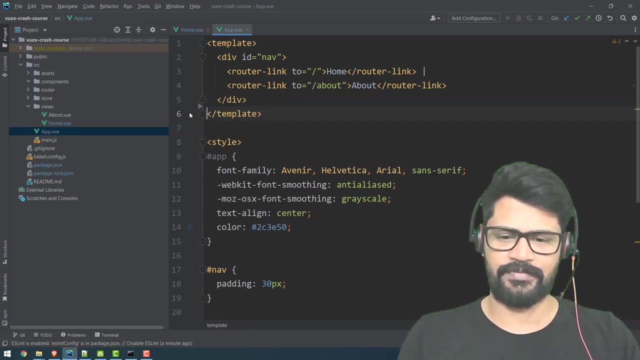 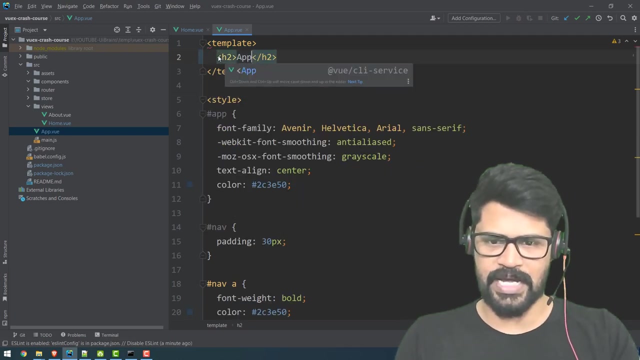 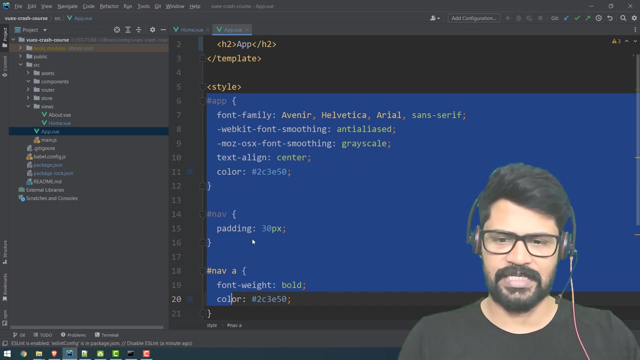 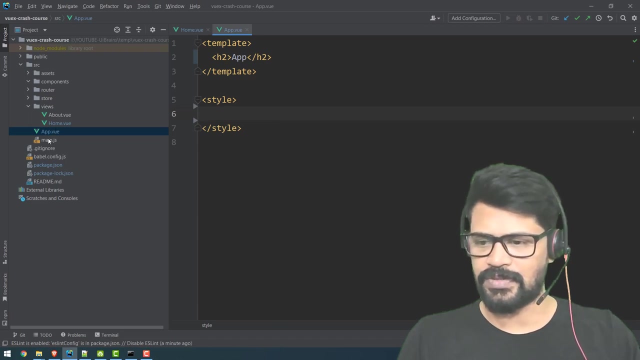 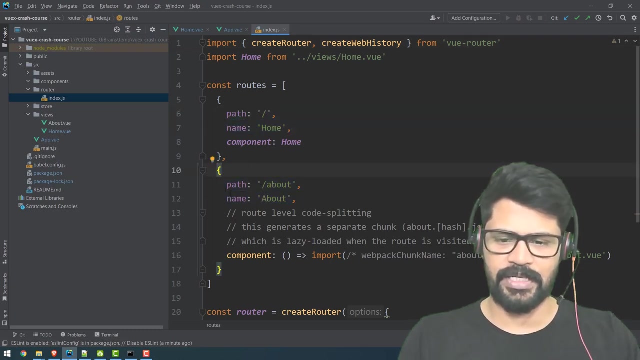 and i go to components i don't need the hello world view and this hello world view was there in the views of home page so i'll remove this hello world and i don't need the import i don't need the components yeah it's fine yeah and i don't need this routing as well so i go to add dot view i can remove this router view and there is nothing let's say h2 app component that's fine this app okay and i don't need any of these styles i can delete those styles okay yep that's fine and uh let's go to routing if i go to router folder index.js so i have a home page and about page actually i don't need 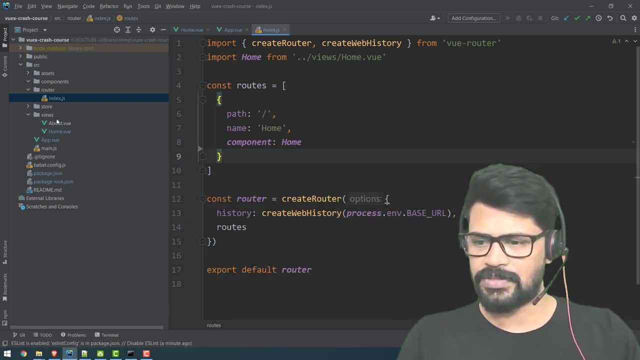 about page i can delete so i about that view is actually not required 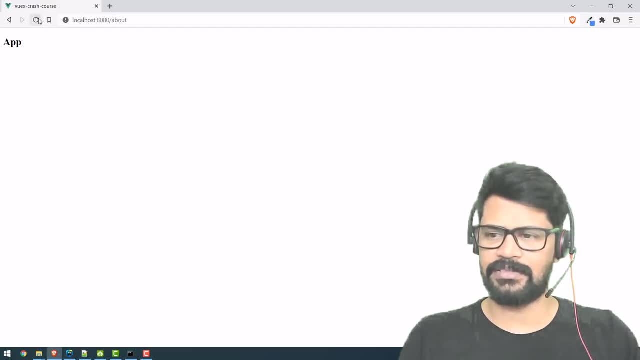 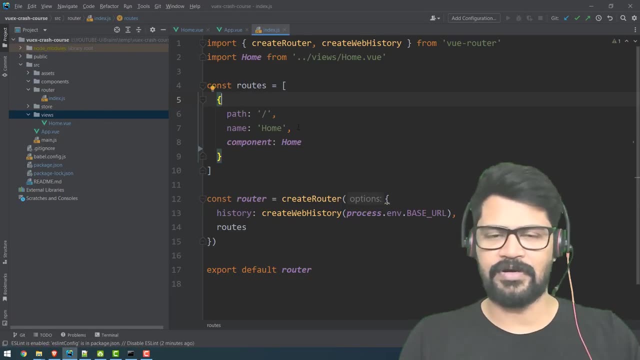 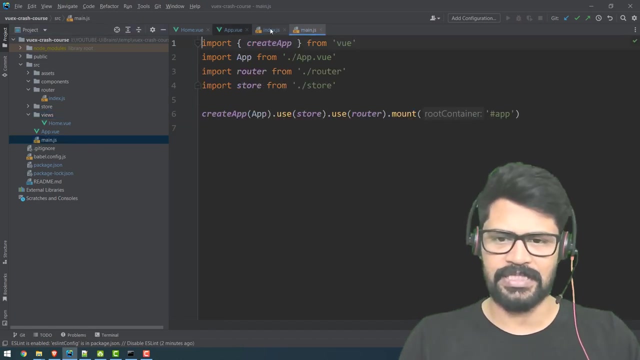 okay so i think that's fine yep yeah first uh one one last thing is we have not configured bootstrap yet for this application so to configure bootstrap you go inside main.js yeah here i'll import um 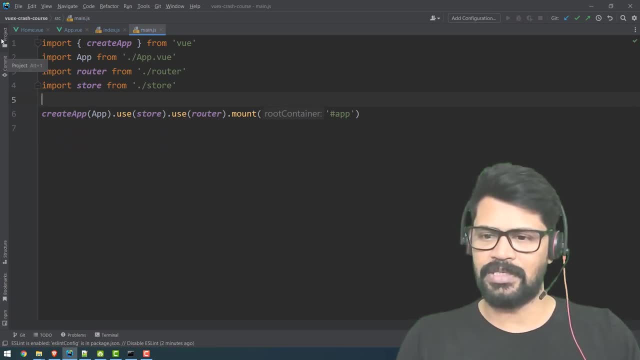 you may import in main.js or else you can 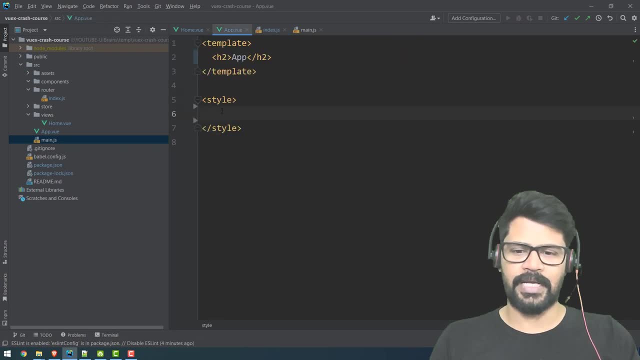 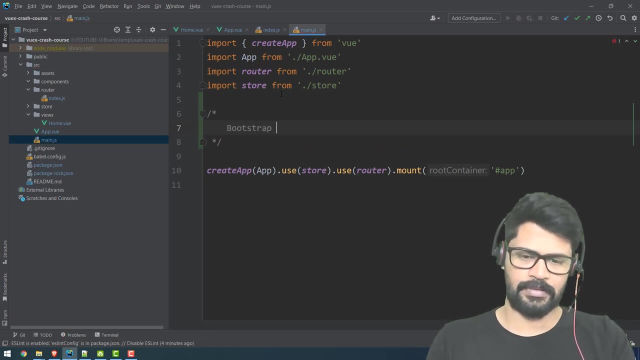 configure all right so in app dot uh no just go to main.js just add a bootstrap bootstrap styles so let's say import uh something dot slash node underscore module slash bootstrap 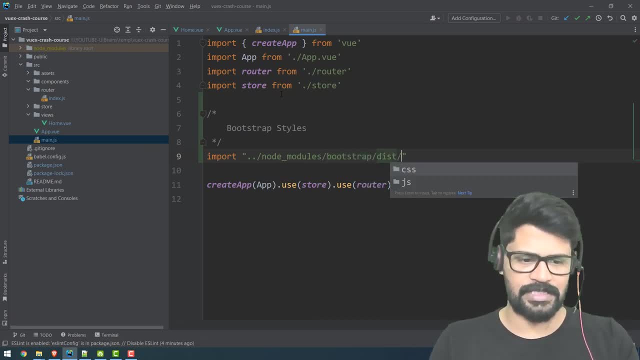 slash this slash css both sam.css and also i need import order slash node underscore modules slash bootstrap slash this and j s and uh i need uh bootstrap 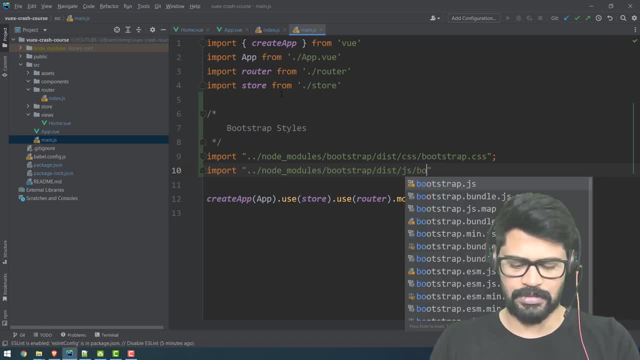 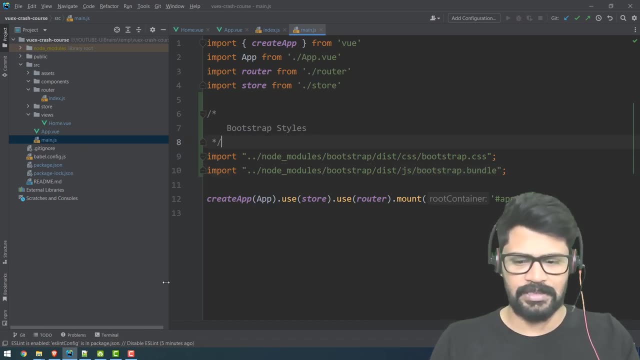 bootstrap bundle.js okay so these two we have to configure I'm not using any font awesome icons here I hope that's fine and let's check see it been 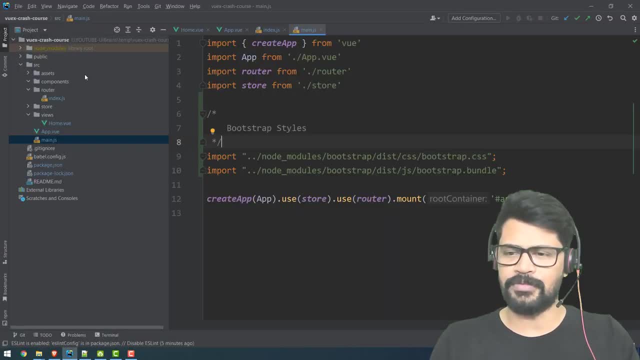 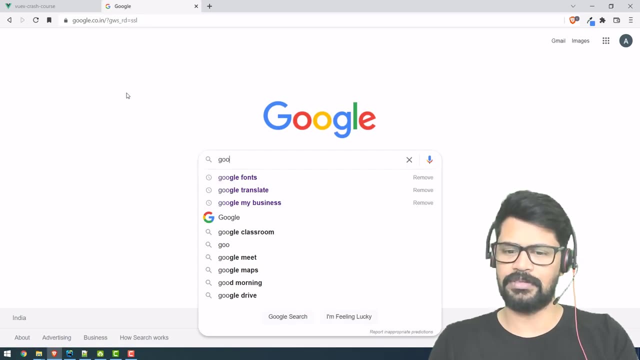 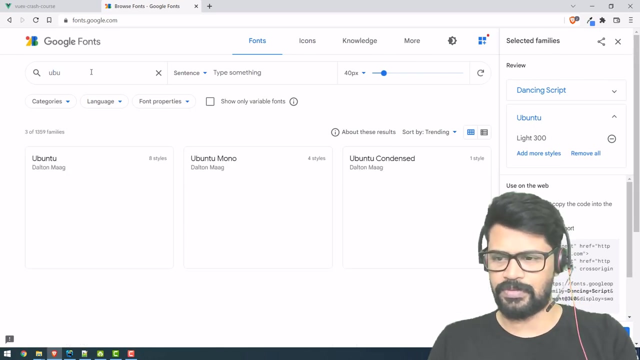 already configured with bootstrap and if you want to have any Google font you can search for Google fonts yeah I can select the regular one is Ubuntu font 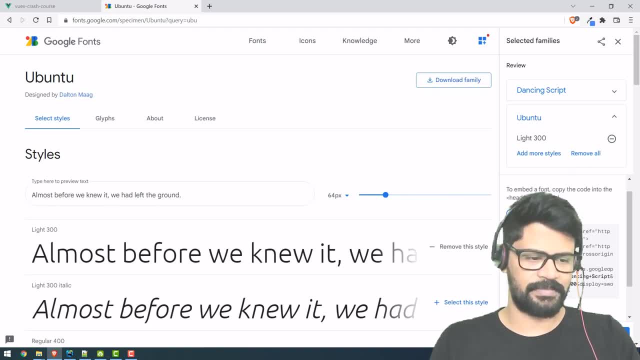 yet this one and let me copy the import statement yes yeah so where do I do was I 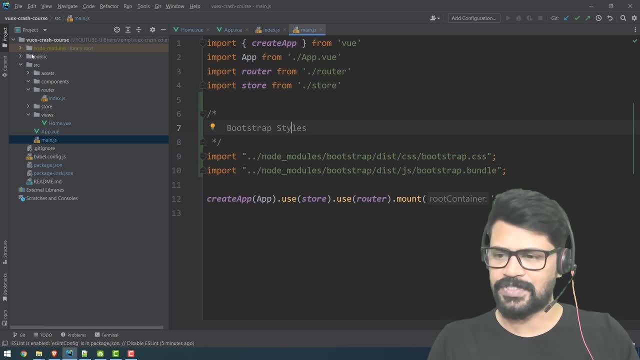 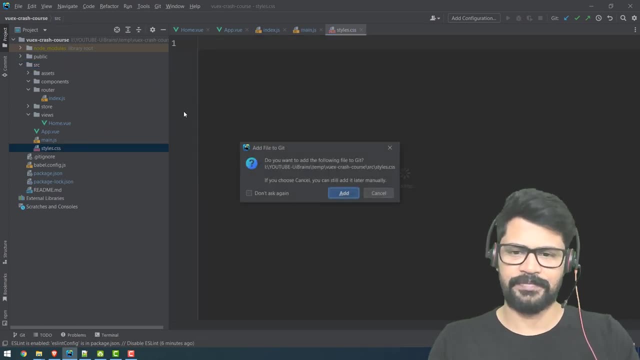 don't have any Excel style sheet so I'll create in SRC I create new style sheet that is style dot CSS this will become your Excel file. 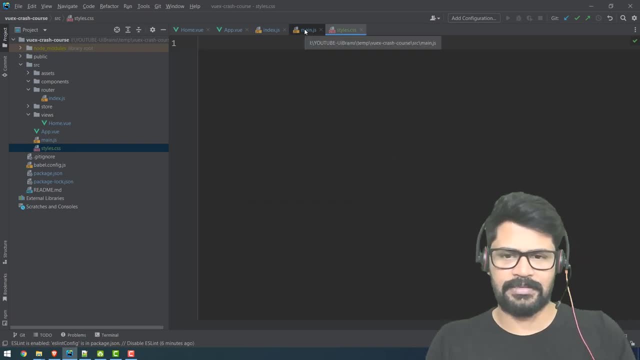 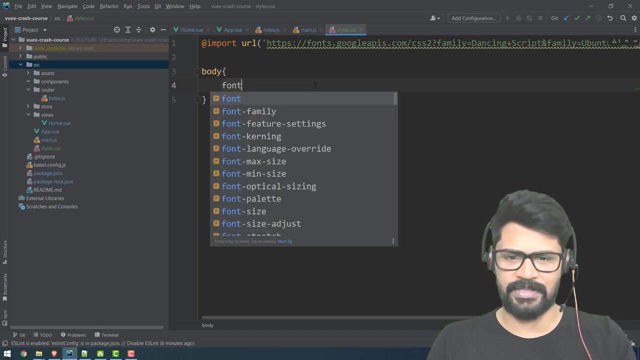 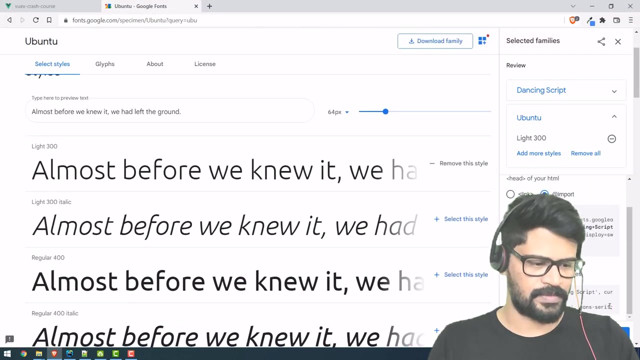 style sheet and let me connect to app dot view so it import from import style dot CSS and in style dot CSS I'll add my font awesome import statement and also for the body tag font family is Ubuntu right this one okay all right so font 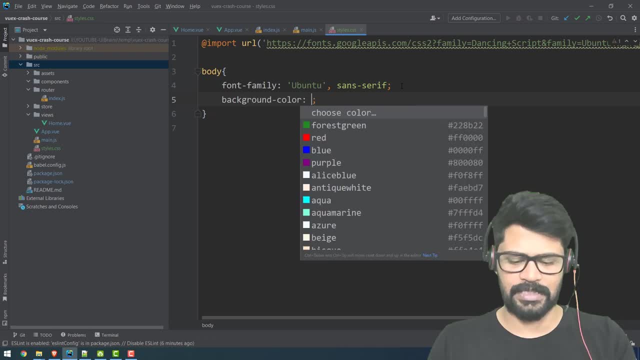 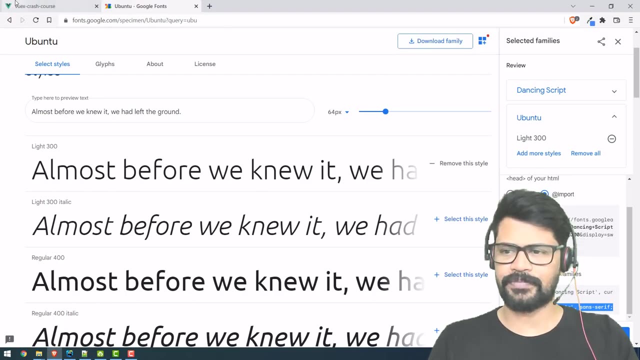 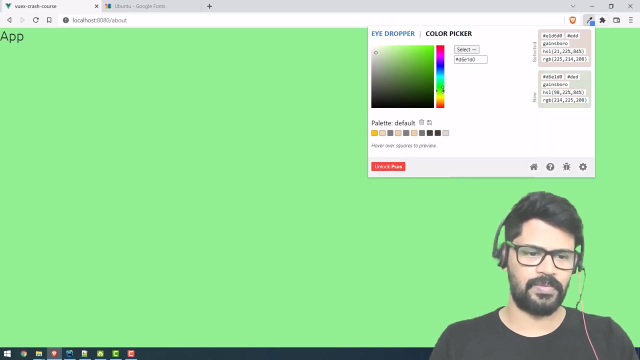 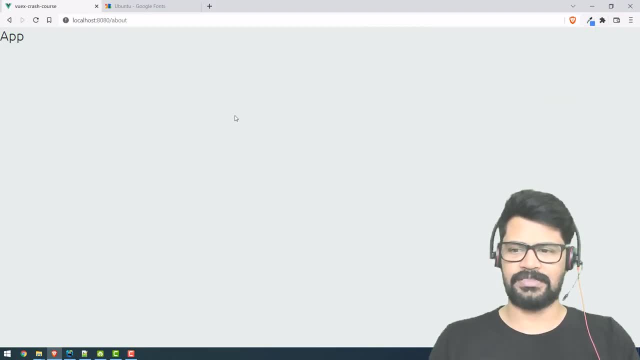 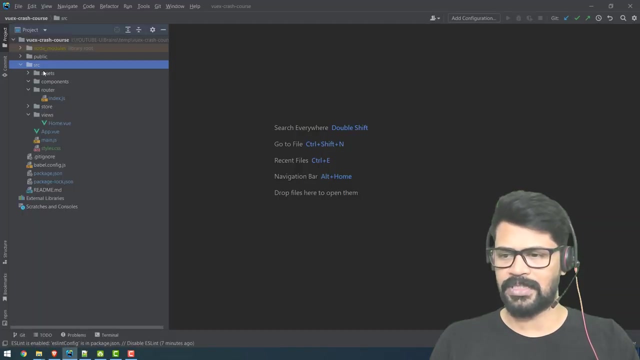 light color I think even lightest okay light color I think even lightest okay okay the slight color that's fine yep so okay the slight color that's fine yep so okay the slight color that's fine yep so this setup is already so we are done this setup is already so we are done this setup is already so we are done with bootstrap and font us I mean with bootstrap and font us I mean with bootstrap and font us I mean the font configuration and then let's the font configuration and then let's the font configuration and then let's create all the views and components so I create all the views and components so I create all the views and components so I will create components so I create first will create components so I create first will create components so I create first component for us is a view component 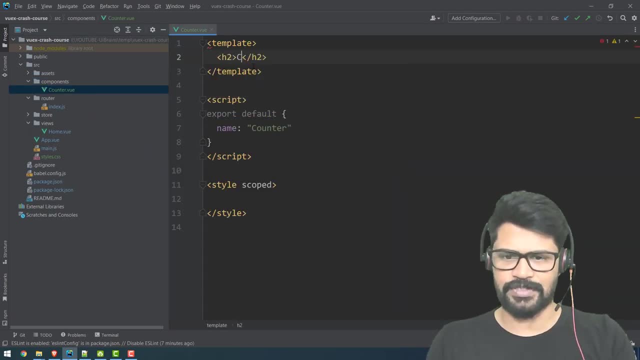 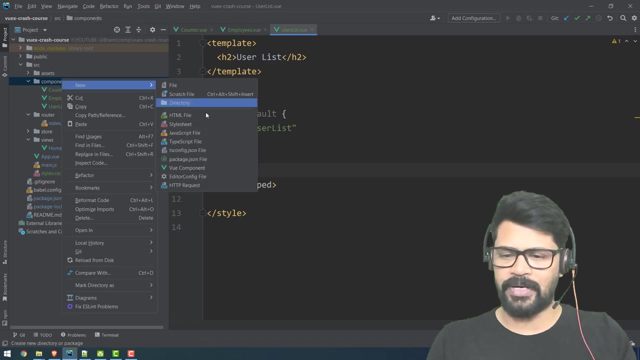 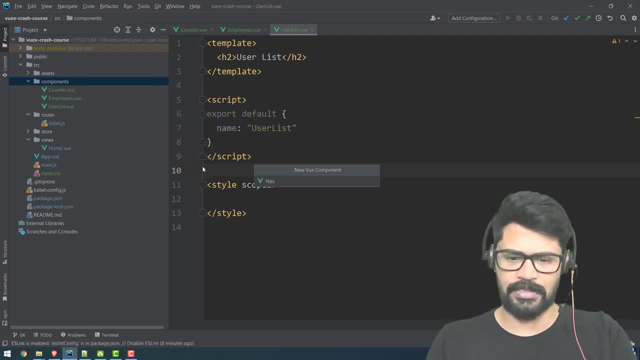 fine and also we need one more component fine and also we need one more component for navbar you can create for navbar okay 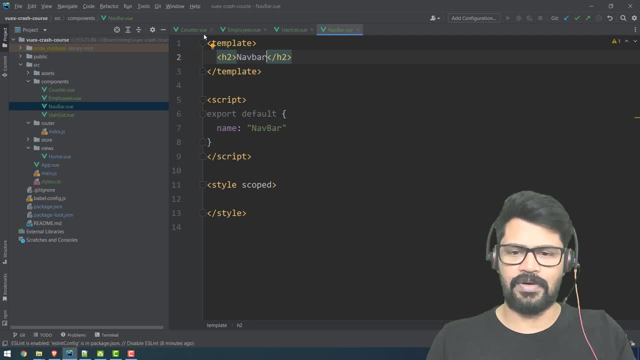 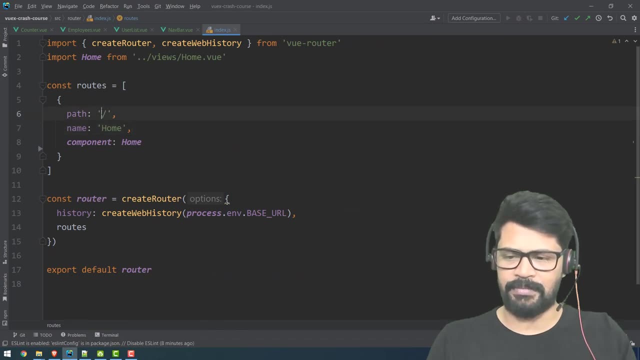 for navbar you can create for navbar okay for navbar you can create for navbar okay let's say h2 navbar okay so all let's say h2 navbar okay so all let's say h2 navbar okay so all these components let me connect with these components let me connect with these components let me connect with routing so you go to router index or J routing so you go to router index or J routing so you go to router index or J yes yeah here for empty path slash home yes yeah here for empty path slash home yes yeah here for empty path slash home is there and let's stay so let's take is there and let's stay so let's take 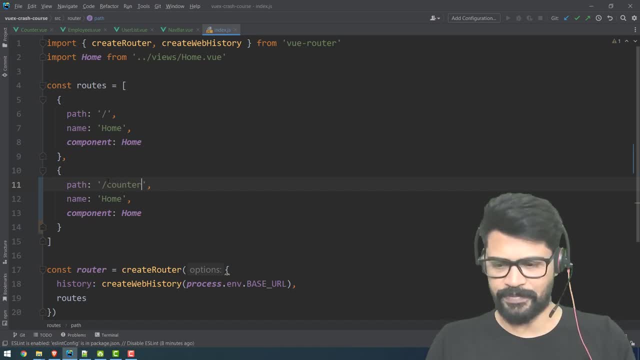 is there and let's stay so let's take here path slash counter okay so slash here path slash counter okay so slash 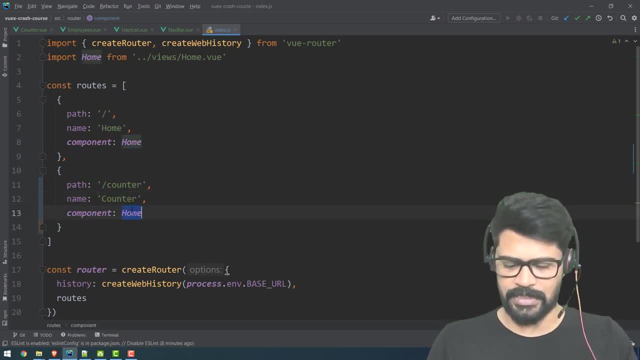 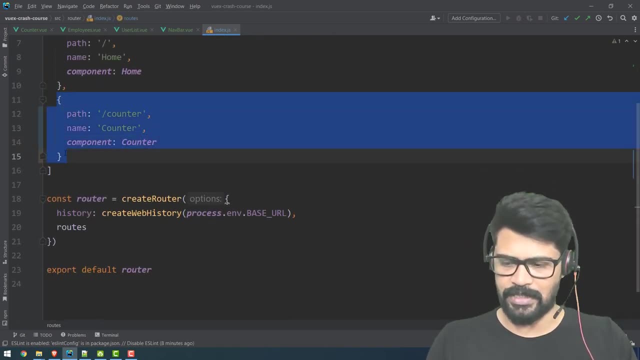 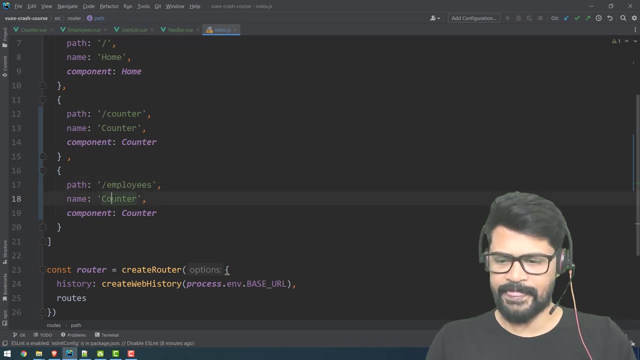 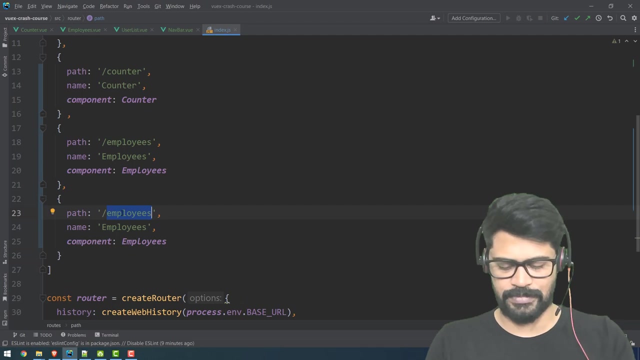 here path slash counter okay so slash counter I'll go to counter component and counter I'll go to counter component and counter I'll go to counter component and this will be the counter component it this will be the counter component it this will be the counter component it will import from our components folder will import from our components folder will import from our components folder and the same way I'll copy here and the same way I'll copy here and the same way I'll copy here this is employees this is employees and this is employees this is employees and this is employees this is employees and employees employees component and one employees employees component and one employees employees component and one last one is the users component this last one is the users component this last one is the users component this will be the user list 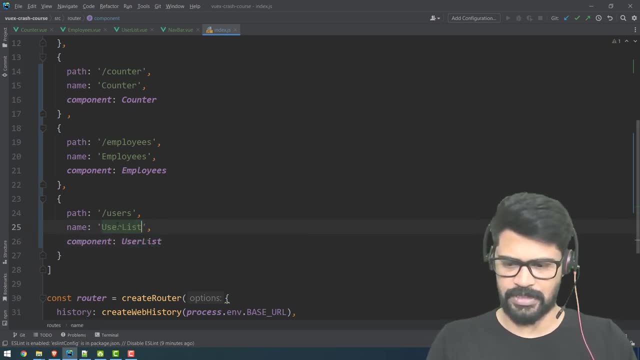 will be the user list will be the user list okay user list component okay so routing has 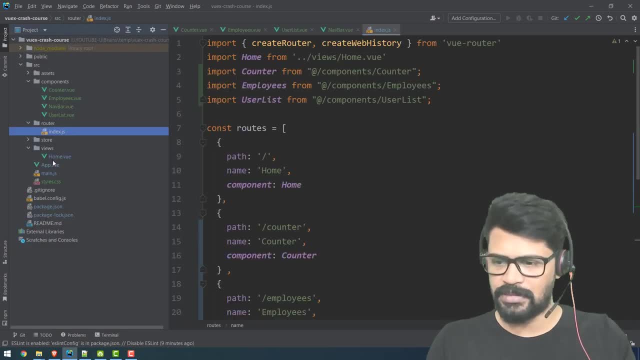 okay user list component okay so routing has okay user list component okay so routing has been done now go to app dot view in 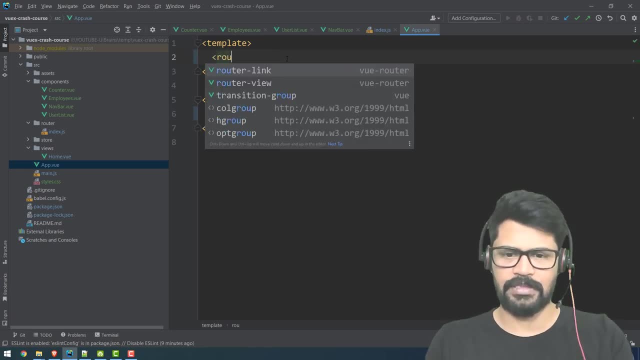 been done now go to app dot view in been done now go to app dot view in this I will configure a router view so 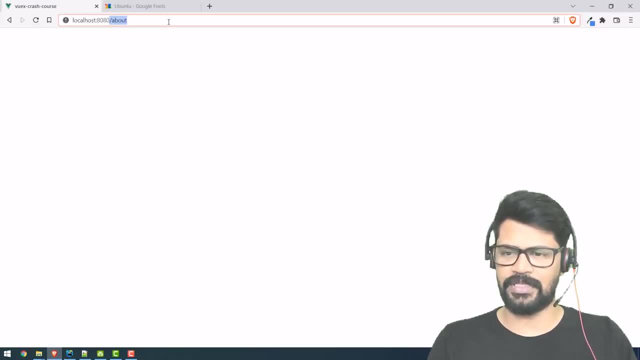 this I will configure a router view so this I will configure a router view so that all the routing configuration will that all the routing configuration will that all the routing configuration will come here okay just home page and I just 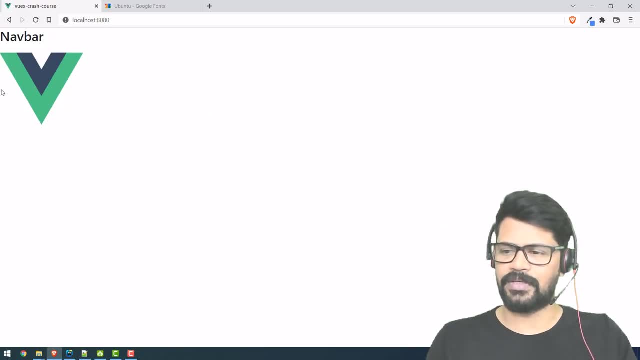 come here okay just home page and I just come here okay just home page and I just need also navbar okay navbar and home 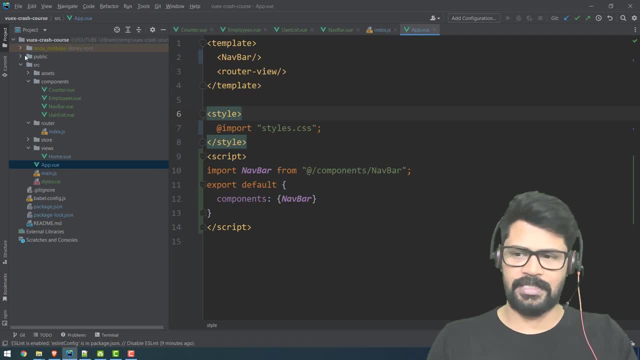 need also navbar okay navbar and home need also navbar okay navbar and home page okay fine and a small configuration 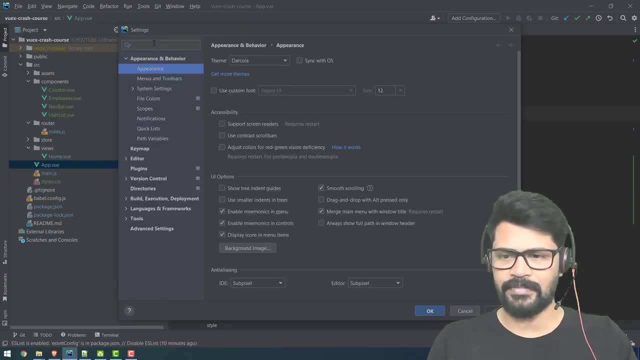 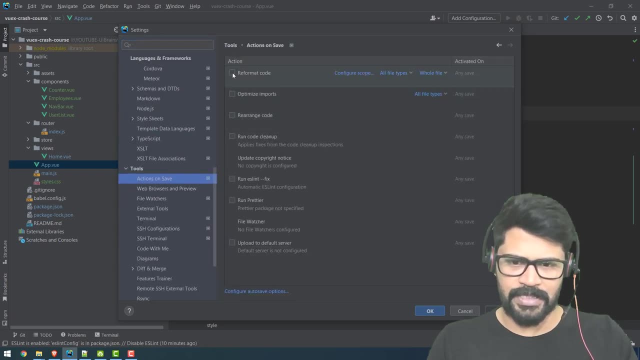 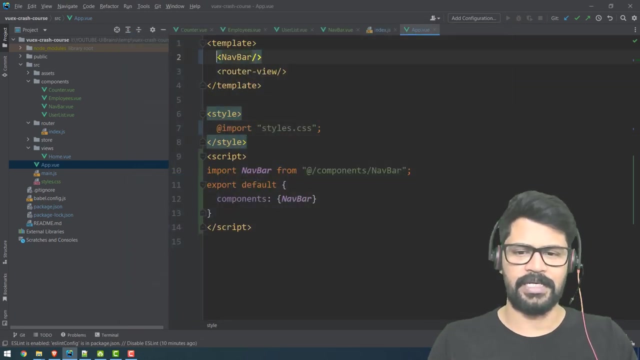 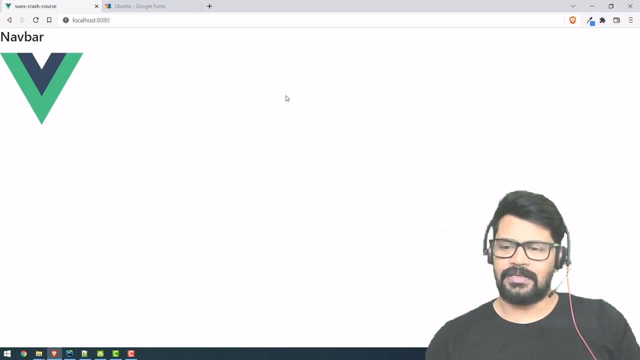 page okay fine and a small configuration I wanna do is for prettier pretty every I wanna do is for prettier pretty every I wanna do is for prettier pretty every format optimize arrange code yep apply format optimize arrange code yep apply format optimize arrange code yep apply because it will format the code if because it will format the code if because it will format the code if something here and there like something something here and there like something something here and there like something here you made it you save it will come here you made it you save it will come here you made it you save it will come in a proper location okay this will in a proper location okay this will in a proper location okay this will formatting the code okay formatting the code okay okay formatting the code okay okay that's fine and let's jump in for the that's fine and let's jump in for the 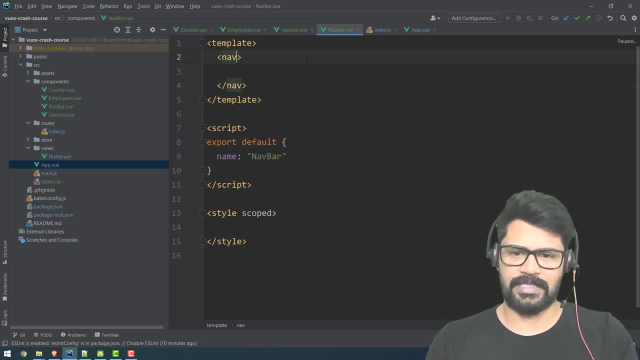 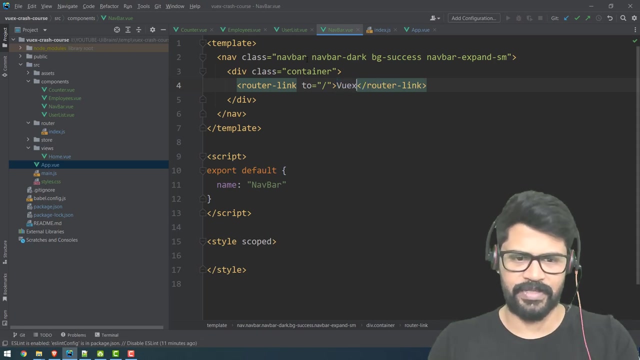 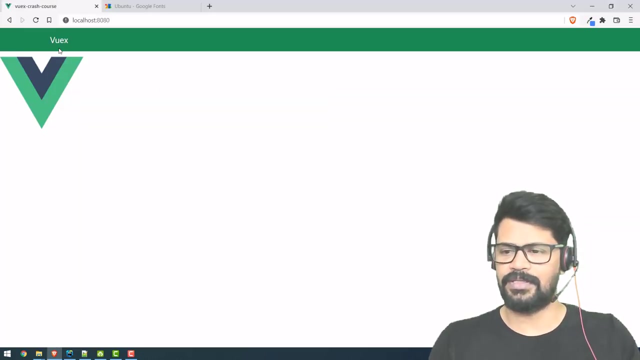 that's fine and let's jump in for the number quickly so now tag with the class number quickly so now tag with the class number quickly so now tag with the class now bar now bar dark and now now bar no now bar now bar dark and now now bar no now bar now bar dark and now now bar no no no BG success and now bar expand SM no no BG success and now bar expand SM no no BG success and now bar expand SM in that one container one router link in that one container one router link in that one container one router link slash for the home and let's say this is slash for the home and let's say this is slash for the home and let's say this is view X okay that's fine and give the view X okay that's fine and give the view X okay that's fine and give the class called now bar brand okay you get class called now bar brand okay you get 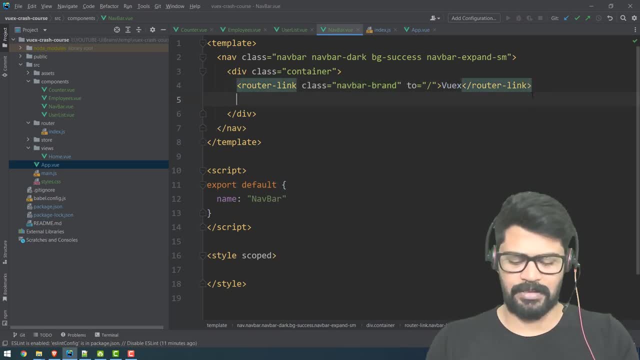 class called now bar brand okay you get the VX and also under that one collapse the VX and also under that one collapse 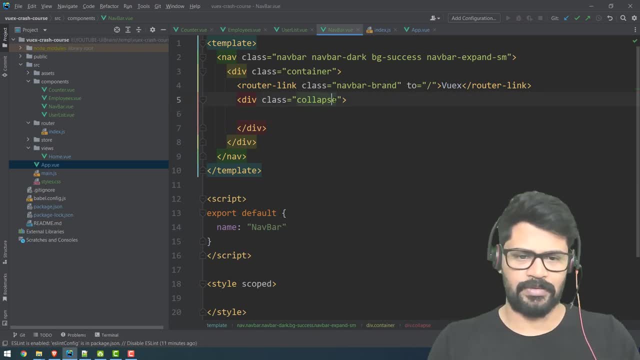 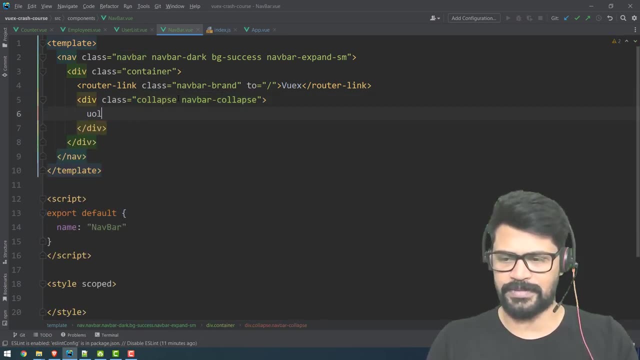 the VX and also under that one collapse and one more class is let me expand now and one more class is let me expand now and one more class is let me expand now about collapse one you well sorry you about collapse one you well sorry you about collapse one you well sorry you well a lie well a lie 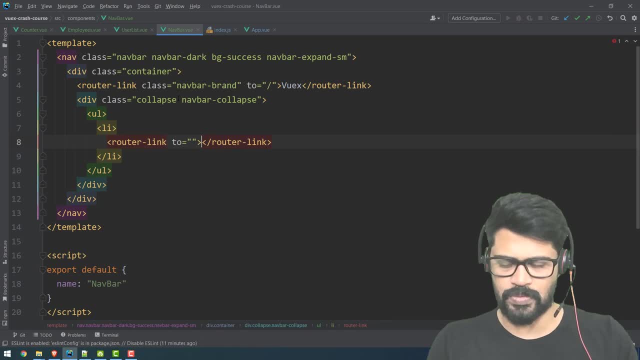 well a lie router link to something here is counter router link to something here is counter router link to something here is counter this will be slash counter let me give this will be slash counter let me give 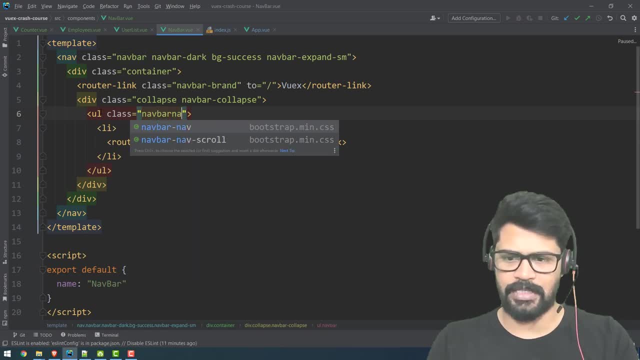 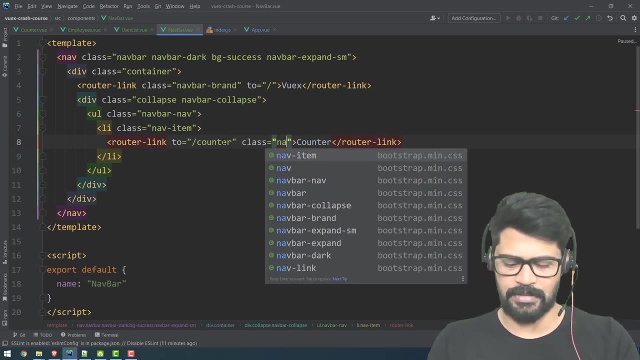 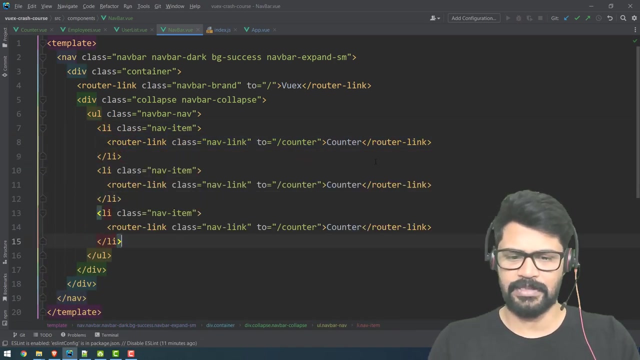 this will be slash counter let me give the class now bar now now item here is the class now bar now now item here is the class now bar now now item here is now link okay so I got one let's copy 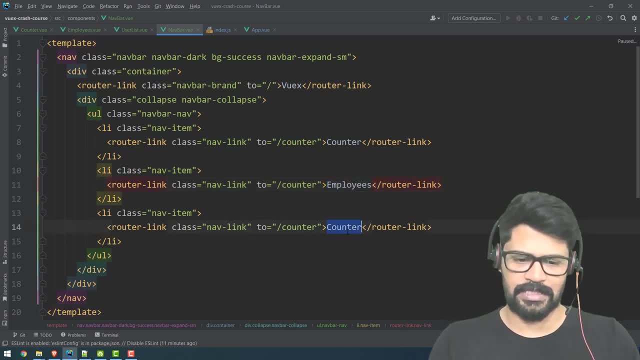 now link okay so I got one let's copy now link okay so I got one let's copy so this is employees and this is user list so this is employees and this is user list so this is employees and this is user list sorry sorry user list so but this is sorry sorry user list so but this is sorry sorry user list so but this is employees and this is users okay is that employees and this is users okay is that 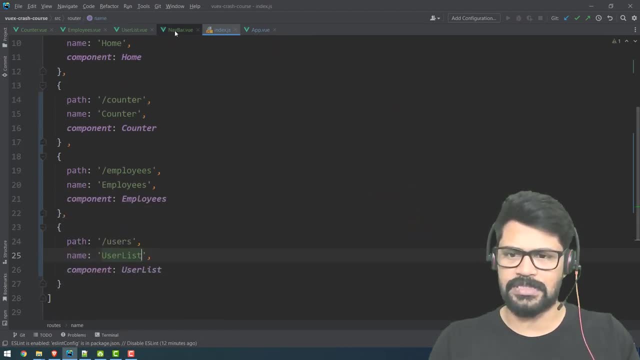 employees and this is users okay is that users counter employees and users okay users counter employees and users okay users counter employees and users okay whites all right yeah that's fine and whites all right yeah that's fine and 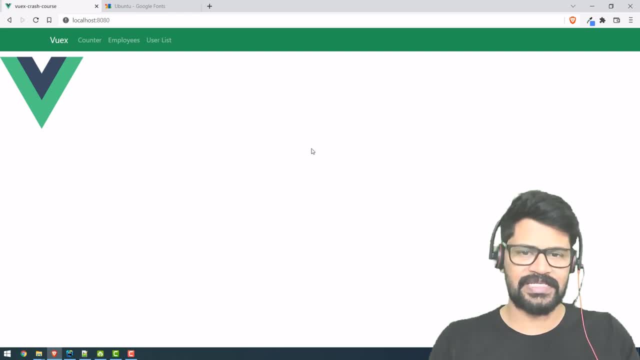 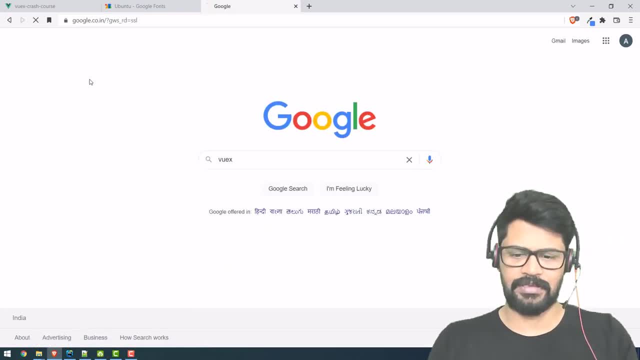 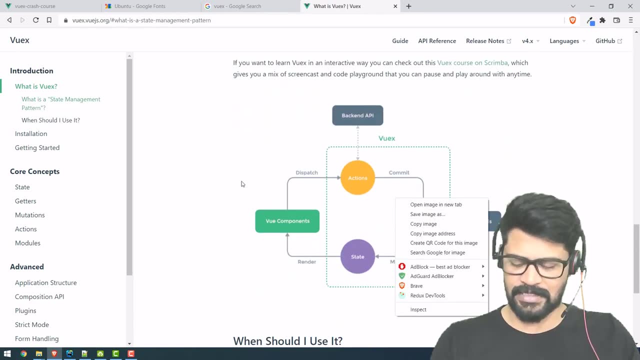 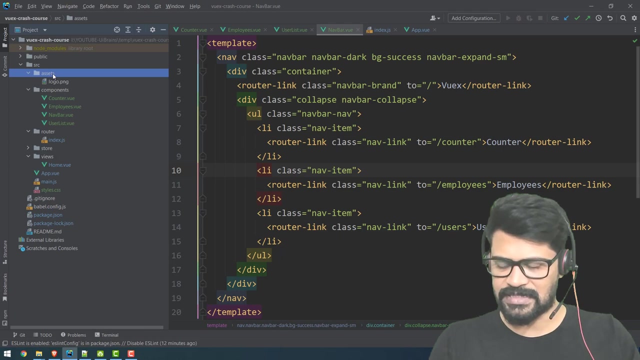 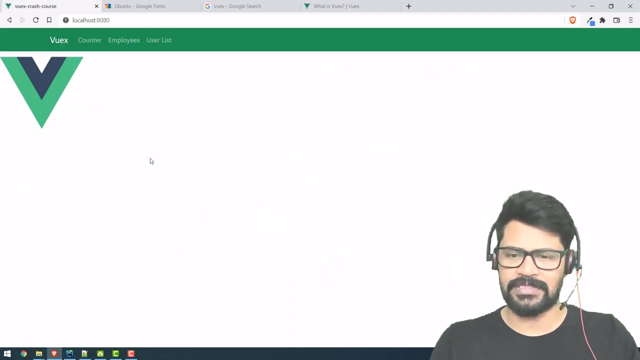 this image from the official this image from the official website you can search for a Google Vue X the website you can search for a Google Vue X the website you can search for a Google Vue X the Vue X dot Vue J dot o R G and here I Vue X dot Vue J dot o R G and here I Vue X dot Vue J dot o R G and here I got this image I can save image as so I got this image I can save image as so I got this image I can save image as so I got that image here on my desktop and so got that image here on my desktop and so got that image here on my desktop and so what I do is I go to assets and I'll what I do is I go to assets and I'll what I do is I go to assets and I'll paste a Vue X and where does this image paste a Vue X and where does this image paste a Vue X and where does this image is coming from this is the home page is coming from this is the home page 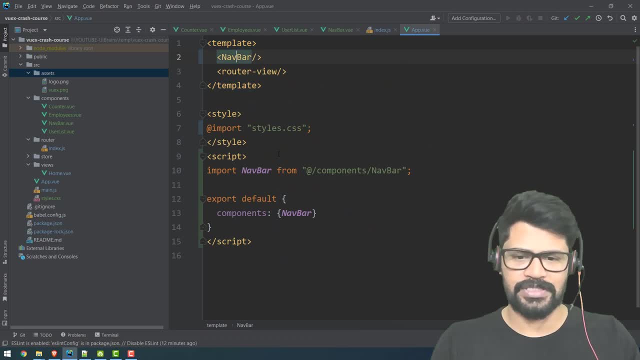 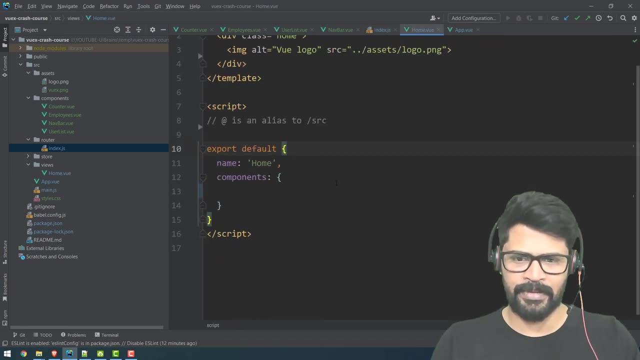 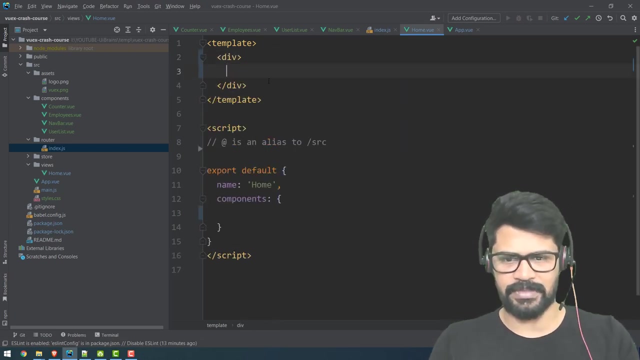 is coming from this is the home page right for empty slash so let me go to a right for empty slash so let me go to a right for empty slash so let me go to a home page in the router router index or home page in the router router index or home page in the router router index or J is go to home page in this I don't J is go to home page in this I don't J is go to home page in this I don't need a division class home and all more need a division class home and all more need a division class home and all more required just simple division one image required just simple division one image required just simple division one image SRC is assets slash Vue X dot PNG you SRC is assets slash Vue X dot PNG you SRC is assets slash Vue X dot PNG you get the image and let's keep it Center get the image and let's keep it Center get the image and let's keep it Center this can just write to the class called this can just write to the class called this can just write to the class called text center okay that's all and you want 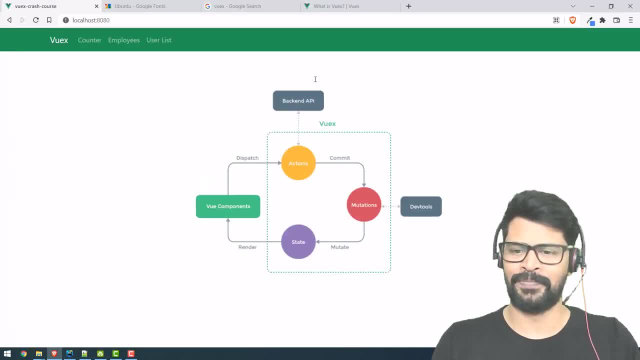 text center okay that's all and you want text center okay that's all and you want to have some margin the same margin of to have some margin the same margin of to have some margin the same margin of files comes in Center okay that's all is files comes in Center okay that's all is files comes in Center okay that's all is your home page just one simple image your home page just one simple image 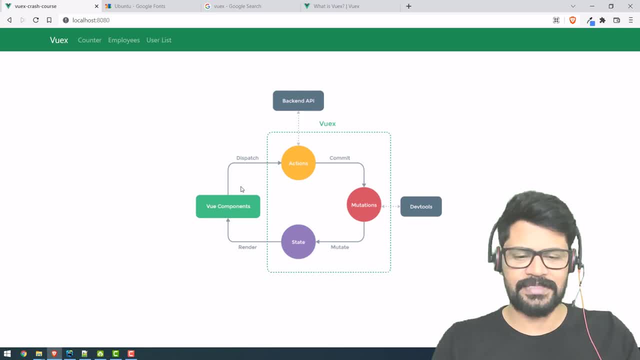 your home page just one simple image which contains the flow and all which which contains the flow and all which which contains the flow and all which helps a lot for creating this view X helps a lot for creating this view X helps a lot for creating this view X application okay the flow and all that's application okay the flow and all that's 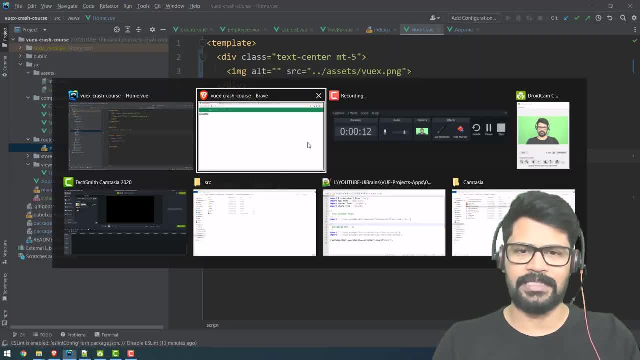 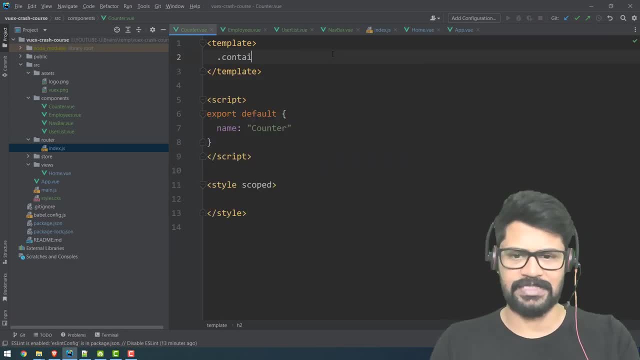 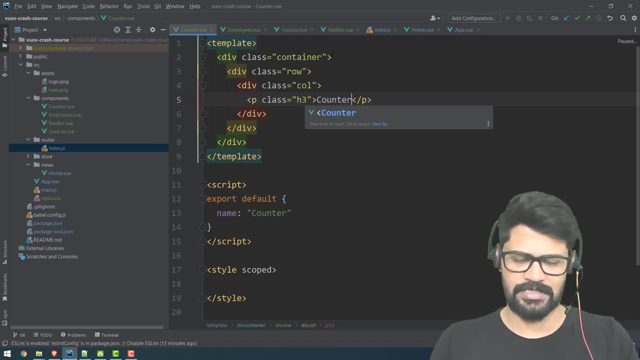 application okay the flow and all that's fine and now let's jump into the fine and now let's jump into the fine and now let's jump into the counter okay and let's make the counter counter okay and let's make the counter counter okay and let's make the counter with local setup so go to counter let's with local setup so go to counter let's with local setup so go to counter let's make some default setup container one make some default setup container one make some default setup container one row single column P dot h3 counter okay so row single column P dot h3 counter okay so row single column P dot h3 counter okay so let's say something called text success let's say something called text success let's say something called text success okay so let's make some margin top three okay so let's make some margin top three okay so let's make some margin top three and one paragraph there's some lorem 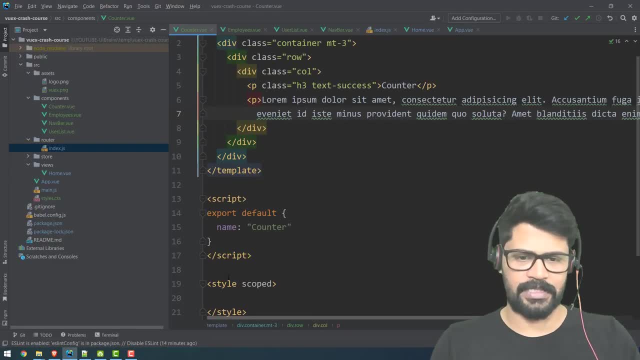 and one paragraph there's some lorem and one paragraph there's some lorem 30 times this introduction content and you 30 times this introduction content and you 30 times this introduction content and you can just be the class called font font can just be the class called font font can just be the class called font font style italic okay so let's make a style italic okay so let's make a style italic okay so let's make a counter with the card and increments so counter with the card and increments so counter with the card and increments so okay let's keep this content as it is okay let's keep this content as it is okay let's keep this content as it is let's start with another container one 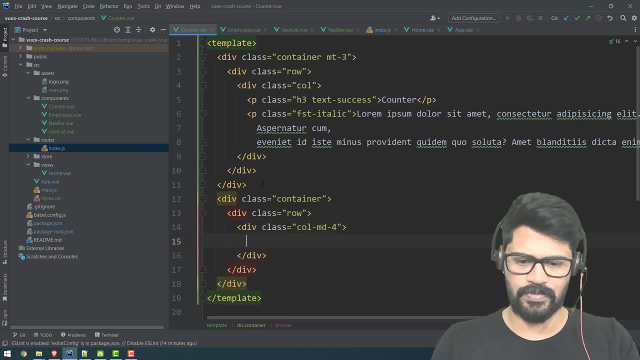 let's start with another container one let's start with another container one row call MD for one card card body so 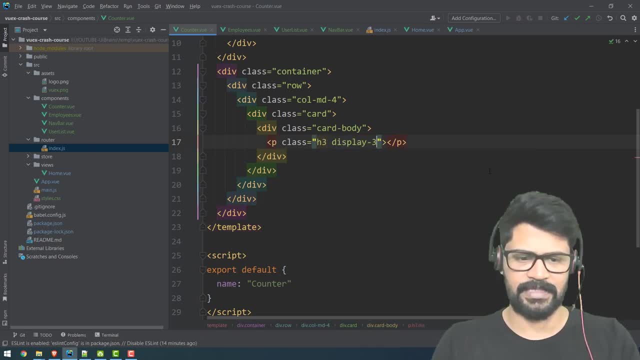 row call MD for one card card body so I'll say here P dot h3 with some I'll say here P dot h3 with some I'll say here P dot h3 with some display 3 some 9 number okay so fuck a display 3 some 9 number okay so fuck a 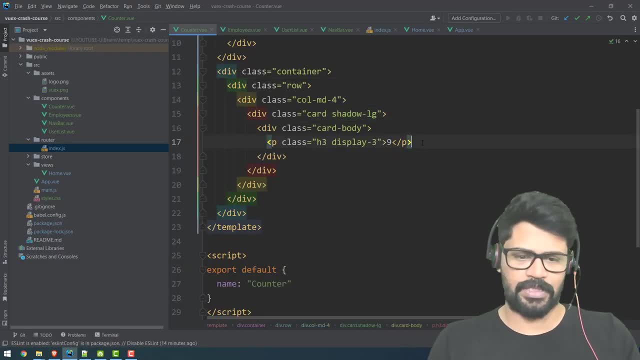 display 3 some 9 number okay so fuck a card you just say some shadow okay under card you just say some shadow okay under card you just say some shadow okay under that I'll have a button with the class that I'll have a button with the class 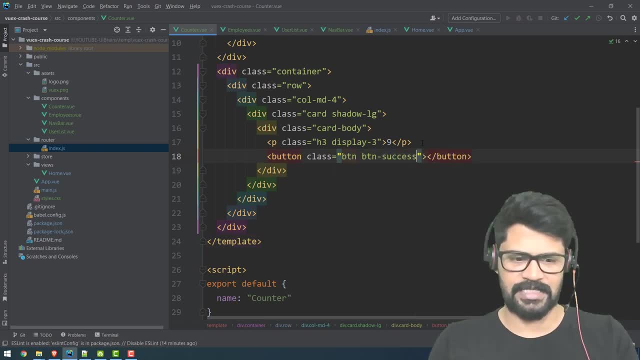 that I'll have a button with the class BT n BT n minus success BT n BT n minus success BT n BT n BT n minus success and yep this is in increments okay and and yep this is in increments okay and 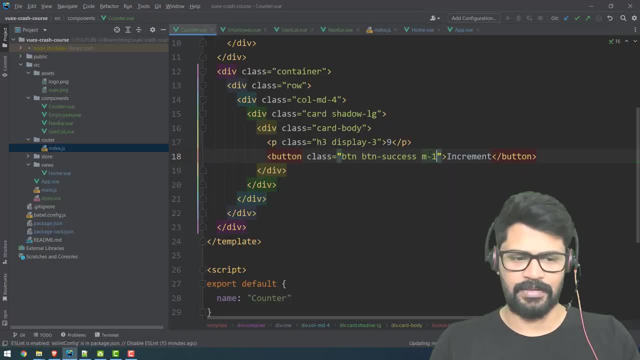 and yep this is in increments okay and let's add some margin okay let's have let's add some margin okay let's have let's add some margin okay let's have few other buttons let's say BT and hyphen few other buttons let's say BT and hyphen few other buttons let's say BT and hyphen warning and this is medium hyphen 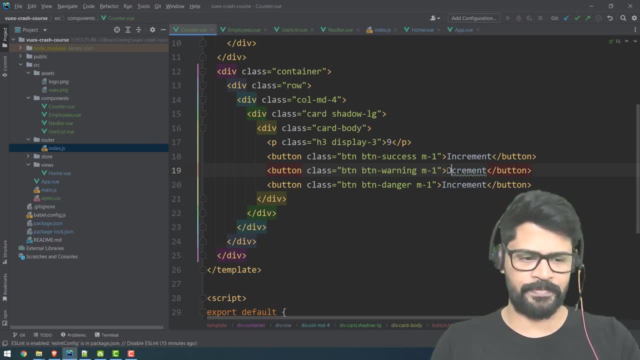 warning and this is medium hyphen warning and this is medium hyphen danger this will be a decrement button danger this will be a decrement button danger this will be a decrement button and this is just increment by okay fine and this is just increment by okay fine and this is just increment by okay fine so I got structure ready so I'll 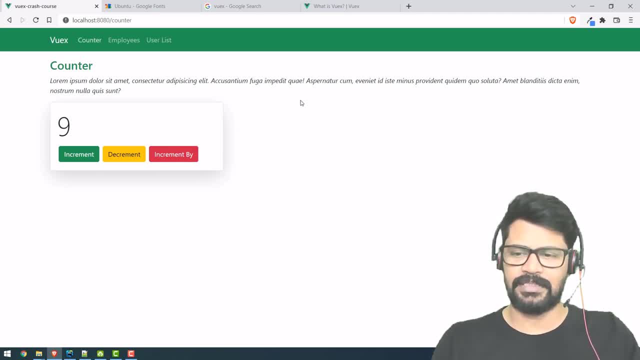 so I got structure ready so I'll so I got structure ready so I'll now now now now let's make this component from I mean 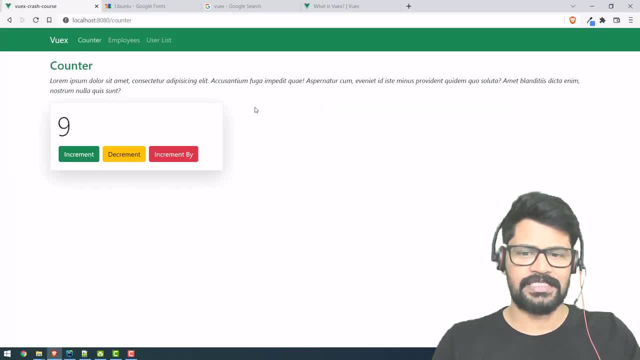 let's make this component from I mean let's make this component from I mean without UX okay local state management 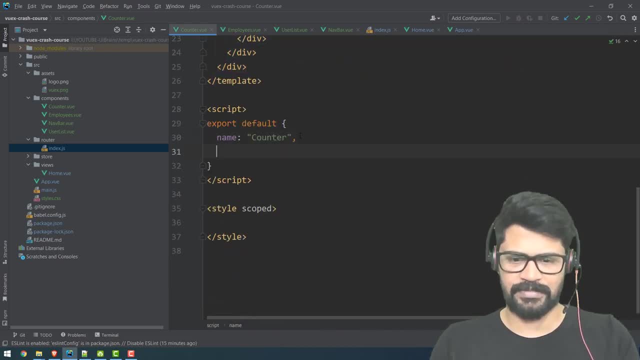 without UX okay local state management so for local state what you do is here so for local state what you do is here so for local state what you do is here data data is actually a function so that data data is actually a function so that data data is actually a function so that function returns an object so that function returns an object so that function returns an object so that contains the count value of type 0 okay contains the count value of type 0 okay contains the count value of type 0 okay and then you have methods what type of and then you have methods what type of and then you have methods what type of methods you have is three methods for methods you have is three methods for methods you have is three methods for increment decrement increment decrement and increment by so increment okay to say click click and increment by so increment okay to say click click 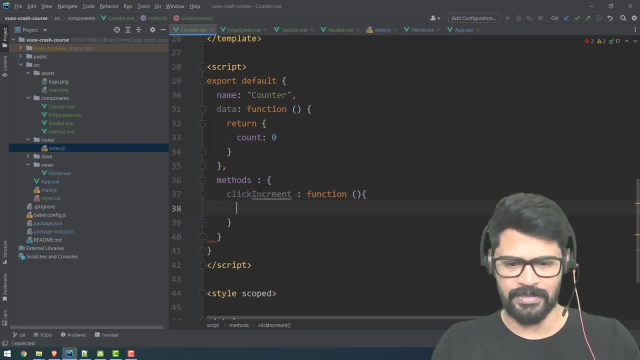 and increment by so increment okay to say click click increment is one function okay increment is one function okay increment is one function okay click increment is one function so what it click increment is one function so what it click increment is one function so what it does is it just update your counter does is it just update your counter does is it just update your counter okay so this dot count is equal to this okay so this dot count is equal to this okay so this dot count is equal to this dot count plus one that's it and let's dot count plus one that's it and let's dot count plus one that's it and let's take one take one take one more method click decrement let's make it more method click decrement let's make it more method click decrement let's make it as minus one and let's make one more 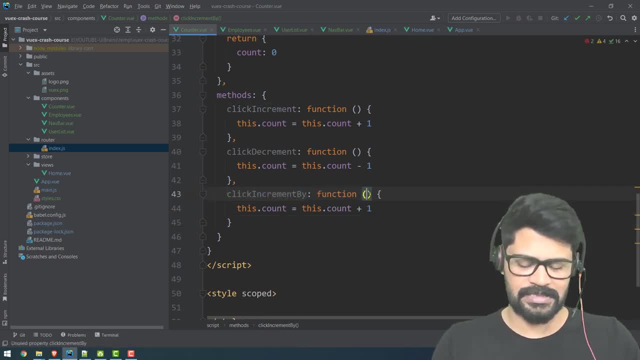 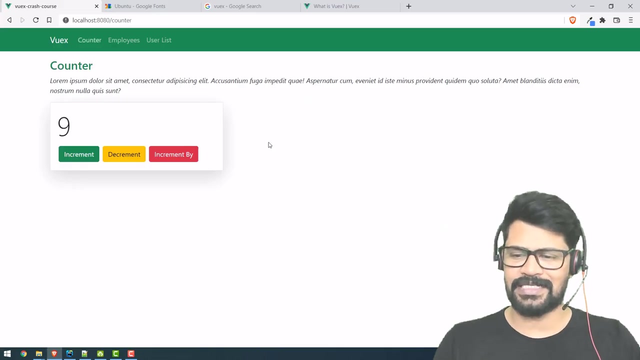 as minus one and let's make one more as minus one and let's make one more click increment by is a function so what click increment by is a function so what click increment by is a function so what it does is it takes a value what is that it does is it takes a value what is that it does is it takes a value what is that you're gonna update and just take it as you're gonna update and just take it as you're gonna update and just take it as value okay increment decrement and value okay increment decrement and value okay increment decrement and increment by is as a value okay so I increment by is as a value okay so I increment by is as a value okay so I have three functions and the state now have three functions and the state now have three functions and the state now let's come let's connect this state data let's come let's connect this state data 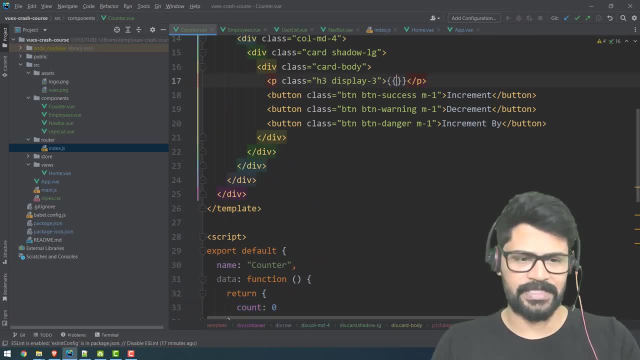 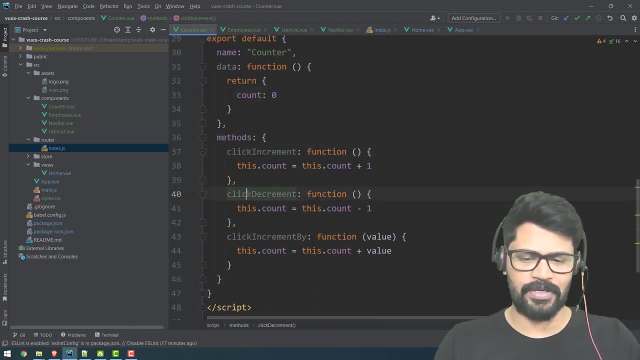 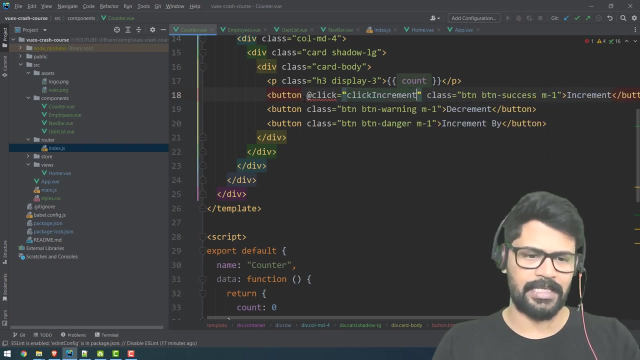 let's come let's connect this state data here so you can use the view expression here so you can use the view expression here so you can use the view expression just say count you get account become just say count you get account become just say count you get account become zero because it was zero and a click zero because it was zero and a click zero because it was zero and a click event happens I have to call these event happens I have to call these event happens I have to call these functions okay so let's say at click functions okay so let's say at click functions okay so let's say at click happens is equal to click increment as a happens is equal to click increment as a happens is equal to click increment as a function so simply it just increments it function so simply it just increments it function so simply it just increments it that's fine and it's also a copy of it 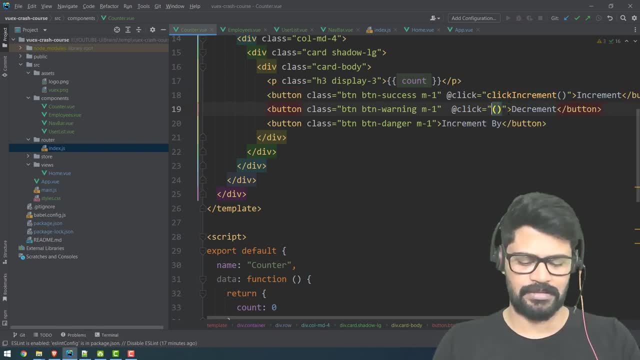 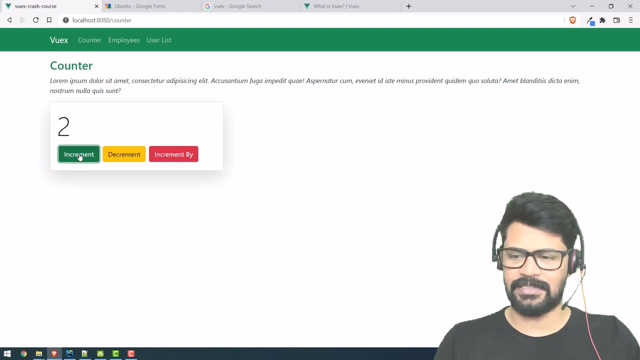 that's fine and it's also a copy of it that's fine and it's also a copy of it so let's make this is for click so let's make this is for click so let's make this is for click decrement and the one so click decrement and the one so click decrement and the one so click increment by you have to provide a value increment by you have to provide a value increment by you have to provide a value of the same height okay so now how this of the same height okay so now how this of the same height okay so now how this works is let's see increment is working works is let's see increment is working works is let's see increment is working perfect increment by is incrementing by perfect increment by is incrementing by perfect increment by is incrementing by Phi okay so that's fine cool so this is Phi okay so that's fine cool so this is 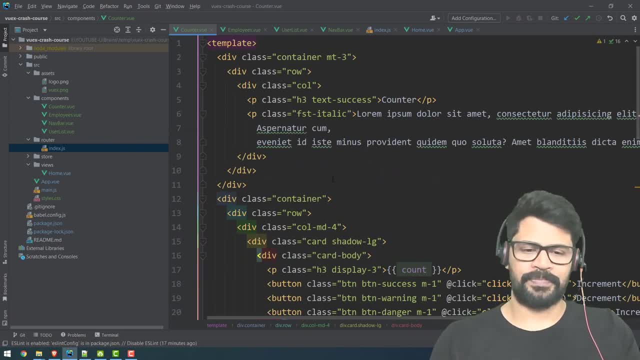 Phi okay so that's fine cool so this is done right so this is just a local local done right so this is just a local local 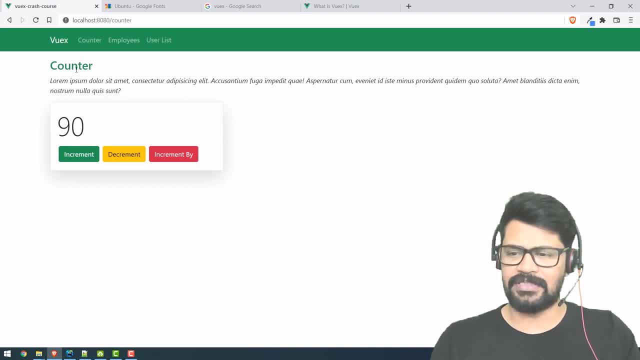 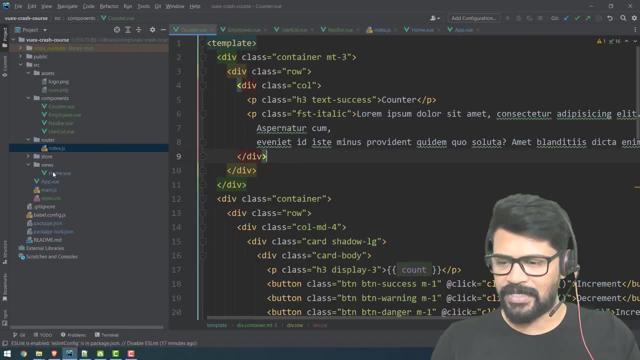 done right so this is just a local local state management now let's convert this state management now let's convert this state management now let's convert this whole setup to view X okay so how to whole setup to view X okay so how to whole setup to view X okay so how to make a view etc you know don't worry we make a view etc you know don't worry we make a view etc you know don't worry we already have view X here if you go to 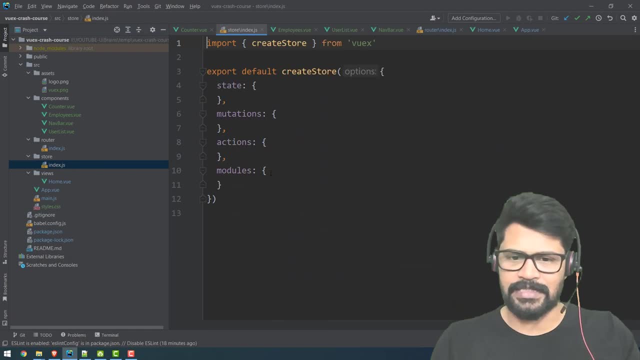 already have view X here if you go to already have view X here if you go to storage storage storage so there's a folder called store in that so there's a folder called store in that so there's a folder called store in that index.js yeah this is actually your view index.js yeah this is actually your view index.js yeah this is actually your view X configuration so create store which X configuration so create store which 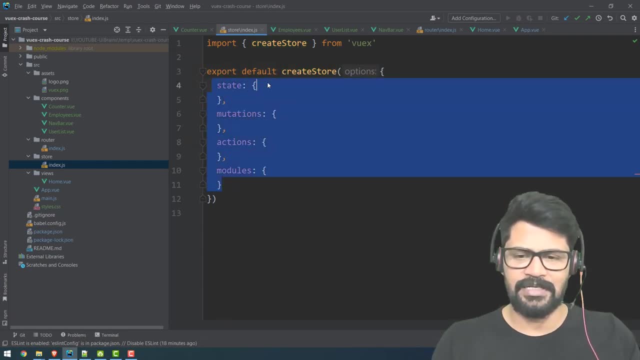 X configuration so create store which contains state mutations actions and contains state mutations actions and contains state mutations actions and modules and this store has configured to modules and this store has configured to 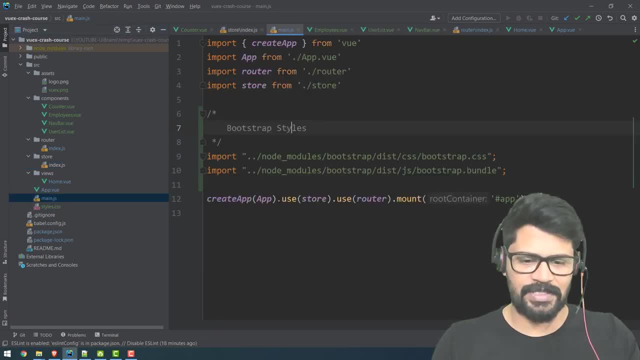 modules and this store has configured to the application in main dot J is is here the application in main dot J is is here the application in main dot J is is here you store okay so with this store is you store okay so with this store is 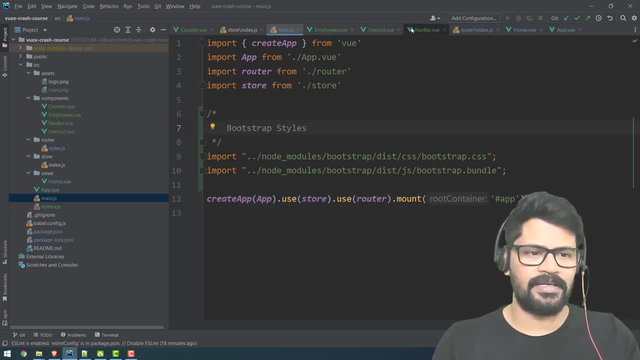 you store okay so with this store is gonna work so when you see back to our gonna work so when you see back to our gonna work so when you see back to our index yeah so now state data is empty so index yeah so now state data is empty so 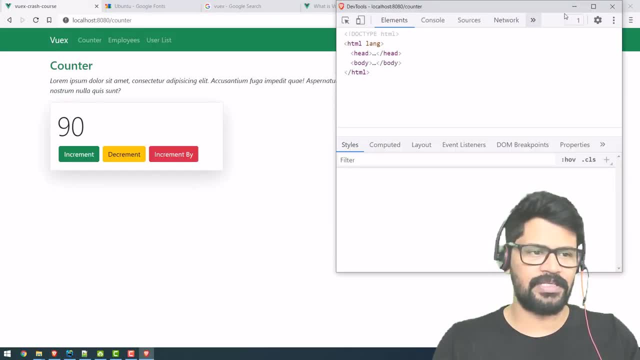 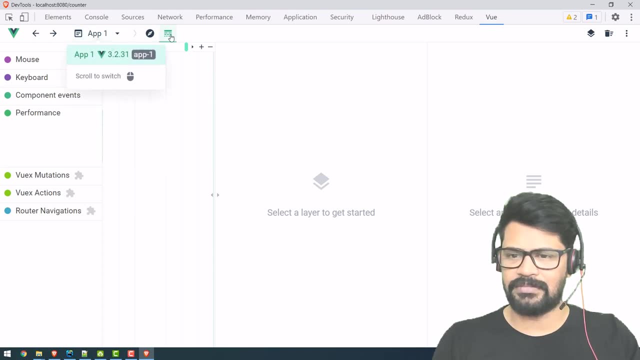 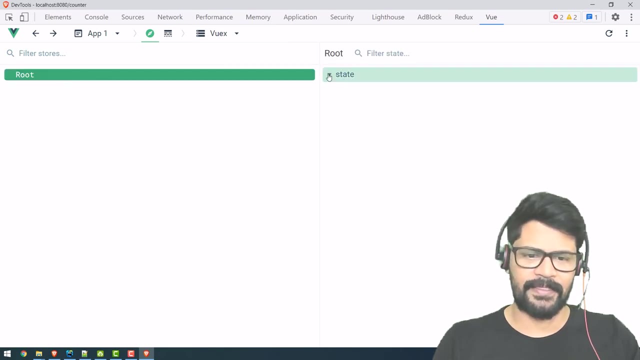 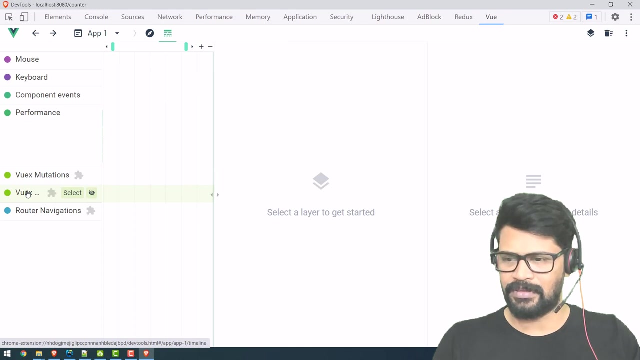 index yeah so now state data is empty so if state data is empty when you inspect if state data is empty when you inspect if state data is empty when you inspect and go with the dev tools of view J's and go with the dev tools of view J's and go with the dev tools of view J's okay you can search for view this dev okay you can search for view this dev okay you can search for view this dev tools so and here I'll search for a view tools so and here I'll search for a view tools so and here I'll search for a view X state okay now state data actually X state okay now state data actually X state okay now state data actually will be empty for example where you can will be empty for example where you can will be empty for example where you can see see see you excite state I think you actions no 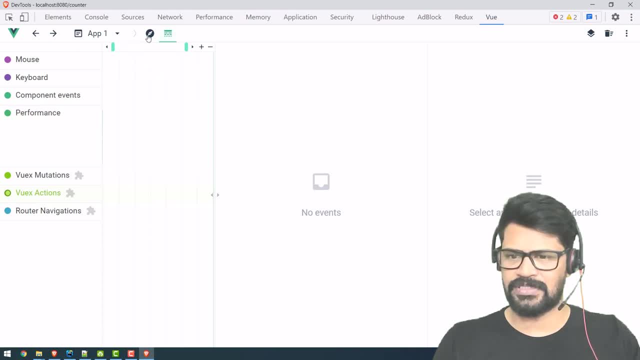 you excite state I think you actions no you excite state I think you actions no actions no mutations nothing okay it's actions no mutations nothing okay it's actions no mutations nothing okay it's not showing but state just empty state not showing but state just empty state 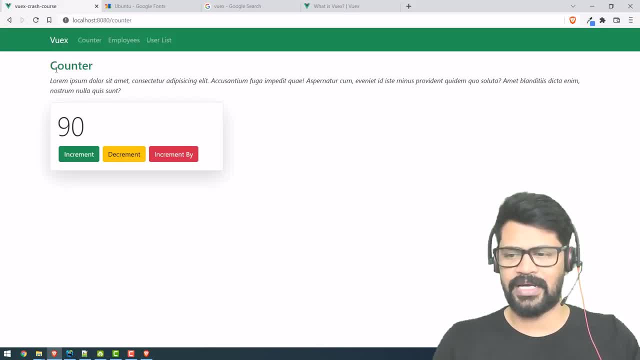 not showing but state just empty state okay fine so now what we have to do is okay fine so now what we have to do is okay fine so now what we have to do is we just need to increment this happens 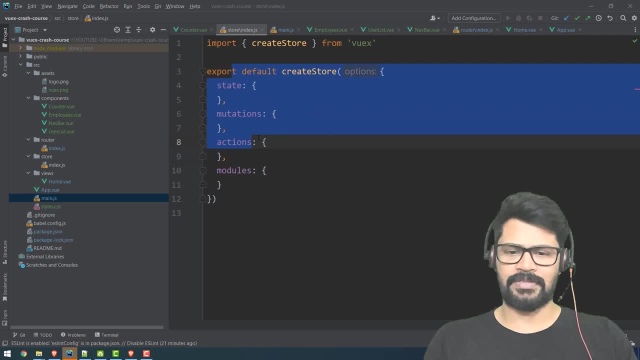 we just need to increment this happens we just need to increment this happens with the view X so to create a counter with the view X so to create a counter with the view X so to create a counter configuration in this actually one thing configuration in this actually one thing configuration in this actually one thing what we have to do is we just need to what we have to do is we just need to 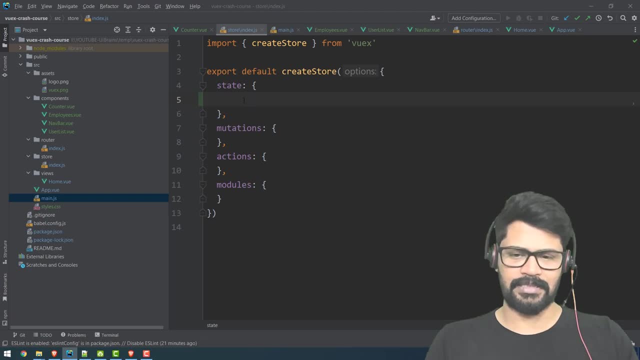 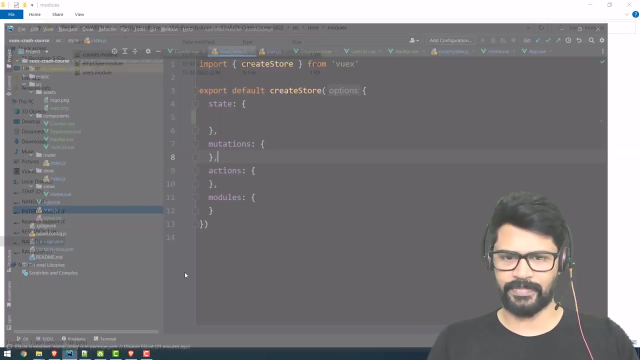 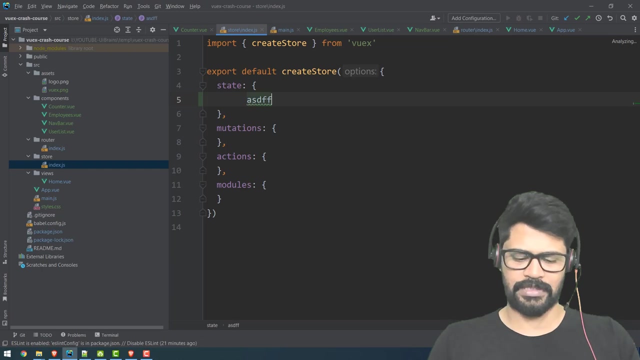 what we have to do is we just need to what we can do is you can create a state what we can do is you can create a state what we can do is you can create a state directly here in the come on I think directly here in the come on I think directly here in the come on I think it's stuck but man it's not allowing me it's stuck but man it's not allowing me it's stuck but man it's not allowing me to type anything it's working right then to type anything it's working right then to type anything it's working right then no sub problem once again go to store no sub problem once again go to store no sub problem once again go to store yeah it's working yeah one thing is you yeah it's working yeah one thing is you yeah it's working yeah one thing is you can configure the counter state and all can configure the counter state and all can configure the counter state and all here but the problem is if you can start 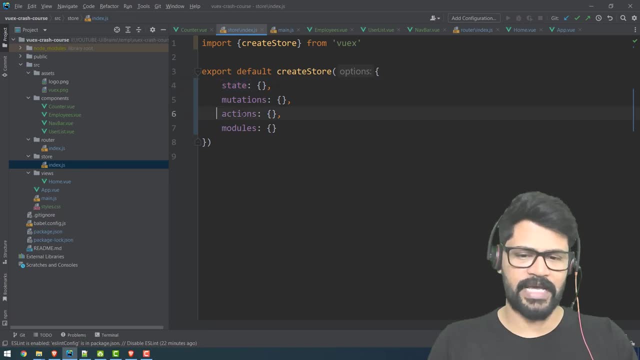 here but the problem is if you can start here but the problem is if you can start configuring everything so every state configuring everything so every state configuring everything so every state you have to configure here in every you have to configure here in every you have to configure here in every action you configure here so it will be action you configure here so it will be action you configure here so it will be like mess up because actions state like mess up because actions state like mess up because actions state everything you configure in one file it everything you configure in one file it everything you configure in one file it not actually looks good so for that we not actually looks good so for that we not actually looks good so for that we use actually modules concept so the plan use actually modules concept so the plan 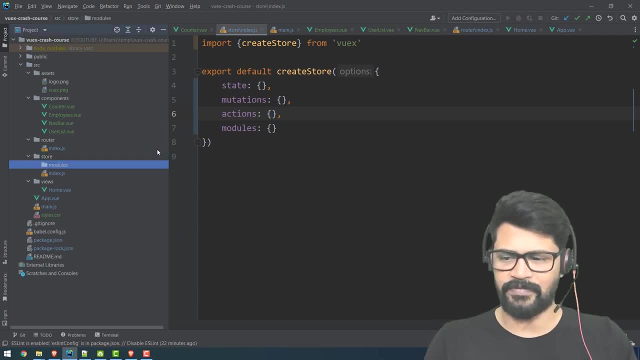 use actually modules concept so the plan is I create a new directory call modules is I create a new directory call modules is I create a new directory call modules so for every component I'll start with 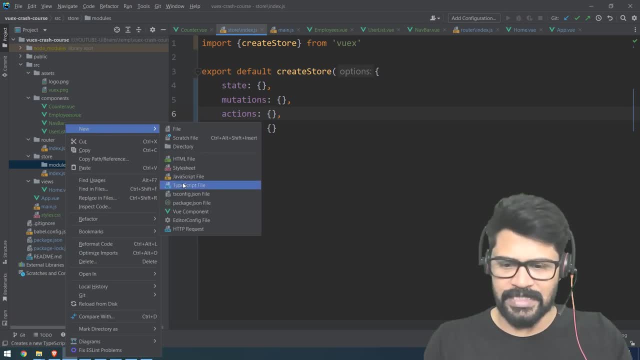 so for every component I'll start with so for every component I'll start with one modules okay in modules I create one 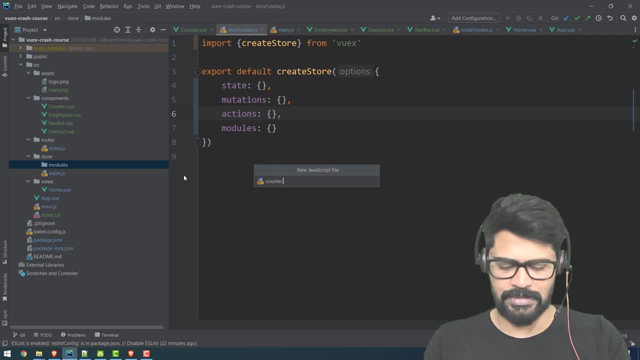 one modules okay in modules I create one one modules okay in modules I create one JavaScript that is counter dot module 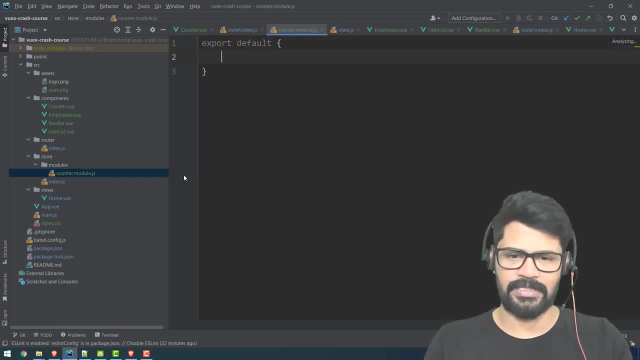 JavaScript that is counter dot module JavaScript that is counter dot module okay so here I say export default export 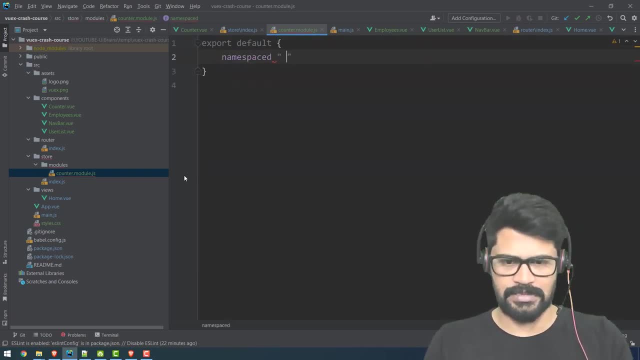 okay so here I say export default export okay so here I say export default export default I say name space it is true okay default I say name space it is true okay default I say name space it is true okay and in this I'll take state and and in this I'll take state and and in this I'll take state and mutation 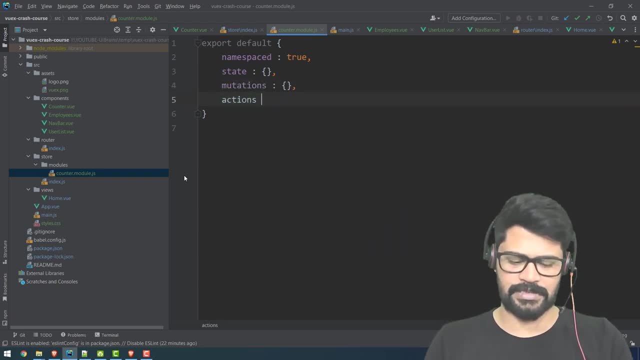 mutation mutation actions and actions okay so this is slightly different than your redux toolkit here we have 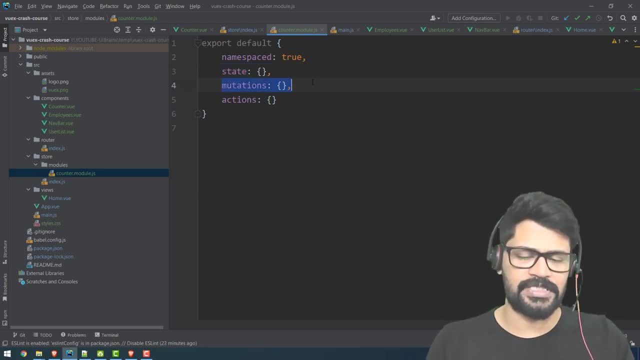 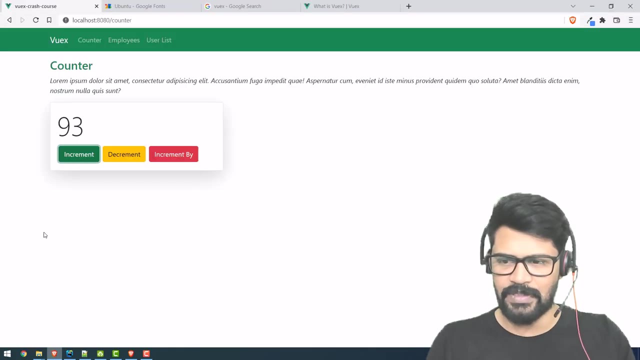 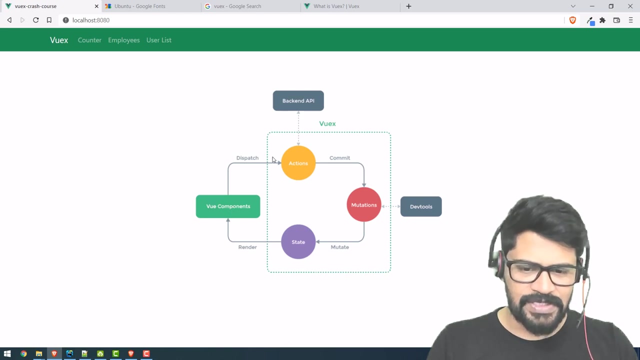 a state same like to have a redux store and mutations mutations are just like your reducers and actions is just like your actions okay when you when you take the diagram let me explain see this is your view component this is going to be dispatching an action okay that action will commits the mutation and that mutation will updates the state and it will run down the view 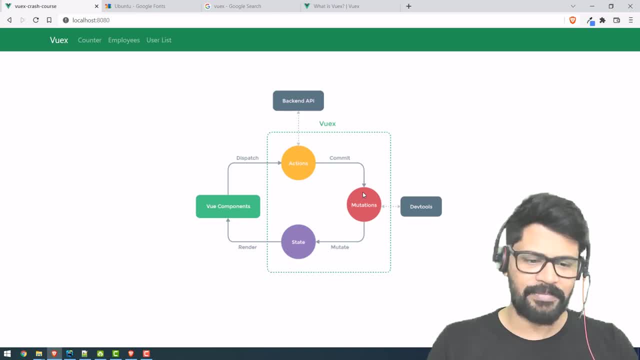 okay and this action itself is connect with a back-end api and this mutations also have connection with their dev tools the dev tools which we have open okay so now story is only between these four so actions mutations and state so actions we're going to execute and mutations are just like a reducer so which will update your state data okay so how you configure 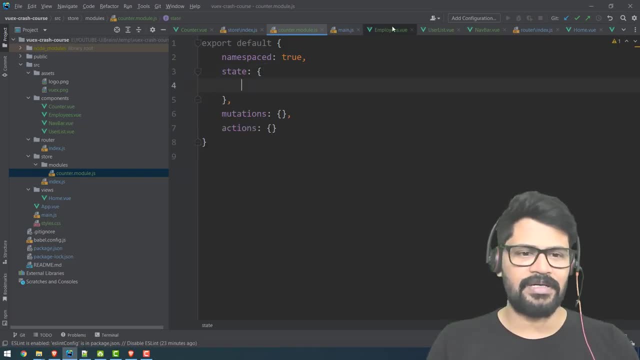 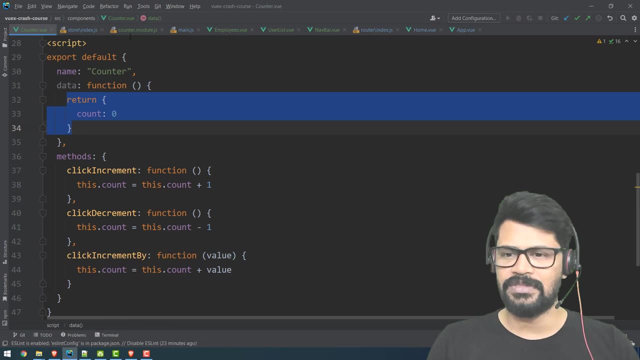 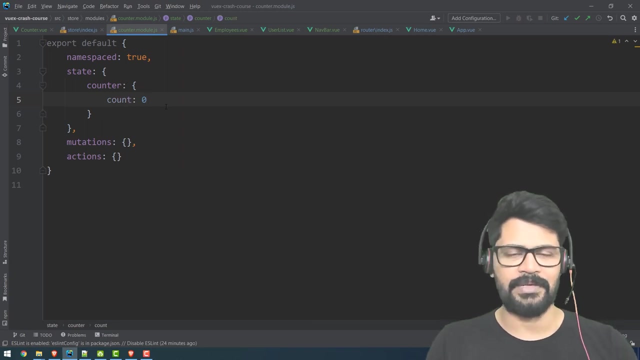 them is first we start with the stator so first of all when you go with your counter so what was the state you taken this discount zero so same thing what you have to do is this a counter where count value zero okay that's to become your stator and mutations mutations are just like your reducer 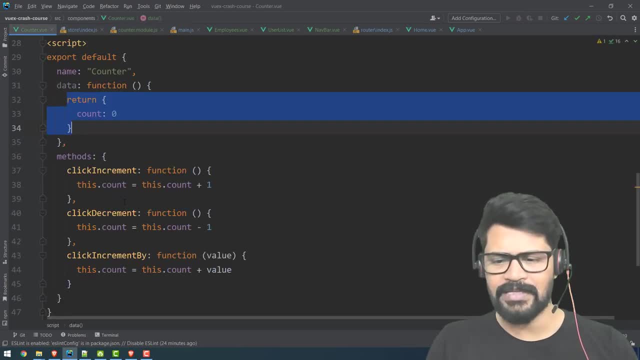 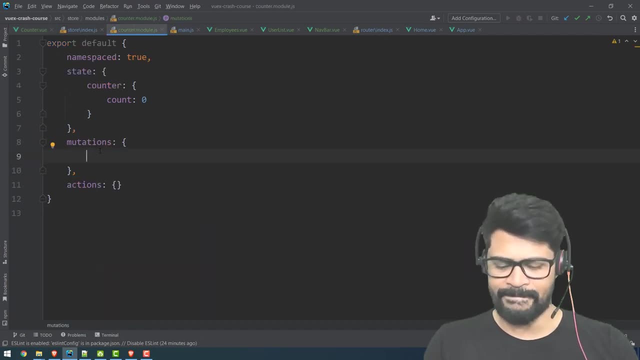 so I have three activities have to make increment decrement and increment by okay so what you do is increment counter okay I'll take like this increment counter is a function increment counter is a function which will take up the state and what it does is this dot counter no no I think is state 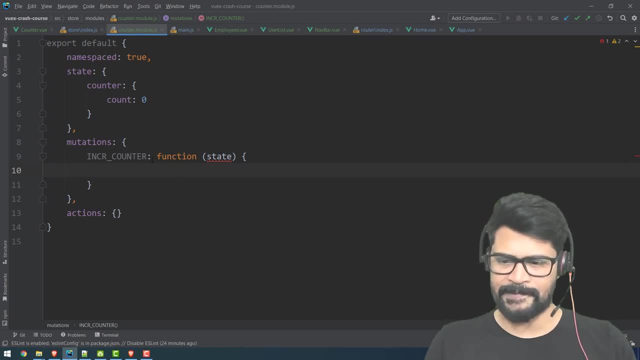 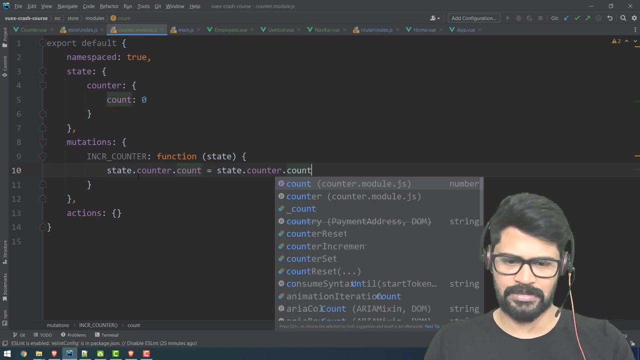 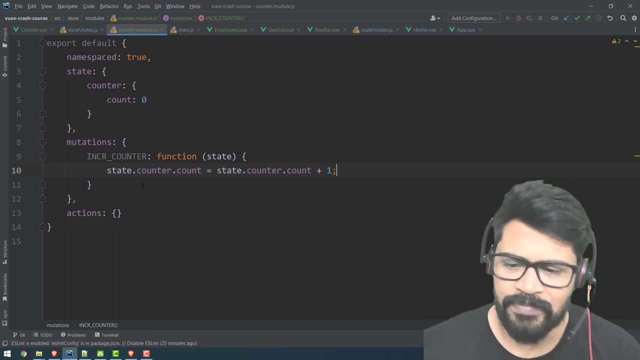 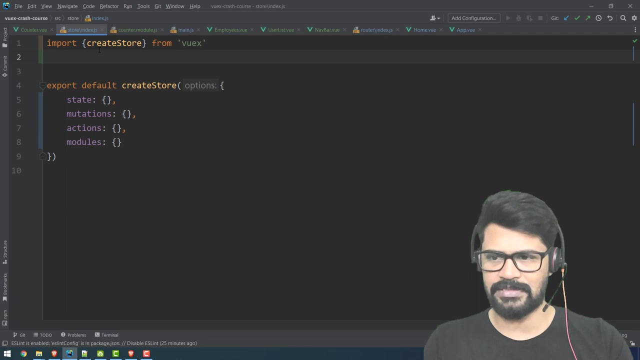 Haushara counter dot new is now count can be Titans is no we need for our stator to count yeah so state dot counter dot count is equal to state sings yeah so state dot counter dot count is equal to state fuse here for the all functions yes we have different functions we have like static mesa so we get all the functions that we want in this such functionusz tough we have different functions we may not have any functions so but this was not giving a proper hint for you uh to to have a proper hint for you first as soon as you create a counter module so you have to configure it with the store so how you configure is the root store import counter module from this counter module and now what you do is state state counter state will be counter module dot state so this is the configuration and also no mutation to configure because we have mutations and actions taken inside the module only 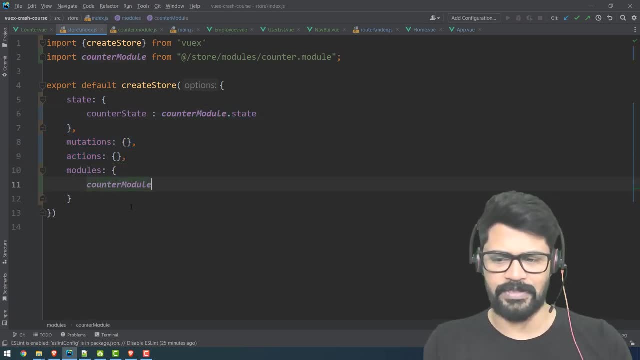 and you can configure the module that is my counter module the only thing is as soon as you 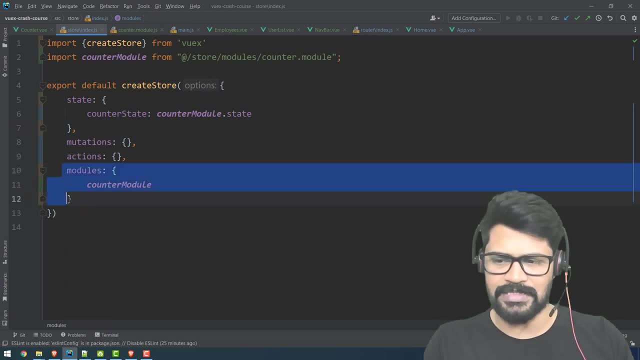 create a module you must have to register with this modules and the state so that it will have an idea what is that activity you are going to perform 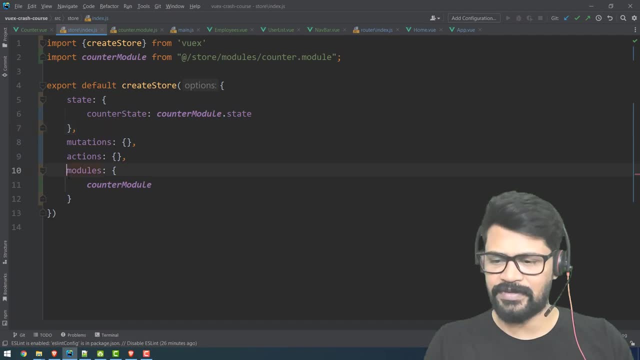 and as soon as i have uh as soon as i have uh i configured this counter module in my global state 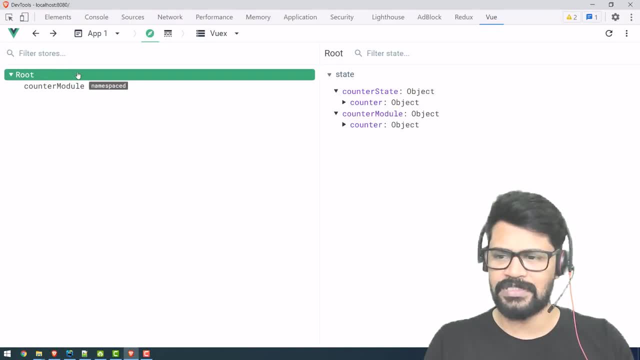 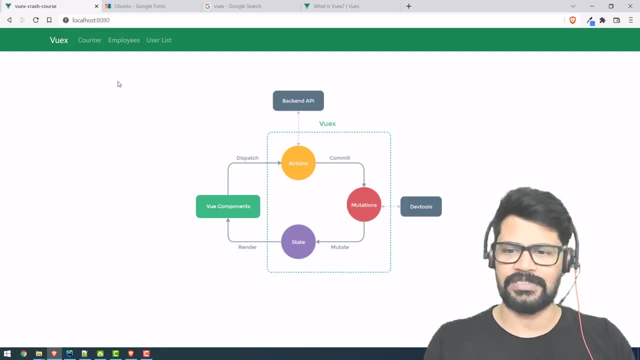 so what happens is if you refresh and go with the dev tools so you can find see counter module has been configured with the state data counter with count zero okay so that's what the counter data 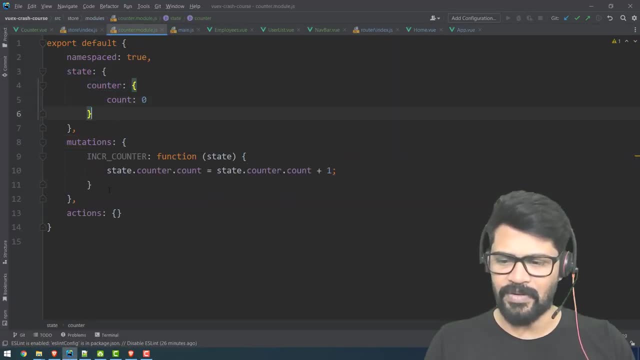 which we have uh configured state okay and this is done now let's say decrement 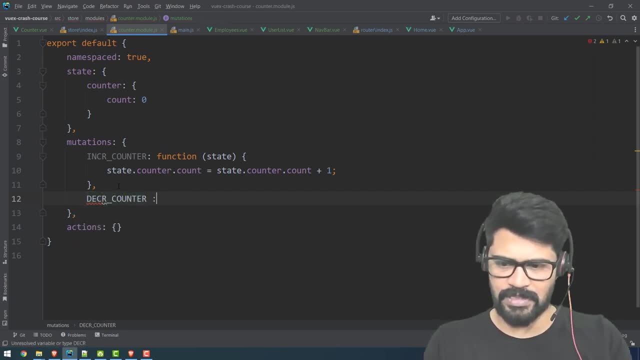 decrement decrement ecr underscore counter is one function that will take up the state again 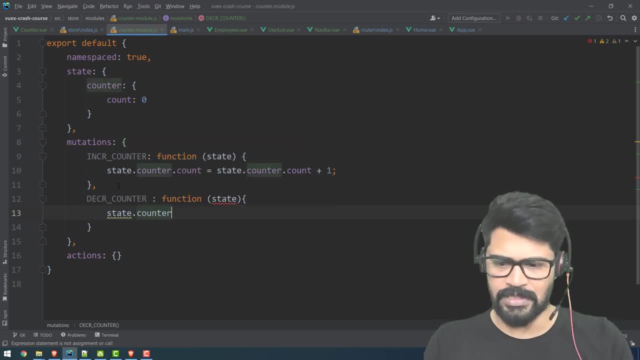 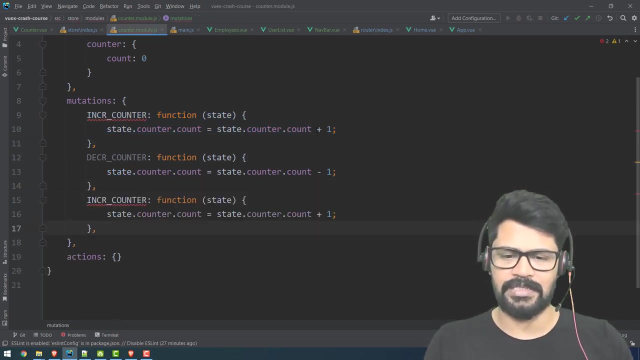 okay so state dot counter dot count is equal to state dot counter dot count minus 1. okay and one more thing is increment by so this will take see uh this is just take one and one this will take actually payload so 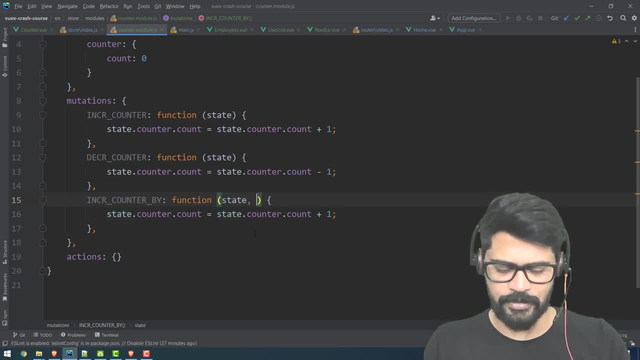 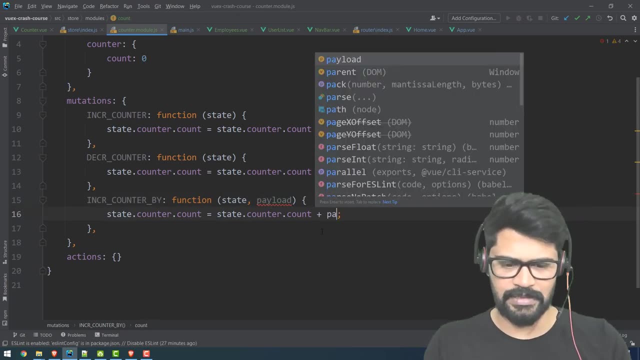 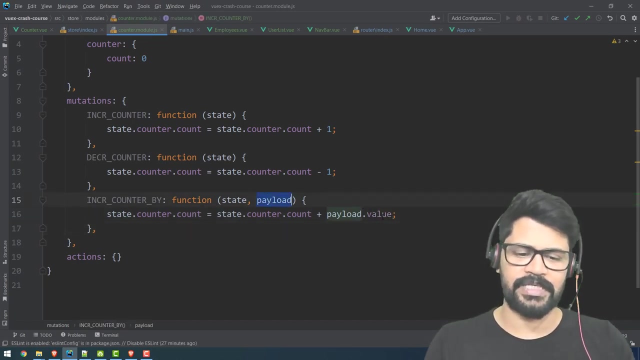 increment buys and how we can take the payload is the second option you take the payload okay so you may write payload dot value okay so payload is actually an object so in that the value what you have passed that will update 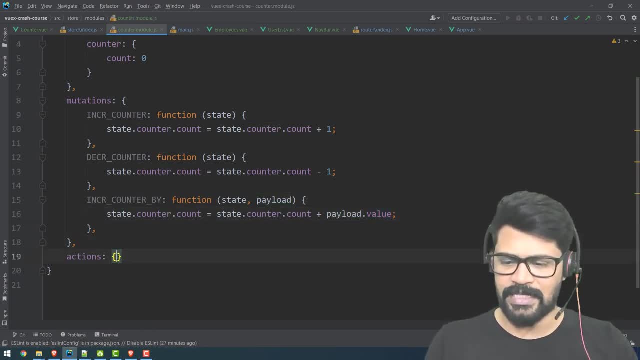 to the counter okay i have three mutations and let's create actions for them so let's say 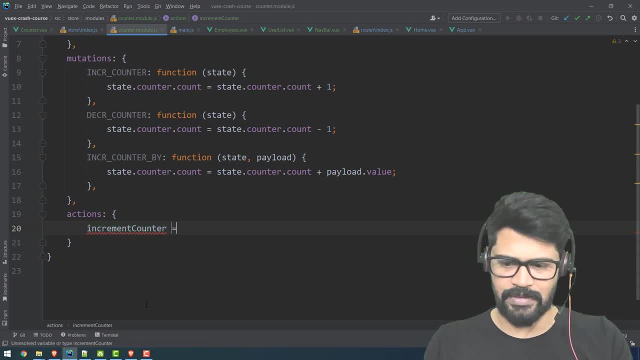 increment increment counter is equal is a function so what happens is it will return this this will take something called commit because as for the diagram it will commit the mutation okay so commit the mutation which i want is increment the counter 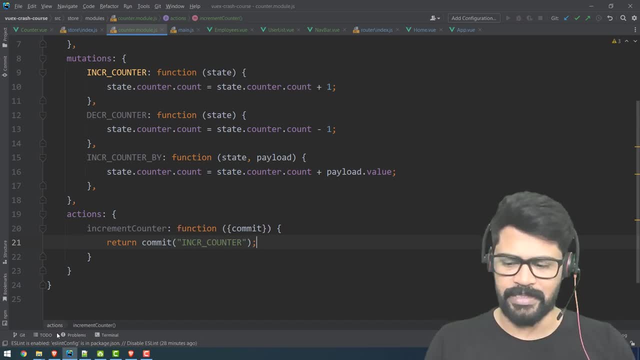 see i'll show you why this commit see on the home page see this 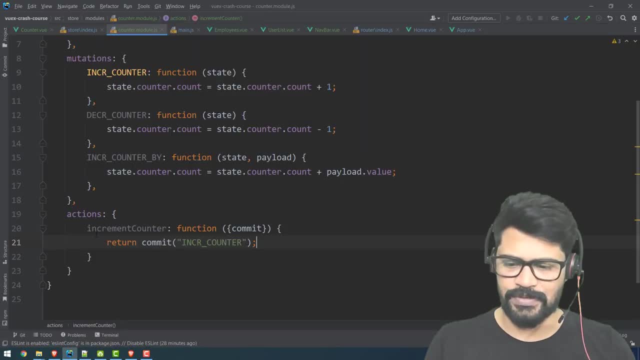 so this action is going to commit the mutation okay so in the this action is going to commit my 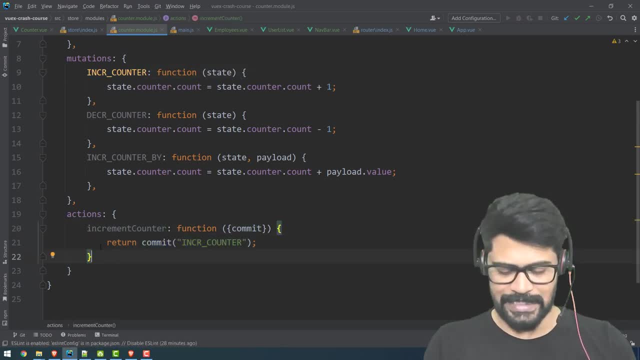 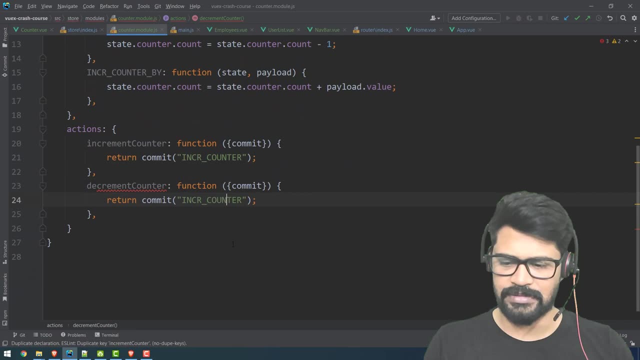 mutation increment counter okay same way i'll take the other one this is decrement counter okay so this will make decrement counter commit and then increment 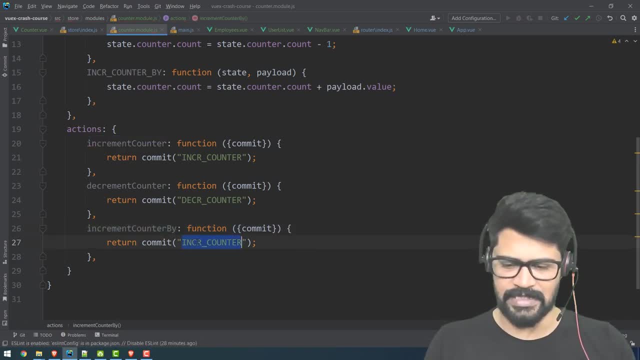 counter by is my action so let's say increment counter by okay it's going to commit but this saves your time here so this is a function it will also give you all the options you need 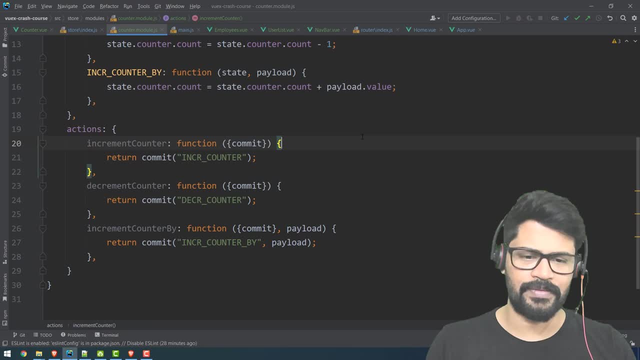 okay so using what p a as i have created you can忘i your expression i mean last abit 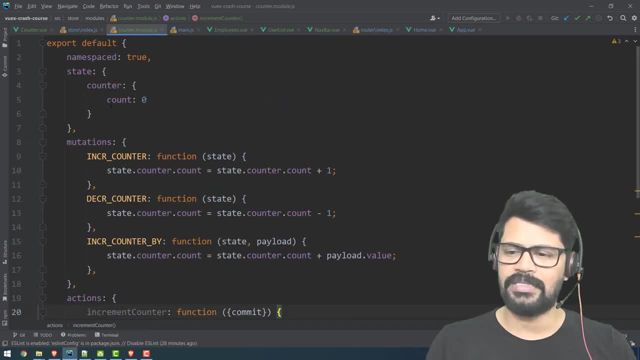 but one more thing is this is taken extra call payload so you will get a payload as a second parameter you can pass on the payload as a second parameter as it is what you have passed okay it 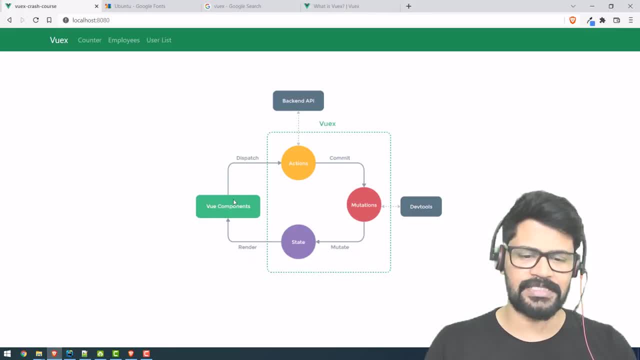 should be an object with a value okay fineeden ah случай so we got 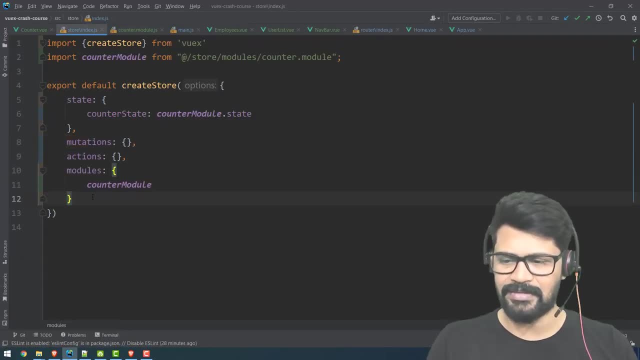 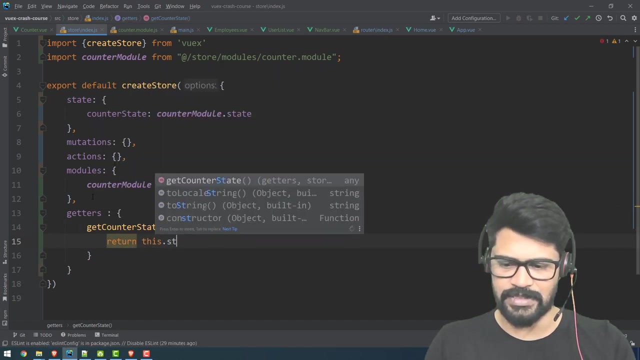 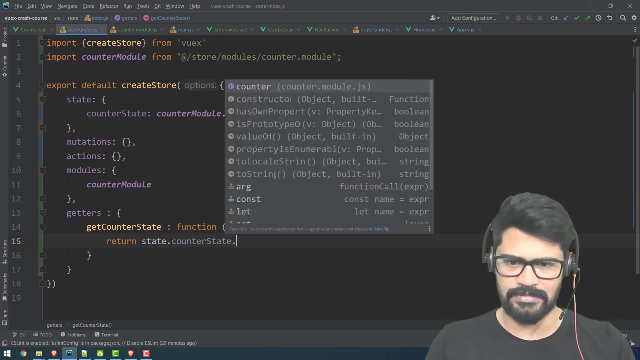 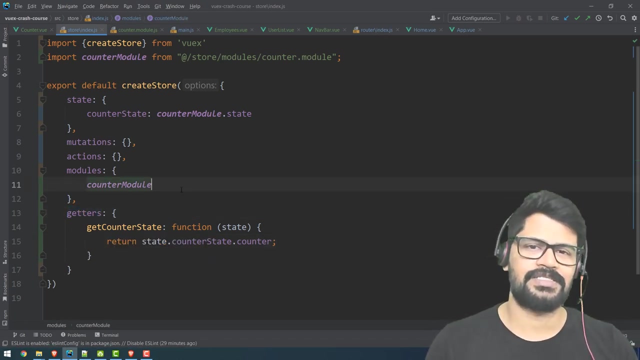 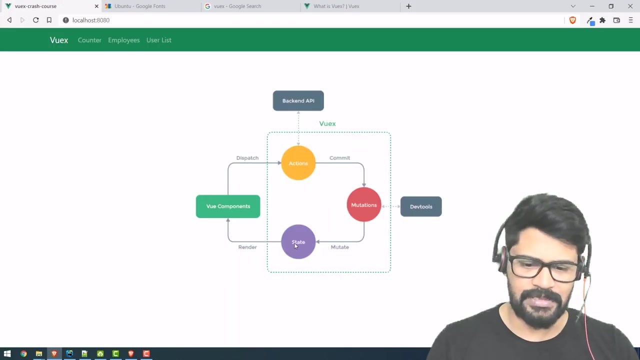 start with the connection I go to store here I will add I will add the getters I will add some getters so get counter get counter state so how can you fetch the counter state is this is a function is going to return this dot this dot okay actually this will take up the state as a parameter so state dot counter state dot counter okay so this is one getter function because you want to fetch generally in react.js we use a useSelector hook but in view.js we need to write some getter function so that will fetch your counter because the specific state data if you want to fetch it for your what's called component okay because here 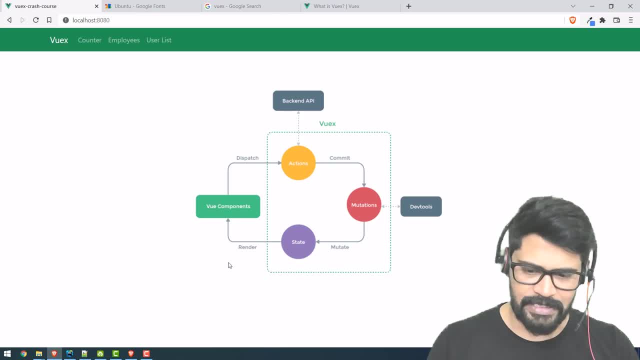 this state in the component we need to get data from the state so that should be 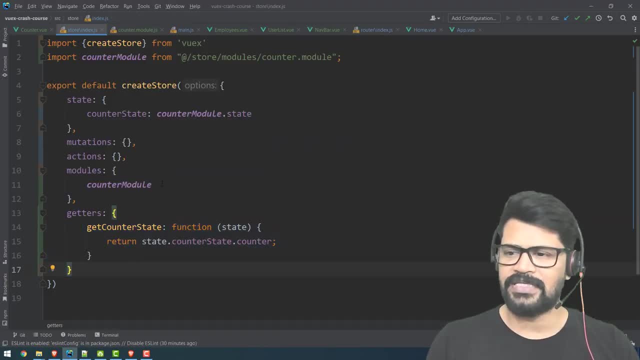 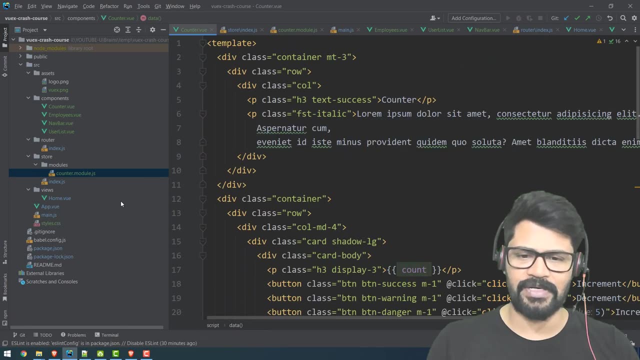 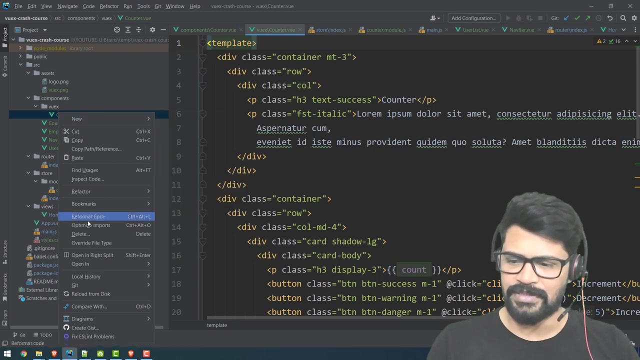 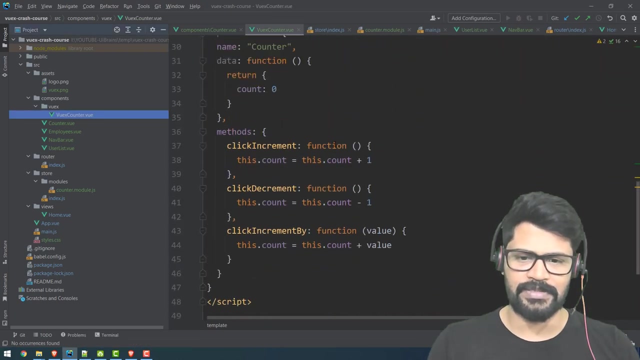 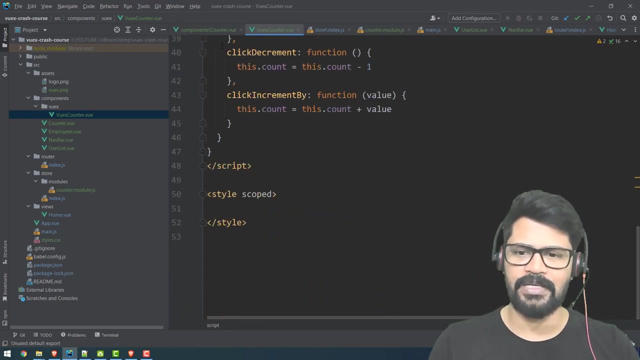 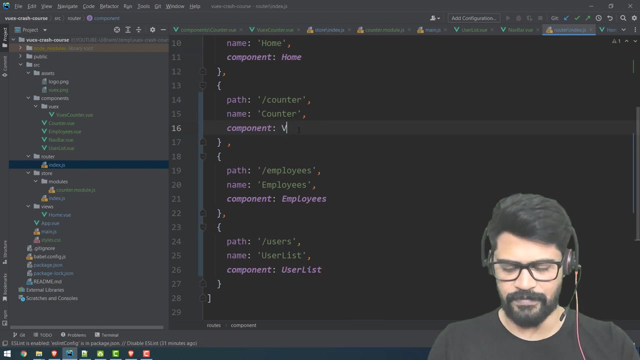 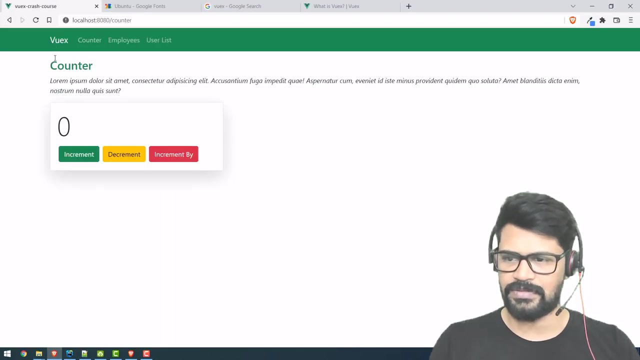 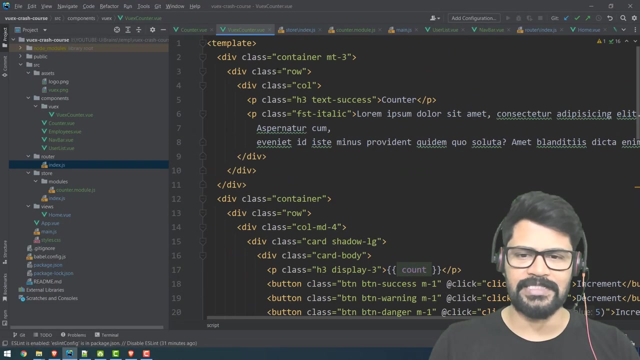 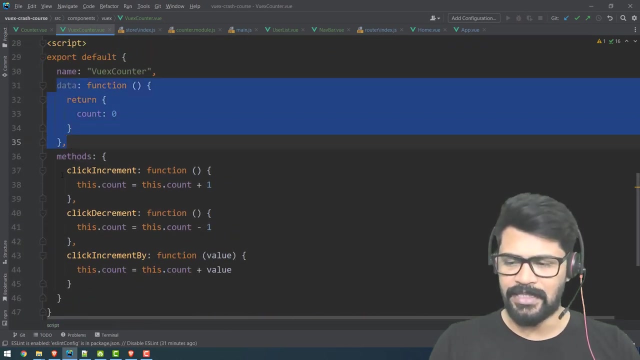 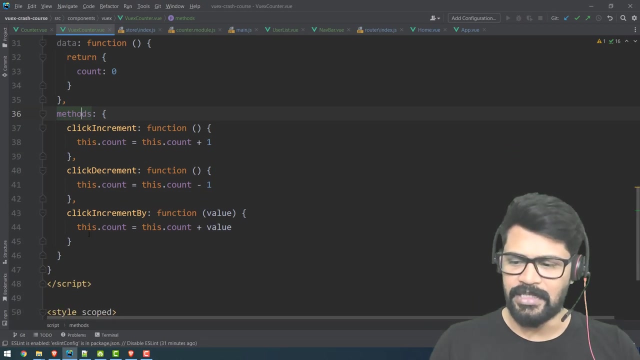 this using getter okay so everything is done now jump into the counter but before I jump into counter I don't want to touch this file for counter so what I do is I just create a viewX counter and then I'll update so what you do is in the same components the same components I create one more folder for viewX so let's copy this and keep it in this and I'll change it to rename as rename as UX counter okay so this will be a view X counter I just change the name okay and where you are to change it in the router I'll just change this to view X counter okay now it's UX counter okay so it should work with the local data okay fine if I switch between is gone okay fine so we have taken a separate component the same setup now the next step is I don't need to have a local data and I don't need to have local state management the very first thing is I want to get the you know state data how we get state data is there is a predefined property called compound computed property which is here map getters map getters this will import from the view X map getters will import 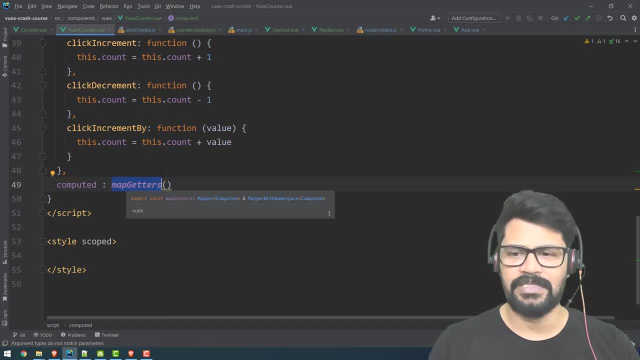 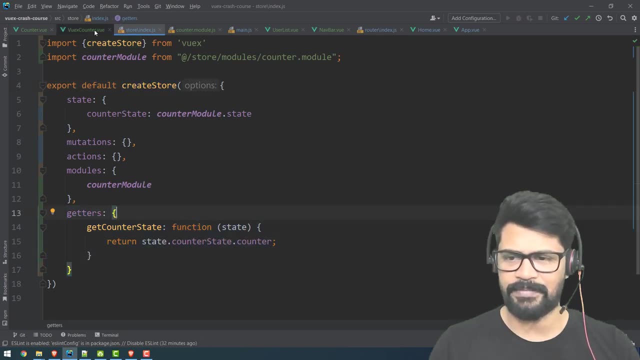 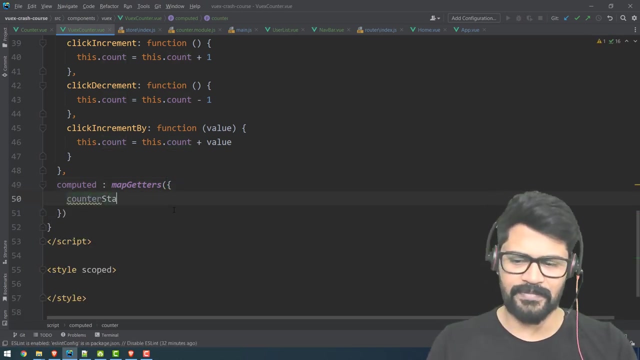 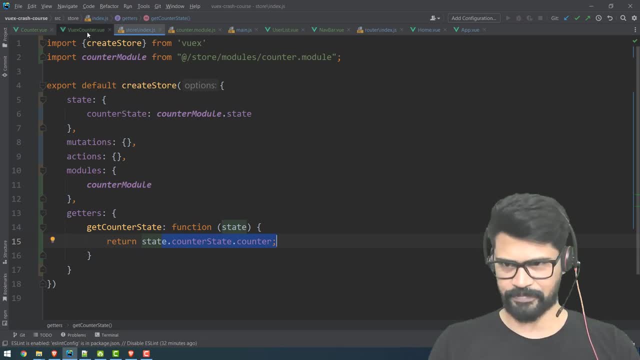 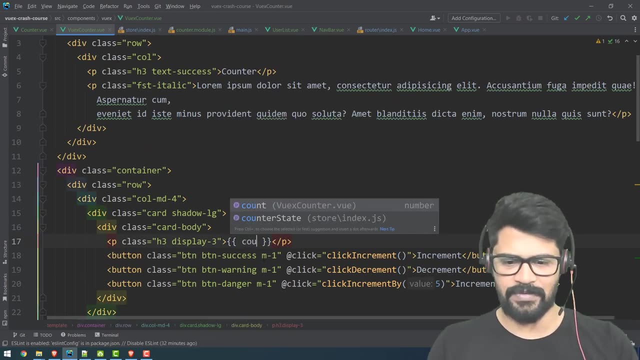 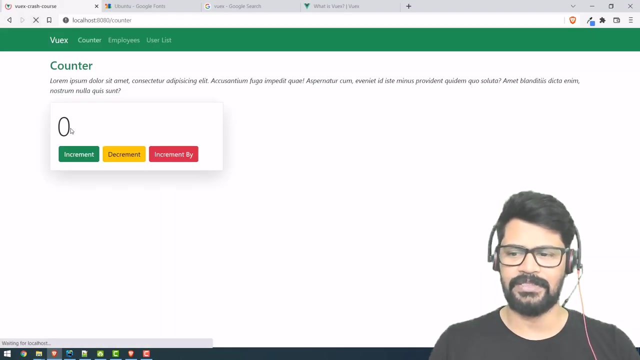 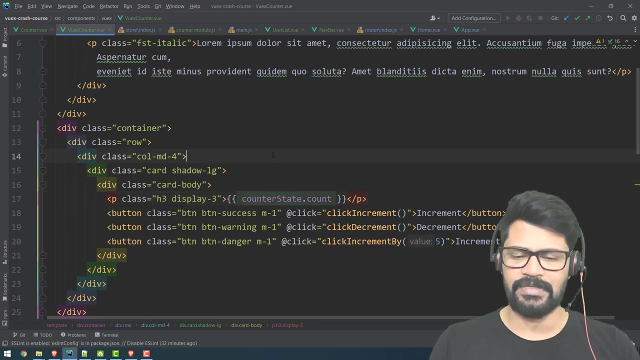 counter state that's all so what happened this function returns me the happened this function returns me the happened this function returns me the counter state that assigned to the counter state that assigned to the counter state that assigned to the variable called counter state so now what variable called counter state so now what variable called counter state so now what I do is in this counter I'll say I do is in this counter I'll say I do is in this counter I'll say counter state dot count so what happened counter state dot count so what happened counter state dot count so what happened it's a value zero so now this zero is it's a value zero so now this zero is it's a value zero so now this zero is going to even conform you go to module going to even conform you go to module going to even conform you go to module and I'll change this to 10 so what 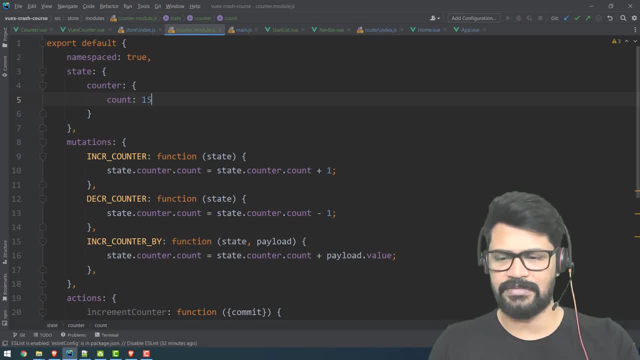 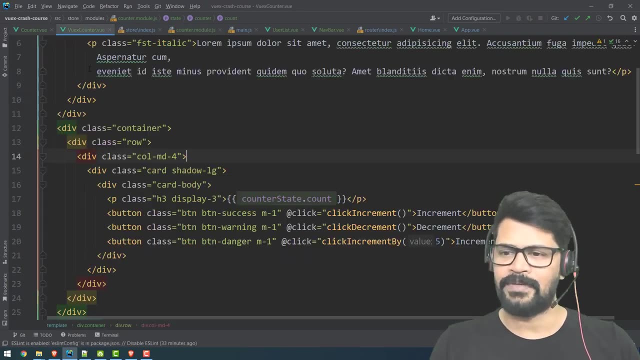 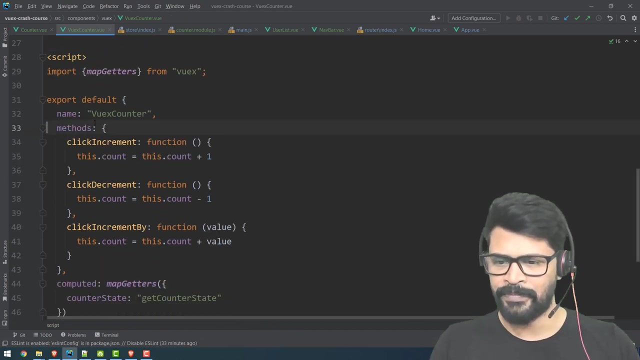 and I'll change this to 10 so what and I'll change this to 10 so what happened is become 10 I'll change to 15 happened is become 10 I'll change to 15 happened is become 10 I'll change to 15 is become 15 okay that way I'll make it is become 15 okay that way I'll make it is become 15 okay that way I'll make it zero so it's zero okay now this is done zero so it's zero okay now this is done zero so it's zero okay now this is done this is has been configured the state this is has been configured the state this is has been configured the state now I don't need to maintain the local now I don't need to maintain the local now I don't need to maintain the local data anymore and I don't need to have data anymore and I don't need to have data anymore and I don't need to have functions like this okay I have to call functions like this okay I have to call 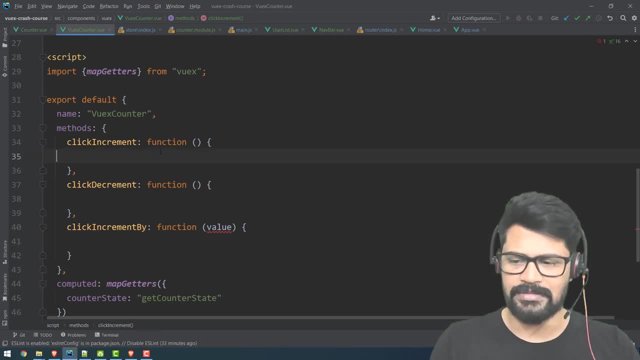 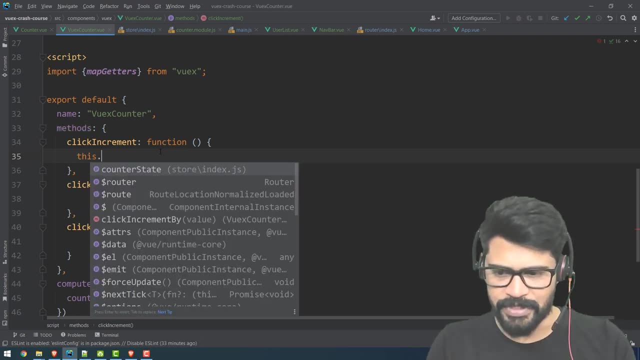 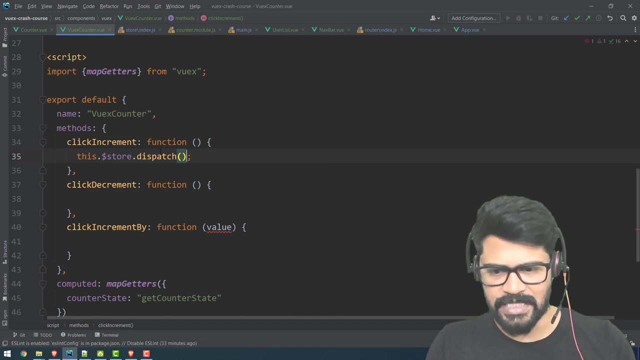 functions like this okay I have to call action because I have to call dispatch action because I have to call dispatch action because I have to call dispatch actions so this thought you can have actions so this thought you can have actions so this thought you can have access to store directly using the access to store directly using the access to store directly using the property called this dot store directly property called this dot store directly property called this dot store directly dot dispatch dispatch you have to dot dispatch dispatch you have to dot dispatch dispatch you have to dispatch an action what is the action is dispatch an action what is the action is dispatch an action what is the action is counter module the the module what you have created slash the action okay and have created slash the action okay and 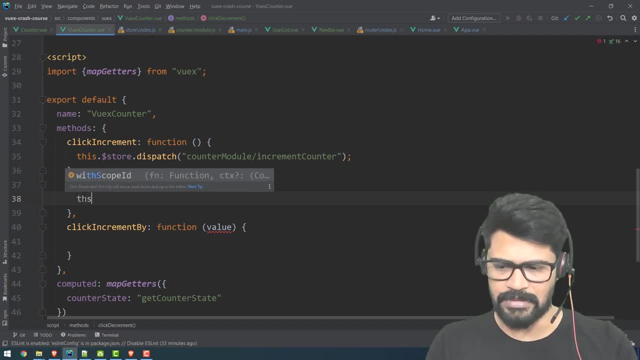 have created slash the action okay and same story here this dot dollar store same story here this dot dollar store same story here this dot dollar store dot dispatch so here I'm gonna specify dot dispatch so here I'm gonna specify 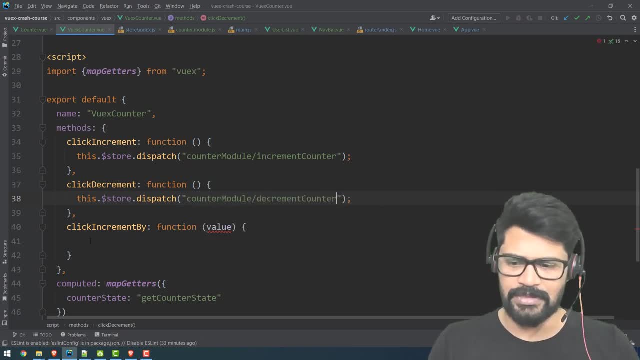 dot dispatch so here I'm gonna specify counter module slash decrement counter counter module slash decrement counter counter module slash decrement counter okay and for this one I have to call 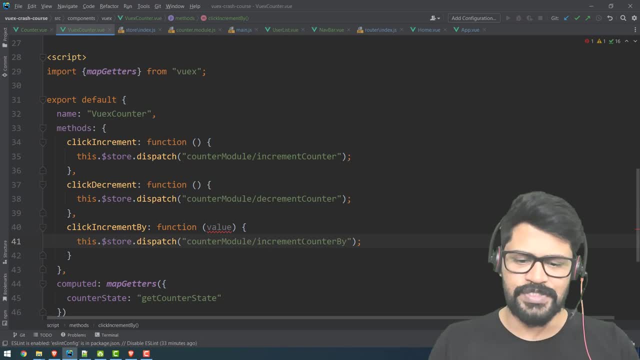 okay and for this one I have to call okay and for this one I have to call this is increment by but this should this is increment by but this should this is increment by but this should accept one extra accept one extra accept one extra parameter because as for my module parameter because as for my module parameter because as for my module configuration which will take up the 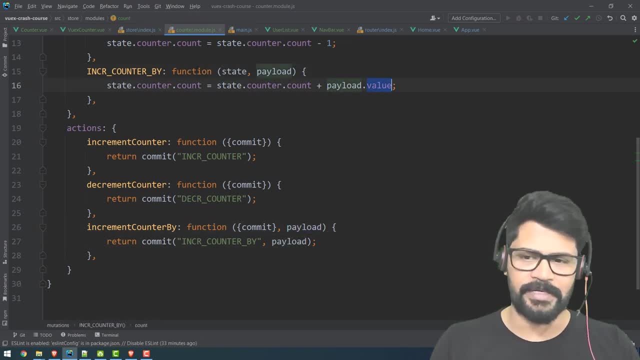 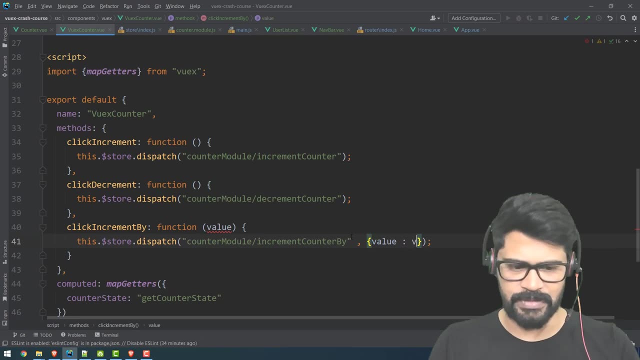 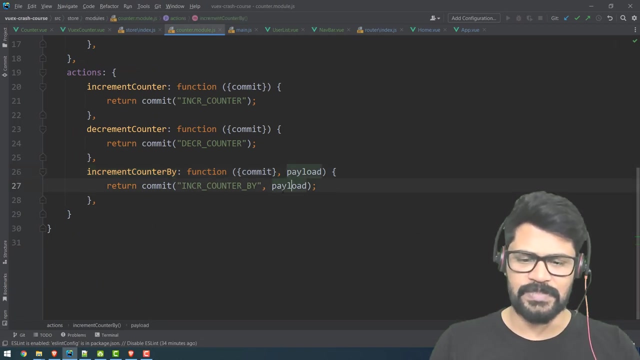 configuration which will take up the configuration which will take up the payload but payload is an object which payload but payload is an object which payload but payload is an object which contains a value as a property so what contains a value as a property so what contains a value as a property so what you do is comma an object where the you do is comma an object where the you do is comma an object where the value goes to be my value okay this will value goes to be my value okay this will value goes to be my value okay this will become your payload so this payload will become your payload so this payload will become your payload so this payload will take in for this function this payload take in for this function this payload take in for this function this payload it is committing this mutation and this it is committing this mutation and this 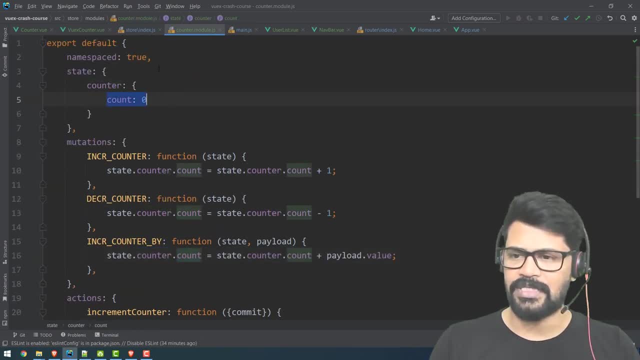 it is committing this mutation and this payload will update your counter and payload will update your counter and payload will update your counter and this counter and that counter can be this counter and that counter can be 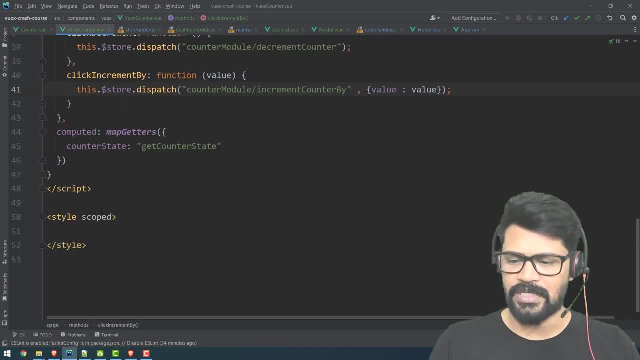 this counter and that counter can be accessed by this getter to this your accessed by this getter to this your accessed by this getter to this your component and that state data we were component and that state data we were 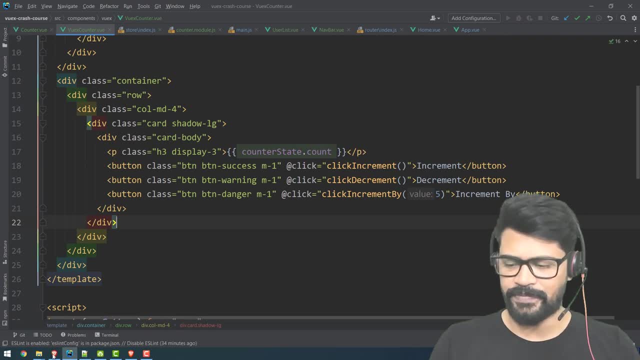 component and that state data we were displaying here okay so now check displaying here okay so now check 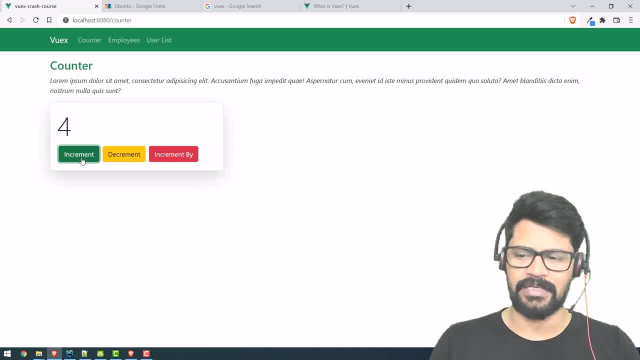 displaying here okay so now check refresh this increment the counter is refresh this increment the counter is refresh this increment the counter is incrementing and you want to see this incrementing and you want to see this incrementing and you want to see this state actions and all you go to the dev state actions and all you go to the dev state actions and all you go to the dev tools you can select the second option 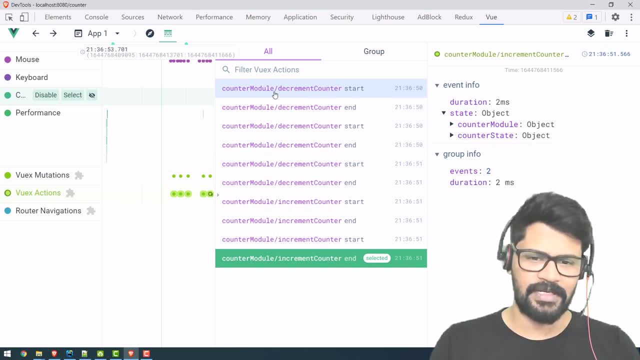 tools you can select the second option tools you can select the second option yeah view X actions yeah you have action yeah view X actions yeah you have action yeah view X actions yeah you have action so increment counter decrement counter so increment counter decrement counter so increment counter decrement counter everything was started and incremented everything was started and incremented everything was started and incremented everything is still there okay and you everything is still there okay and you everything is still there okay and you want to see the state data now the want to see the state data now the want to see the state data now the counter value is 4 like that decrement is 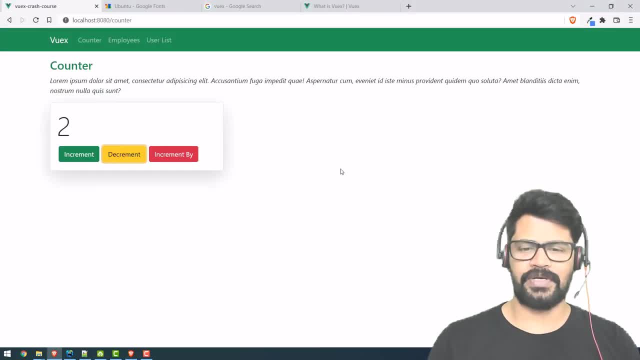 counter value is 4 like that decrement is 2 now it's 2 okay so you can easily 2 now it's 2 okay so you can easily 2 now it's 2 okay so you can easily track the actions and the state data track the actions and the state data track the actions and the state data here okay fine and one last check we can here okay fine and one last check we can here okay fine and one last check we can watch we have to do is when I increment watch we have to do is when I increment watch we have to do is when I increment and I move on to another component and and I move on to another component and and I move on to another component and came back it is still there right I move came back it is still there right I move came back it is still there right I move on to the employees and came back it is on to the employees and came back it is on to the employees and came back it is still there so now this counter is 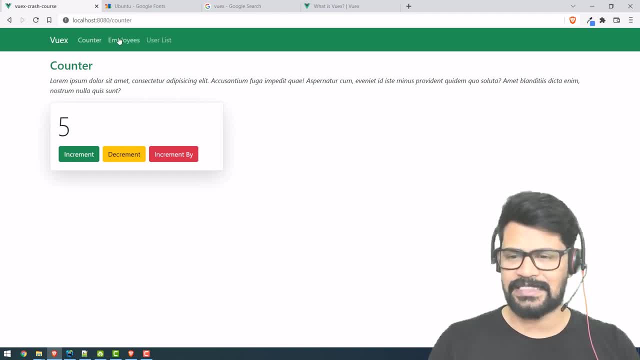 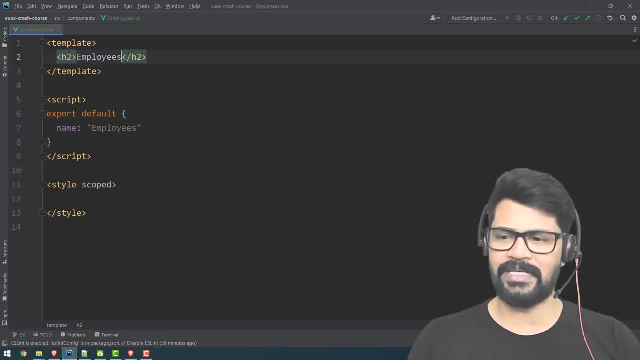 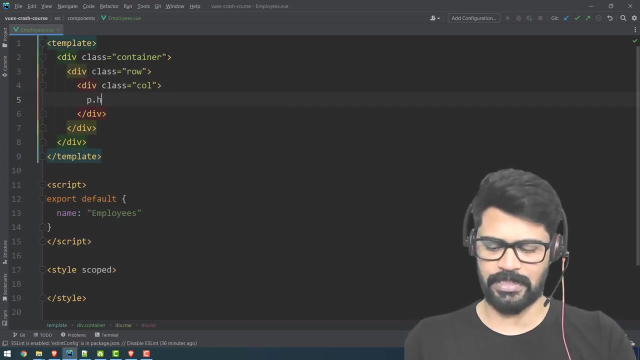 still there so now this counter is still there so now this counter is completely converted to view X so now completely converted to view X so now let's start with employees so now for let's start with employees so now for let's start with employees so now for employees what you do is go to components employees what you do is go to components employees what you do is go to components called employees so let's make the what's called employees so let's make the what's called employees so let's make the what's called design okay yeah so I will start called design okay yeah so I will start called design okay yeah so I will start with one container one row will column with one container one row will column with one container one row will column let's say P dot h3 employees and let's let's say P dot h3 employees and let's let's say P dot h3 employees and let's say take success and I have one para say take success and I have one para say take success and I have one para draw to the class one Sally talik and 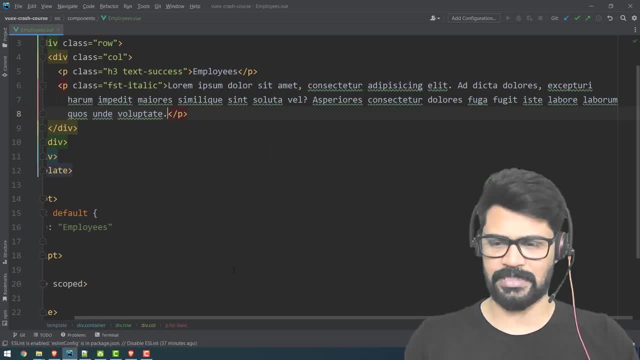 draw to the class one Sally talik and draw to the class one Sally talik and Lauren 30 tap just as a basic heading Lauren 30 tap just as a basic heading Lauren 30 tap just as a basic heading and I also say margin top three okay 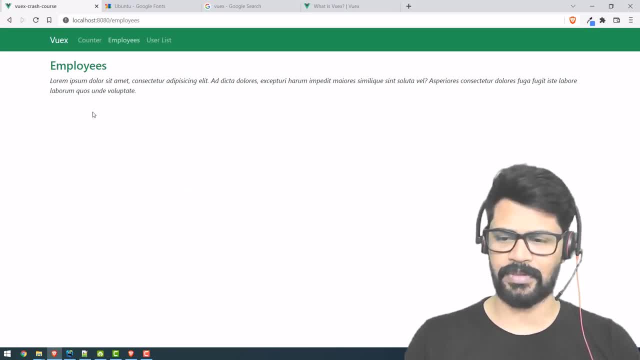 and I also say margin top three okay and I also say margin top three okay and under that I need to have you know and under that I need to have you know and under that I need to have you know list of employees yep so can we start list of employees yep so can we start 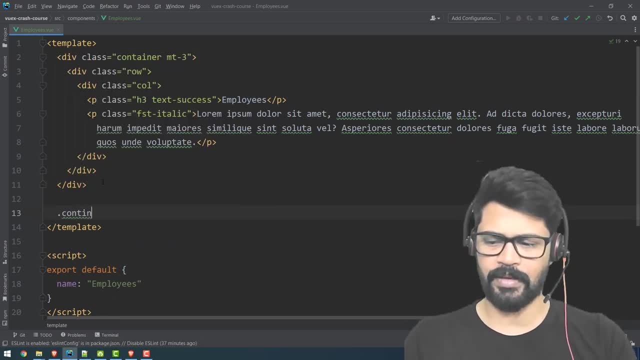 list of employees yep so can we start with another container container row and with another container container row and with another container container row and column D the stick six tab yeah in this column D the stick six tab yeah in this 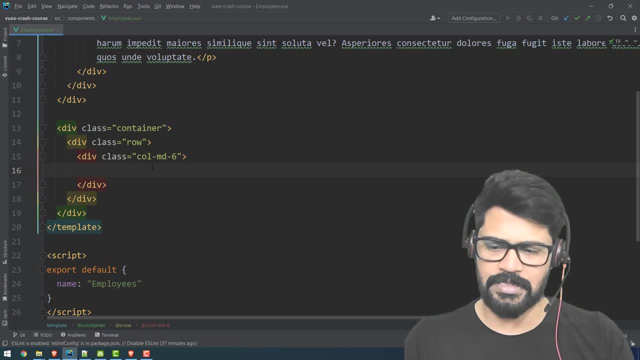 column D the stick six tab yeah in this I need to have all the list of employees I need to have all the list of employees I need to have all the list of employees so but we were before that I need to so but we were before that I need to 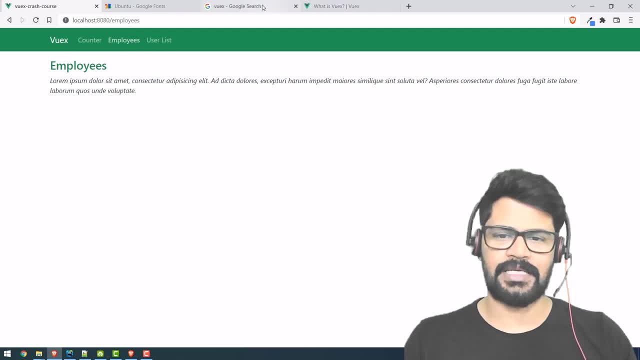 so but we were before that I need to have employees data so for that have employees data so for that have employees data so for that employees data yes I'm using the the employees data yes I'm using the the employees data yes I'm using the the regular Jason placeholder users yeah regular Jason placeholder users yeah 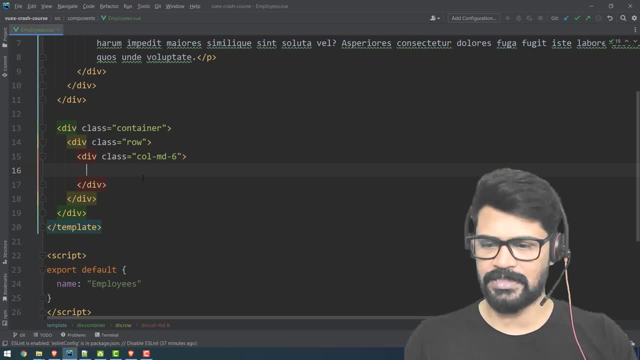 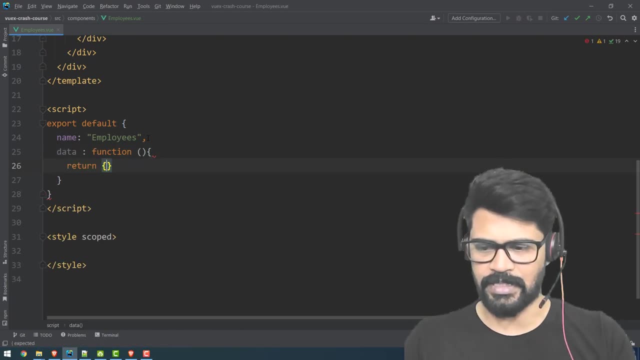 regular Jason placeholder users yeah this one so let's take up the fields this one so let's take up the fields this one so let's take up the fields how do you take the state data that is how do you take the state data that is how do you take the state data that is data is a function that returns an object 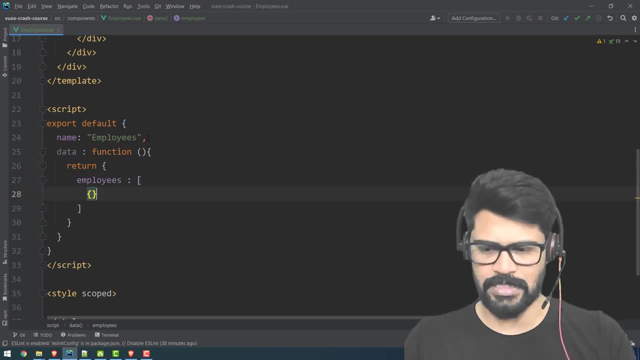 data is a function that returns an object data is a function that returns an object where employees will be an array in that where employees will be an array in that where employees will be an array in that the first object is ID and second the first object is ID and second 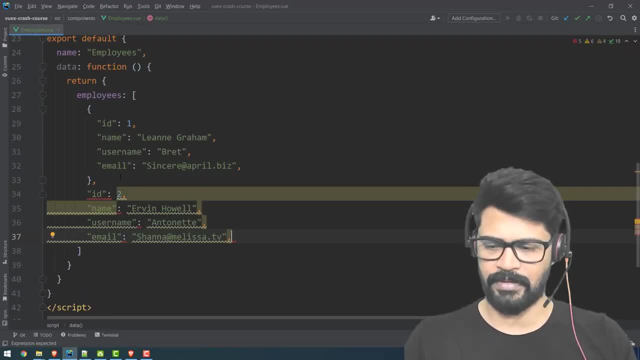 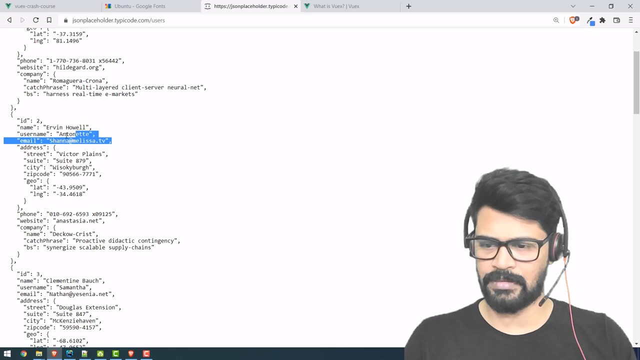 the first object is ID and second object sorry okay object sorry okay object sorry okay and and and and and and third one quickly will make 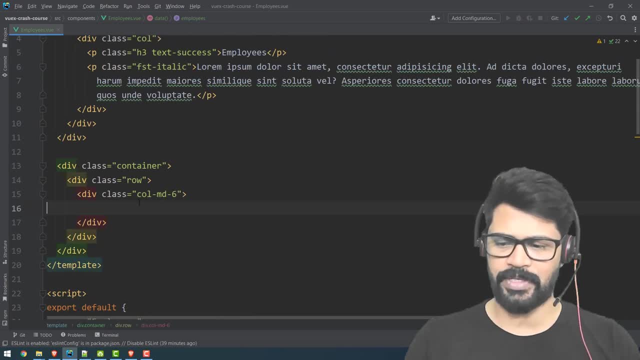 okay so five employees data is there now okay so five employees data is there now okay so five employees data is there now what I do is here 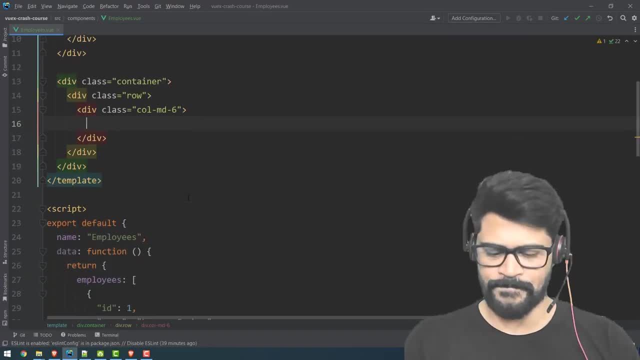 what I do is here what I do is here back here so I have to loop through and back here so I have to loop through and back here so I have to loop through and display so I'll write you well in this display so I'll write you well in this 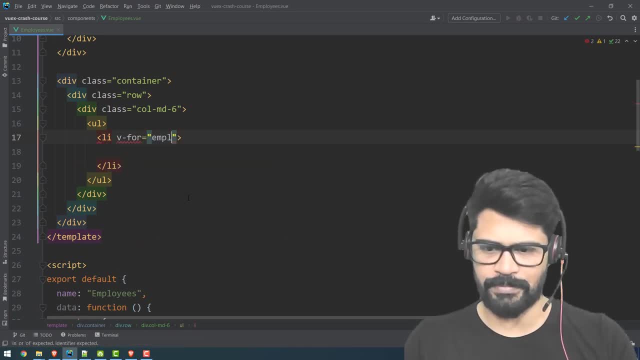 display so I'll write you well in this ally so here I write V for employee of ally so here I write V for employee of ally so here I write V for employee of employees and also let's add a key that employees and also let's add a key that employees and also let's add a key that is employee dot ID and let's add employee is employee dot ID and let's add employee 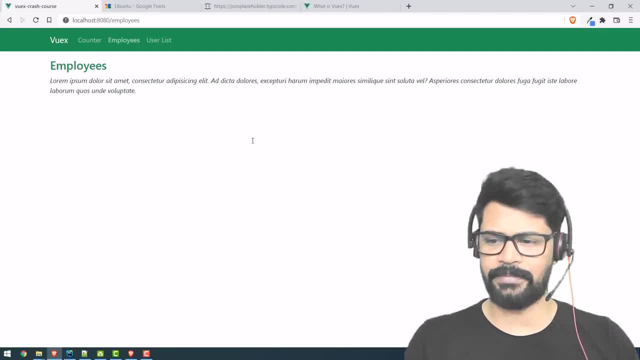 is employee dot ID and let's add employee dot name so you get the name yep dot name so you get the name yep dot name so you get the name yep so let's give us classes to say list to so let's give us classes to say list to 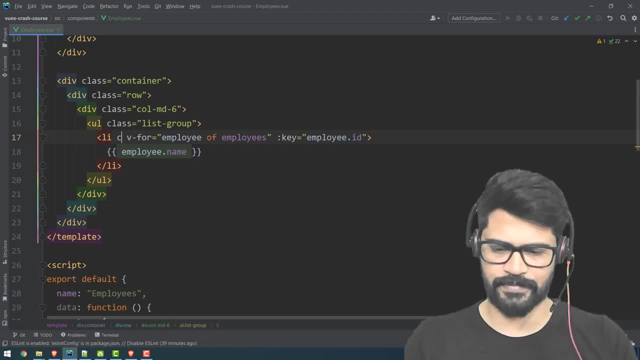 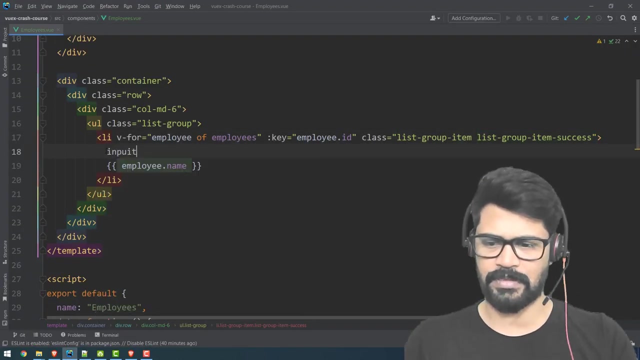 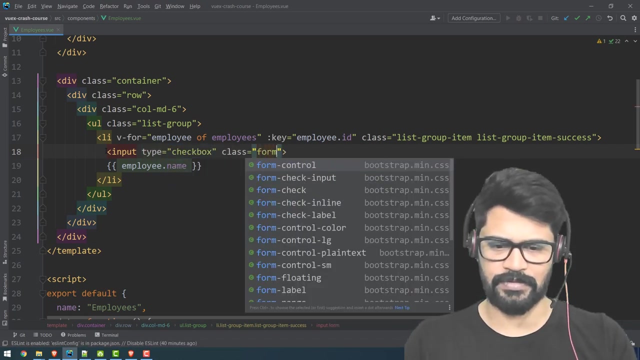 so let's give us classes to say list to group and there's gonna be the let's group and there's gonna be the let's group and there's gonna be the let's group item okay you know have some color group item okay you know have some color group item okay you know have some color I say this group item success okay and I I say this group item success okay and I I say this group item success okay and I also have the check boxes so let's add a also have the check boxes so let's add a also have the check boxes so let's add a check box input type check box and the check box input type check box and the check box input type check box and the class form check from check input it's class form check from check input it's class form check from check input it's all all all 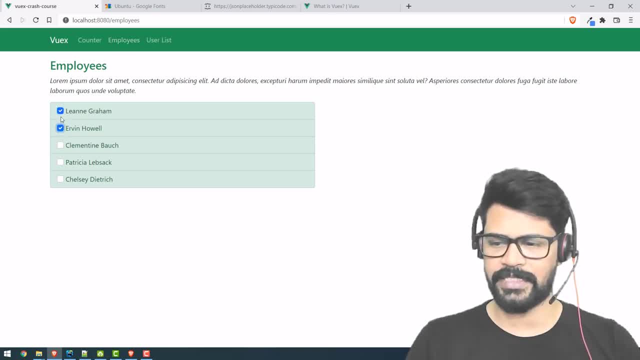 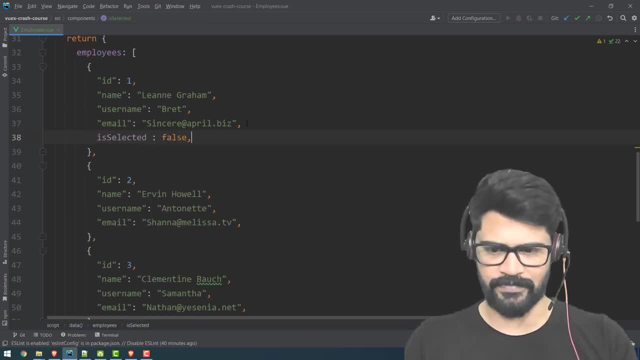 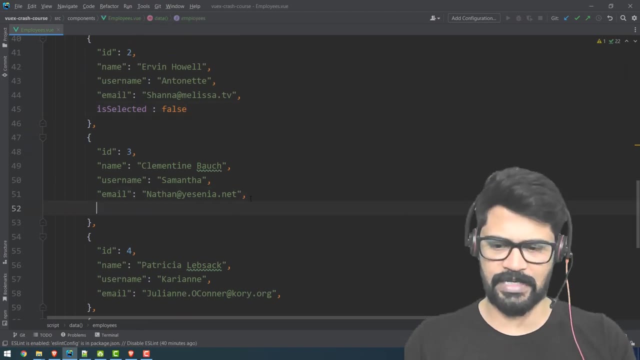 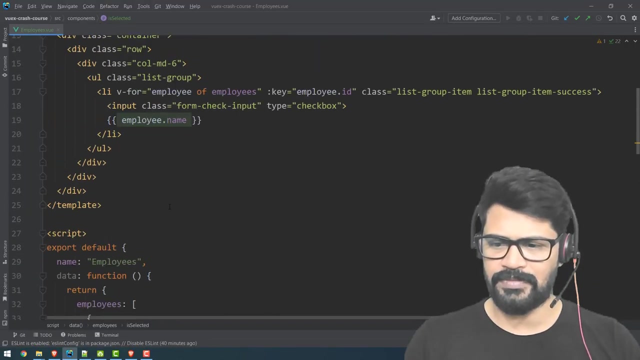 all yep you get the check box for yep you get the check box for yep you get the check box for selecting this data one extra property I selecting this data one extra property I selecting this data one extra property I forgot it is is selected will be false forgot it is is selected will be false forgot it is is selected will be false by default so let's make this guy for by default so let's make this guy for by default so let's make this guy for all you have to make this extra to have all you have to make this extra to have all you have to make this extra to have selected data okay okay fine I have all selected data okay okay fine I have all selected data okay okay fine I have all this now data has been done okay so this now data has been done okay so this now data has been done okay so when I make a selection I need to update this 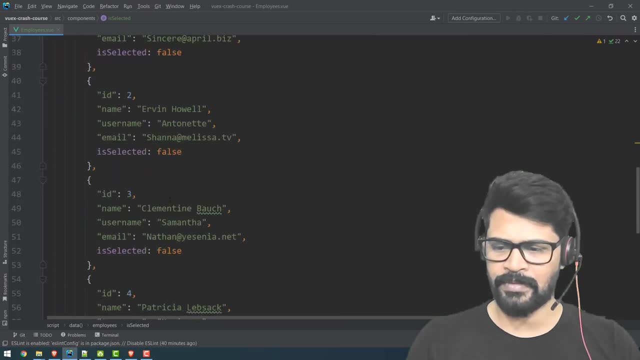 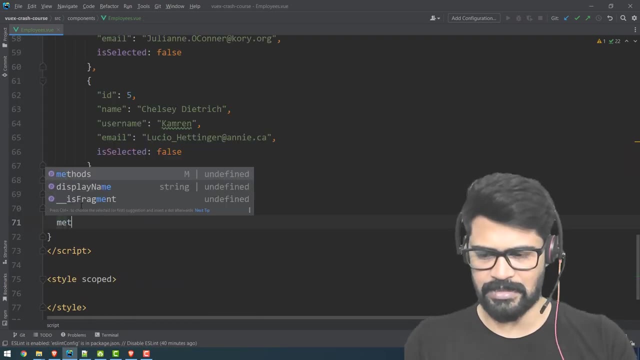 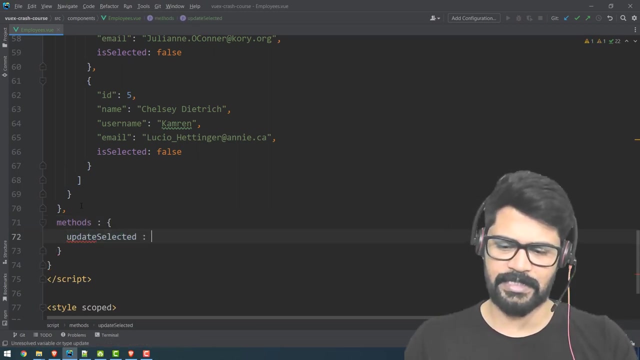 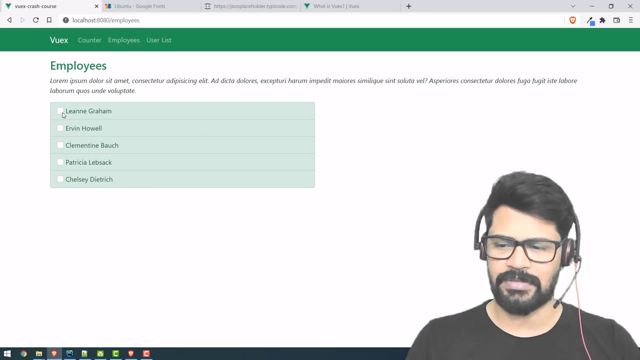 when I make a selection I need to update this when I make a selection I need to update this state so how do I do yeah let me state so how do I do yeah let me state so how do I do yeah let me create a method so where is data close data create a method so where is data close data create a method so where is data close data close here and then they say methods close here and then they say methods close here and then they say methods will be an object where update selected will be an object where update selected will be an object where update selected will be a function okay when you make a will be a function okay when you make a will be a function okay when you make a check for the check box I have to make check for the check box I have to make check for the check box I have to make this guys you selected value to be true this guys you selected value to be true this guys you selected value to be true okay so this okay so this 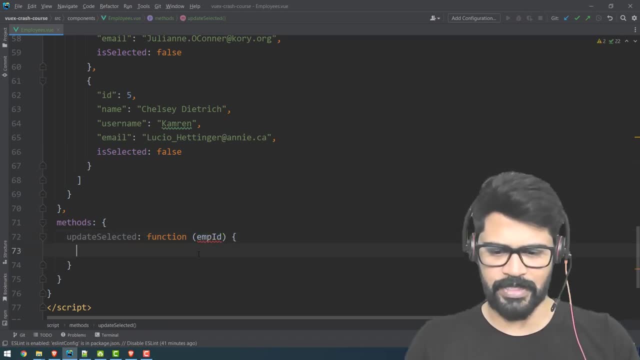 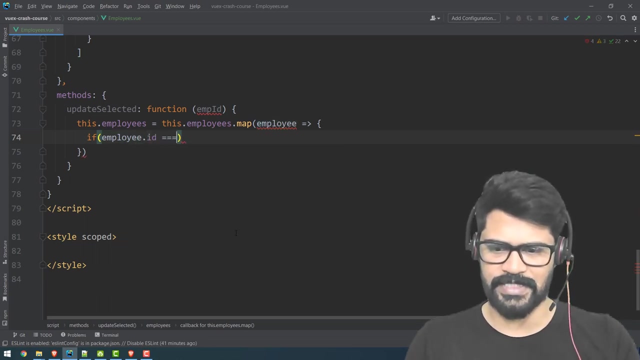 okay so this pass on the employee ID employee ID so what pass on the employee ID employee ID so what pass on the employee ID employee ID so what I do is so I'll say this dot this I do is so I'll say this dot this I do is so I'll say this dot this dot employees is equal to this dot dot employees is equal to this dot dot employees is equal to this dot employees dot map each employee so I'll employees dot map each employee so I'll employees dot map each employee so I'll say if employee dot ID is matched with say if employee dot ID is matched with say if employee dot ID is matched with my employee EMP ID then for that case my employee EMP ID then for that case my employee EMP ID then for that case I return an object where all the 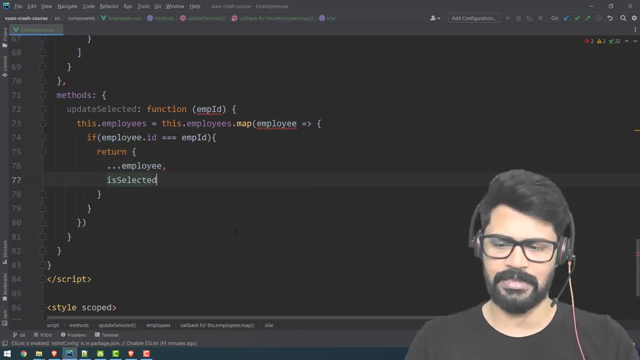 I return an object where all the I return an object where all the employees properties and is selected will employees properties and is selected will employees properties and is selected will be will be not employee dot is be will be not employee dot is be will be not employee dot is selected so opposite to true okay if it selected so opposite to true okay if it selected so opposite to true okay if it is false opposite to false and also if is false opposite to false and also if is false opposite to false and also if else hit an employee as it is unchanged else hit an employee as it is unchanged else hit an employee as it is unchanged okay so I have a function for update okay so I have a function for update okay so I have a function for update selected okay the is letter value so now selected okay the is letter value so now 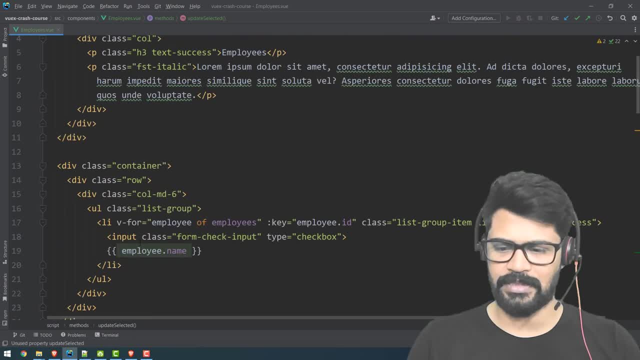 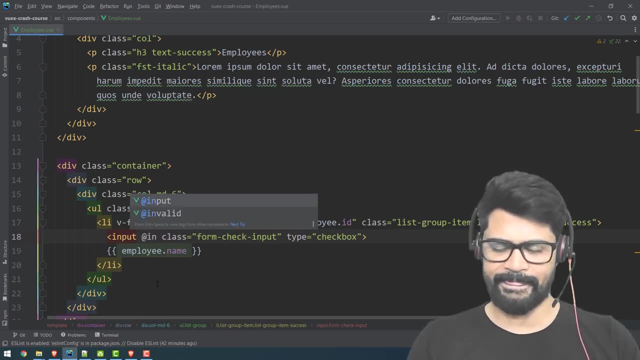 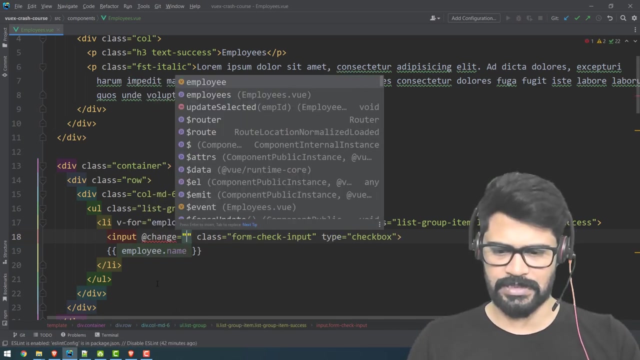 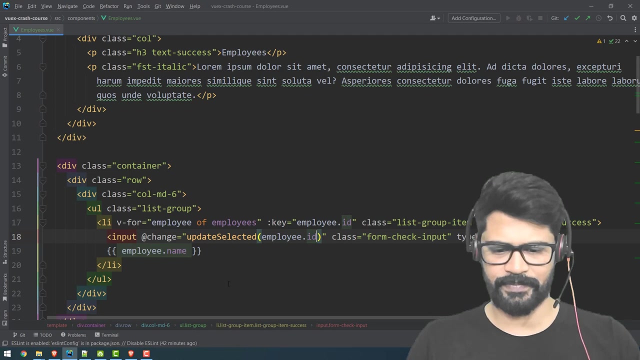 selected okay the is letter value so now I have to connect with my input so I say I have to connect with my input so I say I have to connect with my input so I say here it let's say on change okay on here it let's say on change okay on here it let's say on change okay on change is equal to update selected okay change is equal to update selected okay change is equal to update selected okay is a function which you have to pass is a function which you have to pass is a function which you have to pass employee ID okay I'm passing it but I employee ID okay I'm passing it but I employee ID okay I'm passing it but I have to see the state changes so can we have to see the state changes so can we have to see the state changes so can we write a free write a free write a free tag expression where all the employees you 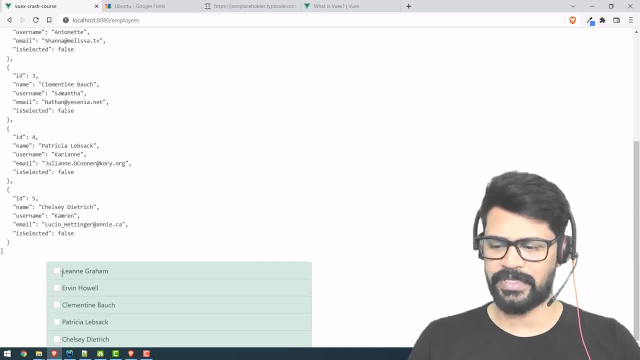 tag expression where all the employees you tag expression where all the employees you have all list of employees so all are have all list of employees so all are have all list of employees so all are this false so when I select for linen 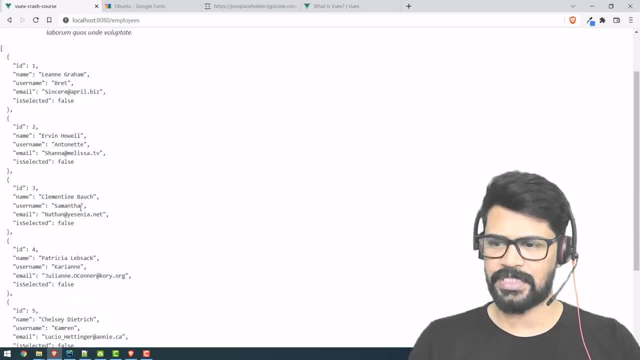 this false so when I select for linen this false so when I select for linen yes it's become true and when I make it yes it's become true and when I make it yes it's become true and when I make it uncheck it's become false yeah perfect uncheck it's become false yeah perfect 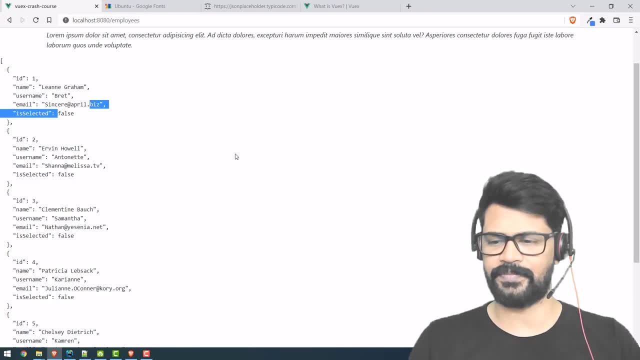 uncheck it's become false yeah perfect so I don't need this now okay so all so I don't need this now okay so all so I don't need this now okay so all selected data I need to describe the selected data I need to describe the selected data I need to describe the right side so this is the first column right side so this is the first column 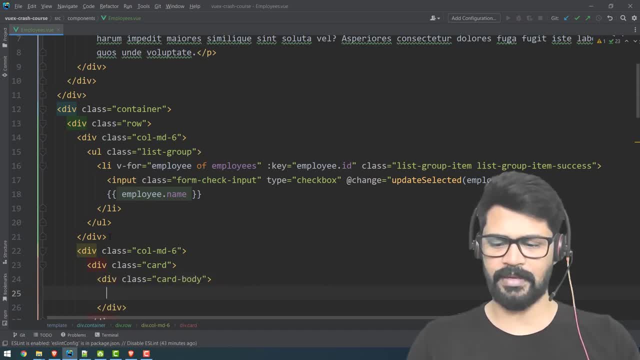 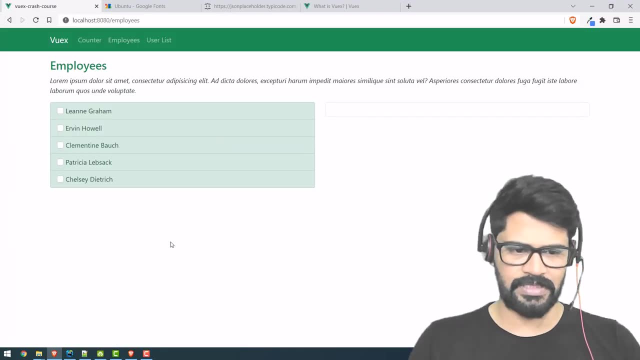 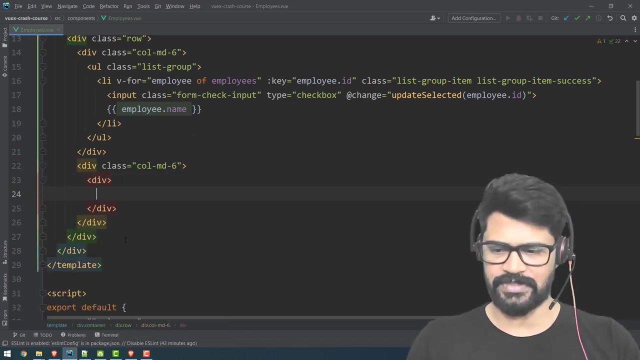 right side so this is the first column with the card body card body and instead with the card body card body and instead with the card body card body and instead of card body okay I'll do one thing I'll of card body okay I'll do one thing I'll of card body okay I'll do one thing I'll just take a division and then card okay just take a division and then card okay just take a division and then card okay how to write multiple cards based on the how to write multiple cards based on the how to write multiple cards based on the selection so you have to light a loop selection so you have to light a loop selection so you have to light a loop through so we for let's know this through so we for let's know this through so we for let's know this employee employee employee and plow is okay employee of 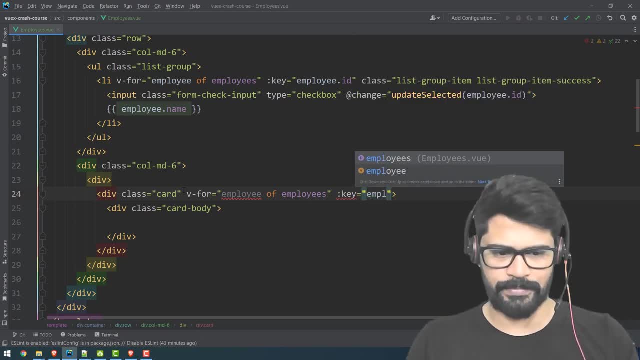 and plow is okay employee of and plow is okay employee of employees and the key will be employee ID okay so 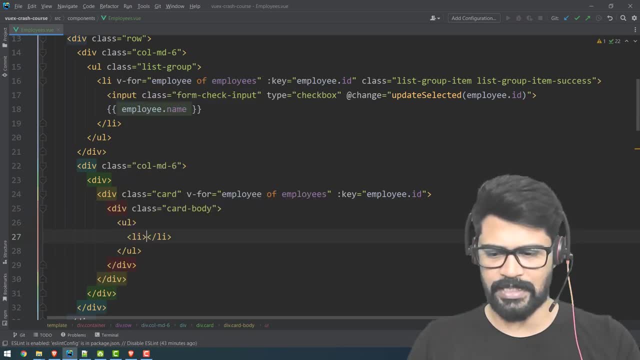 employees and the key will be employee ID okay so employees and the key will be employee ID okay so in this card I'll make a ul Li in this card I'll make a ul Li in this card I'll make a ul Li let's make the name or employee ID can we let's make the name or employee ID can we let's make the name or employee ID can we start with like this some start with like this some start with like this some ID span with the class one with all and ID span with the class one with all and 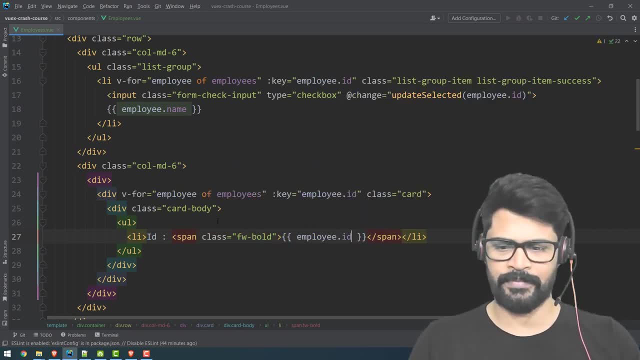 ID span with the class one with all and let's make employee dot ID okay I got let's make employee dot ID okay I got let's make employee dot ID okay I got all IDs yeah let's make for the card all IDs yeah let's make for the card 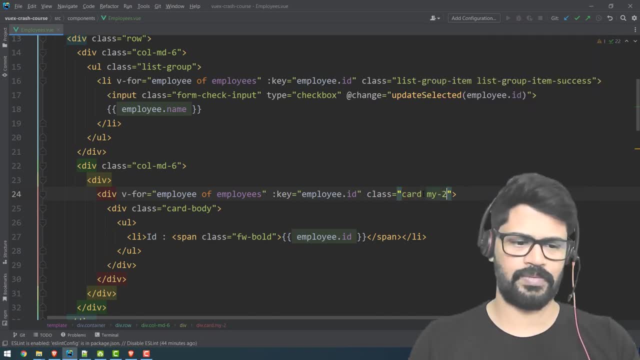 all IDs yeah let's make for the card I'll say some margin top and bottom to I'll say some margin top and bottom to I'll say some margin top and bottom to some space yep card body this group 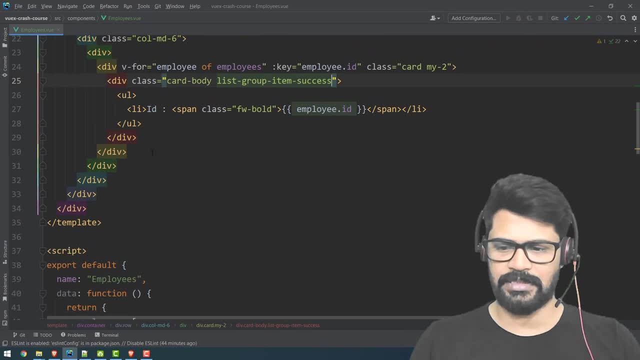 some space yep card body this group some space yep card body this group item success for some color okay that's item success for some color okay that's item success for some color okay that's fine fine 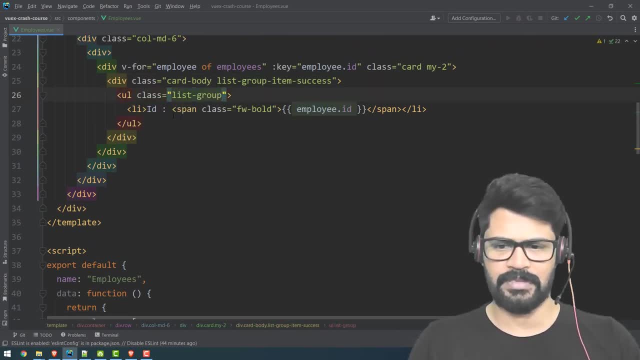 fine this is this this is this this is this group and this one list the group item okay group and this one list the group item okay 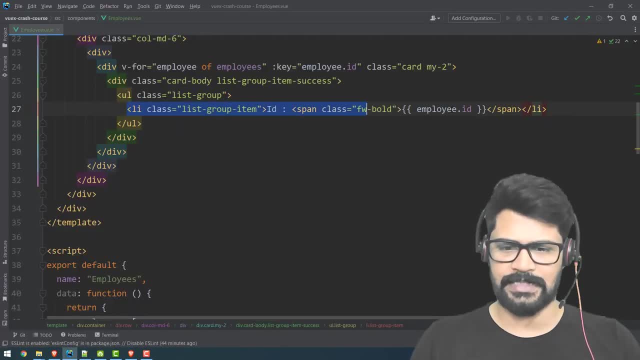 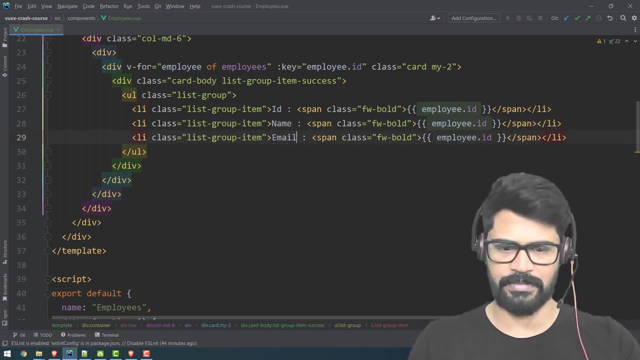 group and this one list the group item okay so I got an ID and same way copy so I got an ID and same way copy so I got an ID and same way copy that so ID name and it's email okay so let's 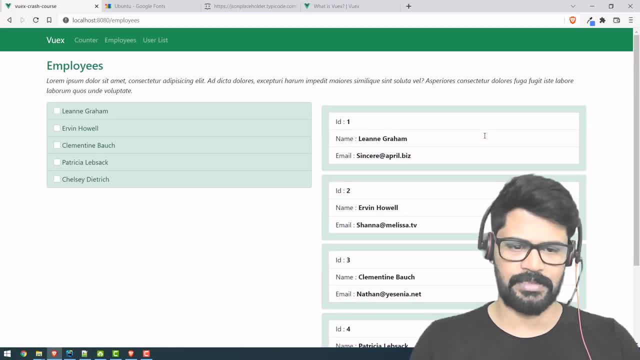 that so ID name and it's email okay so let's that so ID name and it's email okay so let's say the name and this is email okay 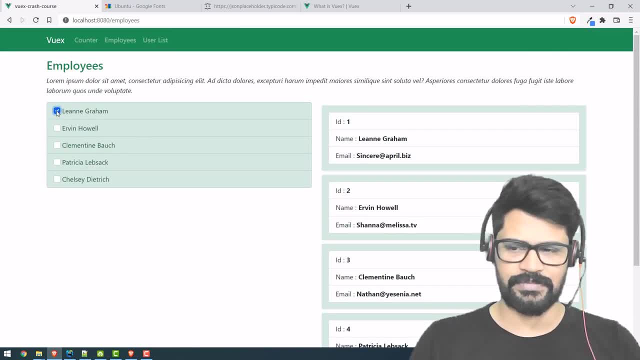 say the name and this is email okay say the name and this is email okay that's fine but I'm getting all the that's fine but I'm getting all the that's fine but I'm getting all the records but I don't need that I just records but I don't need that I just records but I don't need that I just need only the 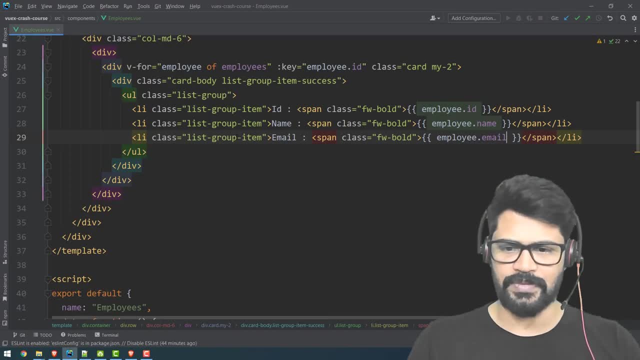 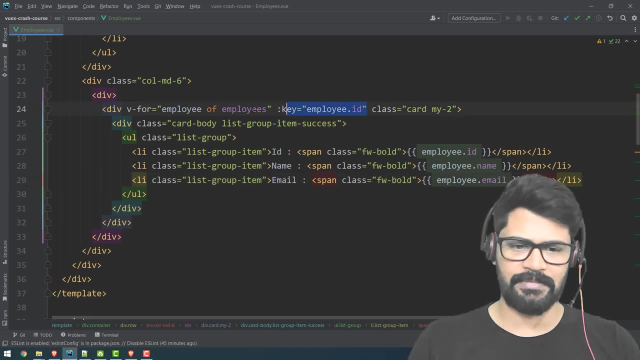 need only the need only the one which was selected so where do I one which was selected so where do I one which was selected so where do I read a condition so for can I do one read a condition so for can I do one read a condition so for can I do one thing can I make a looping for this thing can I make a looping for this 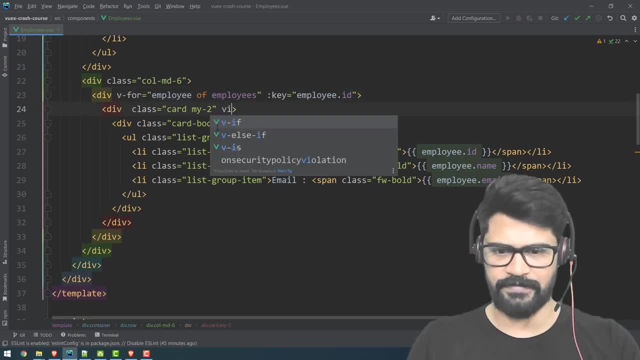 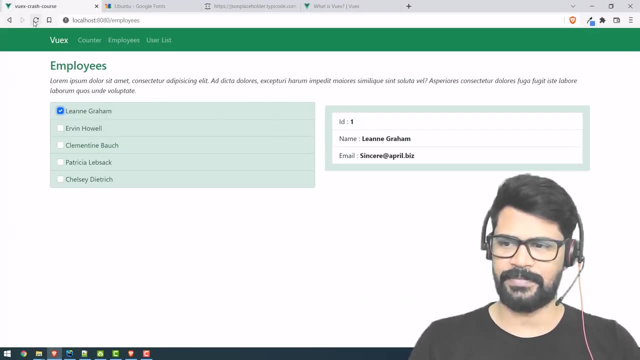 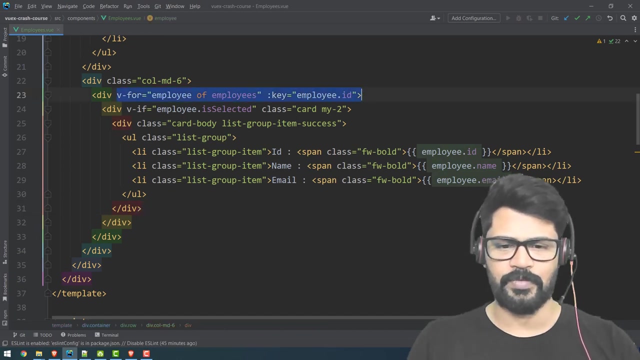 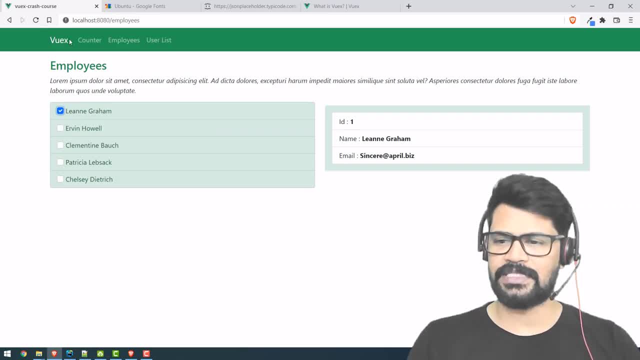 looping here and then if selected for card and all this okay so now this card and all this okay so now this card and all this okay so now this example is perfectly done without view X example is perfectly done without view X example is perfectly done without view X when you make a selection so two people when you make a selection so two people when you make a selection so two people I have selected I got two but when I move I have selected I got two but when I move I have selected I got two but when I move on to use that list and came back this on to use that list and came back this on to use that list and came back this selection was gone because for example selection was gone because for example selection was gone because for example you have some product items and we use you have some product items and we use you have some product items and we use it one product okay if you use it some 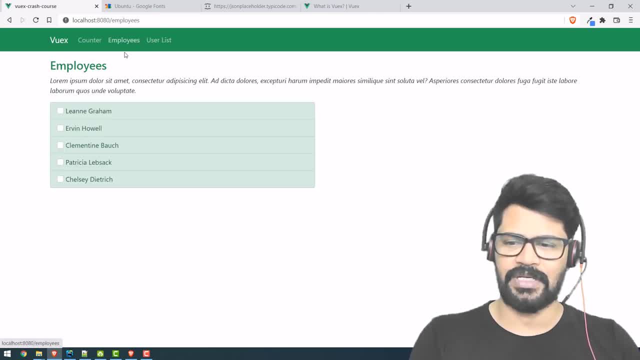 it one product okay if you use it some it one product okay if you use it some few of products and you went to the cart few of products and you went to the cart few of products and you went to the cart page so now the session has gone okay 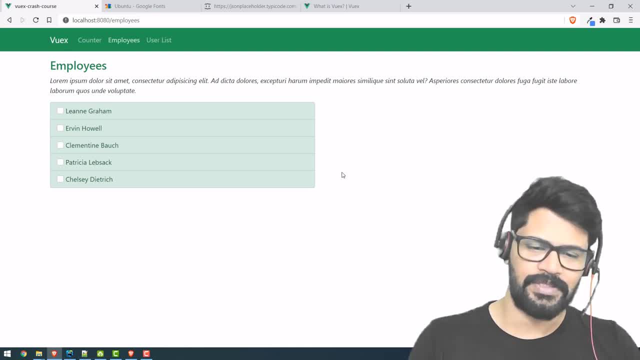 page so now the session has gone okay page so now the session has gone okay so but I have to recite that you have to I so but I have to recite that you have to I so but I have to recite that you have to I have to you know preserve the state have to you know preserve the state 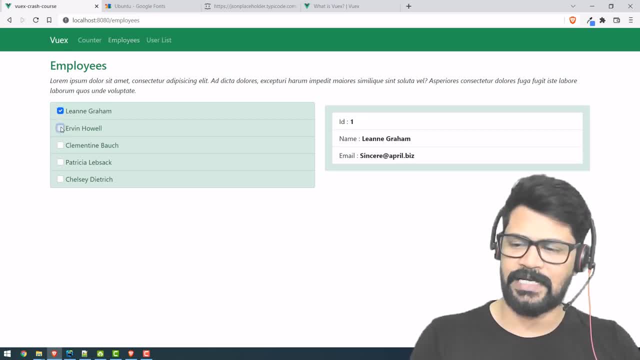 have to you know preserve the state data which you have selected okay so for data which you have selected okay so for data which you have selected okay so for that we must have to move on to the that we must have to move on to the that we must have to move on to the view X so let's convert this example view X so let's convert this example 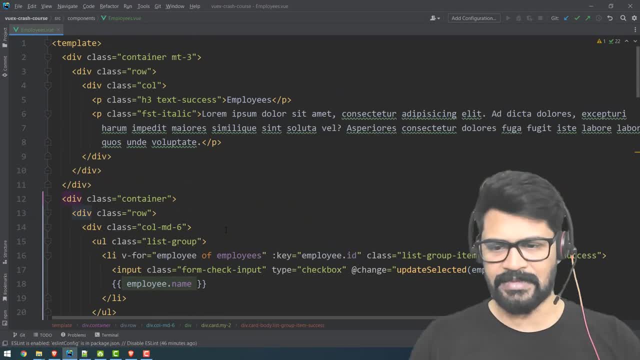 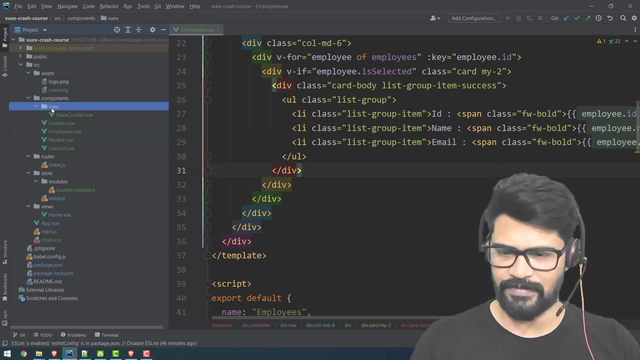 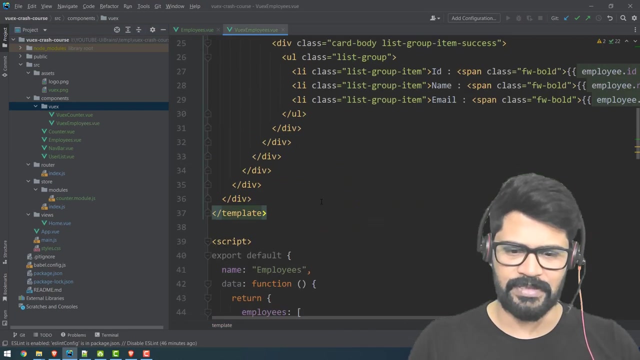 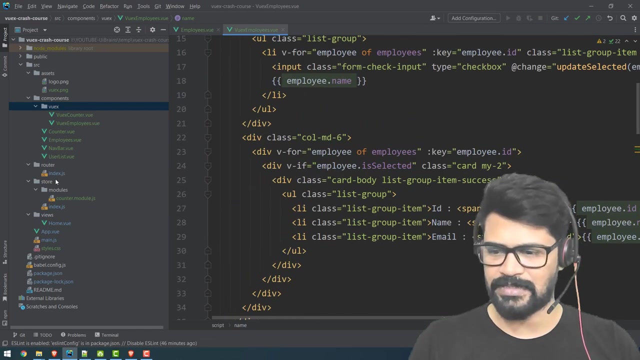 view X so let's convert this example with UX I don't want to touch this with UX I don't want to touch this with UX I don't want to touch this component so I'll make a copy of the component so I'll make a copy of the component so I'll make a copy of the same component in VX folder so let's same component in VX folder so let's same component in VX folder so let's copy employees and the view X I'll paste copy employees and the view X I'll paste copy employees and the view X I'll paste it as a view X dot employee so it will it as a view X dot employee so it will it as a view X dot employee so it will become a view X is the name yeah become a view X is the name yeah become a view X is the name yeah everything is common and let's go to everything is common and let's go to everything is common and let's go to router I'll change this to view X router I'll change this to view X router I'll change this to view X employees okay I just only change the 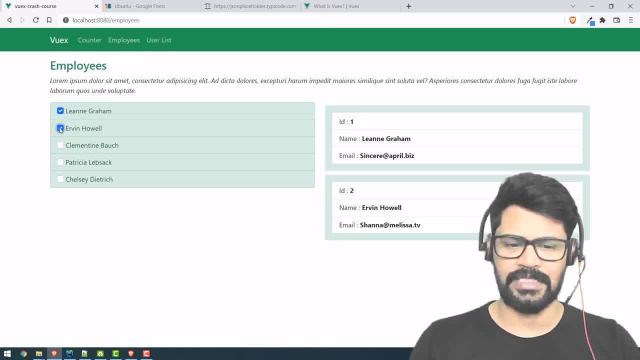 employees okay I just only change the employees okay I just only change the name nothing much still working but data name nothing much still working but data name nothing much still working but data lapse I need to make this lapse I need to make this lapse I need to make this to happen with VX before just start with to happen with VX before just start with to happen with VX before just start with the view X can we do one thing one last 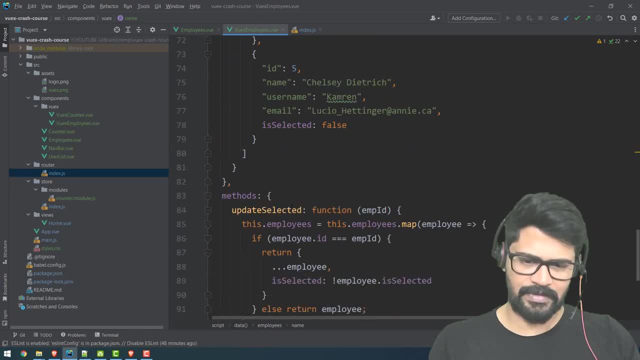 the view X can we do one thing one last the view X can we do one thing one last thing because for employees I don't need thing because for employees I don't need thing because for employees I don't need to have all this data list out here okay 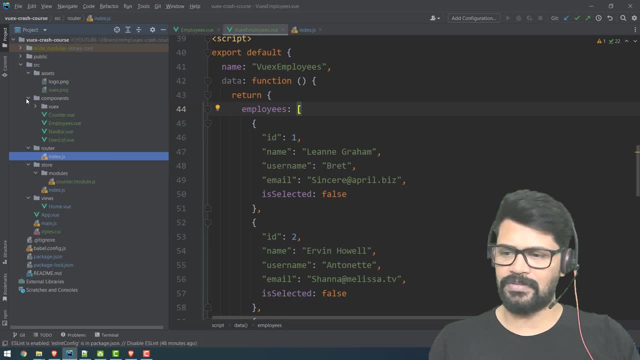 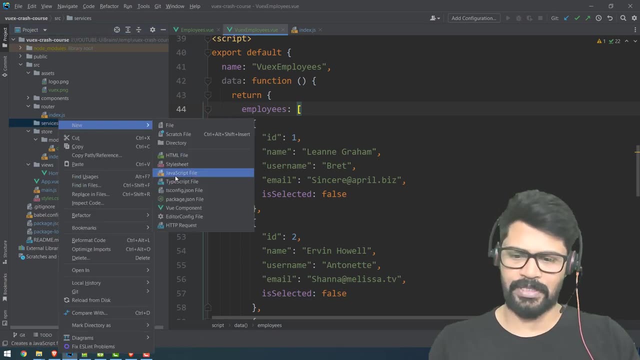 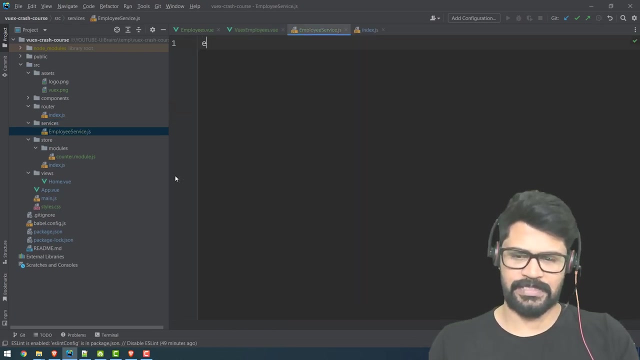 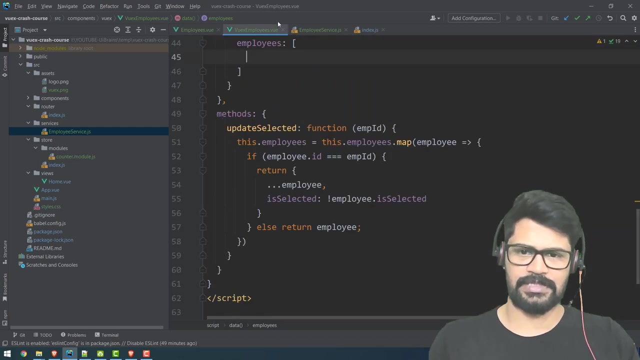 to have all this data list out here okay why can't you create a service for this why can't you create a service for this why can't you create a service for this okay so my plan here is I create one okay so my plan here is I create one okay so my plan here is I create one that recalls services okay I create one that recalls services okay I create one that recalls services okay I create one javascript to say employee employee javascript to say employee employee javascript to say employee employee service so export class employee service service so export class employee service service so export class employee service so here I'll say static employee less is so here I'll say static employee less is so here I'll say static employee less is equal to an array so can we have all equal to an array so can we have all equal to an array so can we have all these employees in this my service okay these employees in this my service okay these employees in this my service okay so can we keep quickly write a function 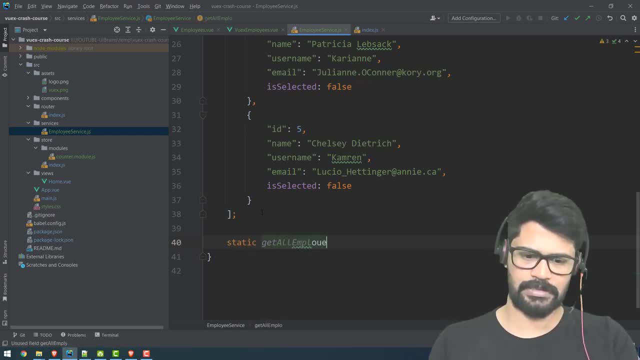 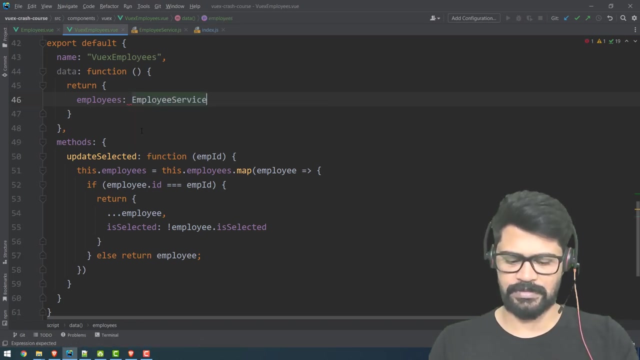 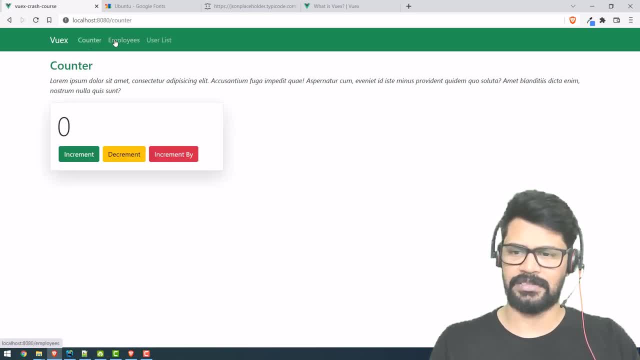 simple line of code which imports service simple line of code which imports service so it's still able to work yeah 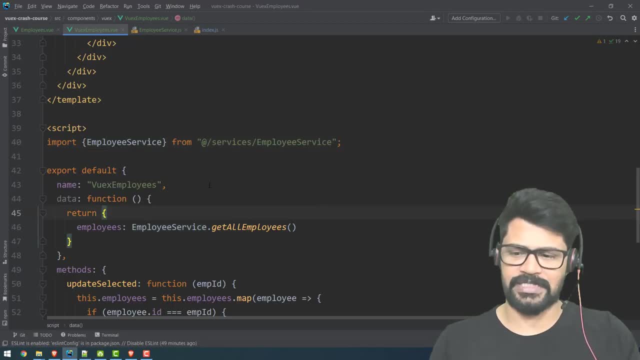 so it's still able to work yeah so it's still able to work yeah I still working that's fine yeah so I still working that's fine yeah so I still working that's fine yeah so now let's convert to VX but now let's convert to VX but now let's convert to VX but when you convert to VX what are the when you convert to VX what are the when you convert to VX what are the things you have to make first thing we 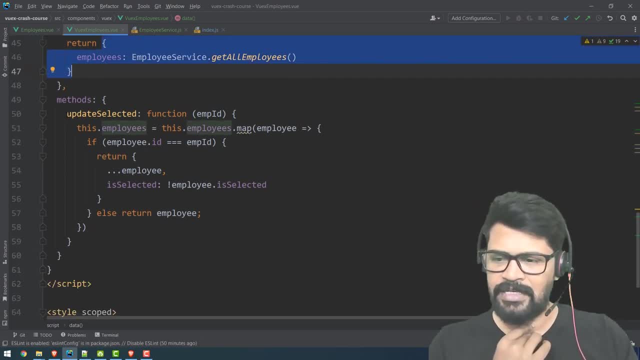 things you have to make first thing we things you have to make first thing we have a data so this data we have to take have a data so this data we have to take have a data so this data we have to take and this methods also we have to take and this methods also we have to take 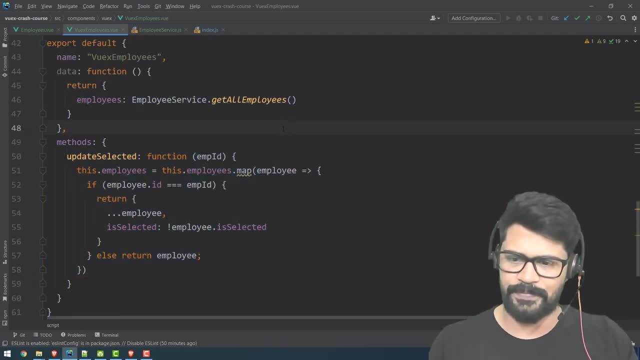 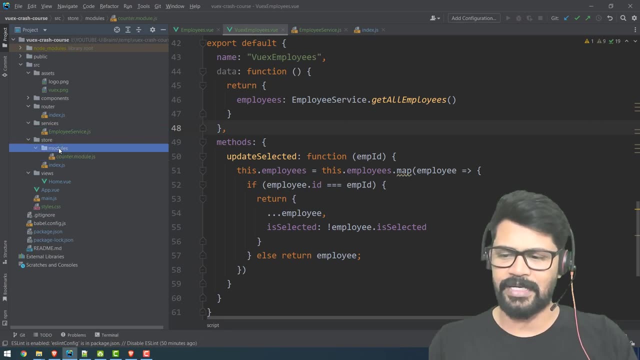 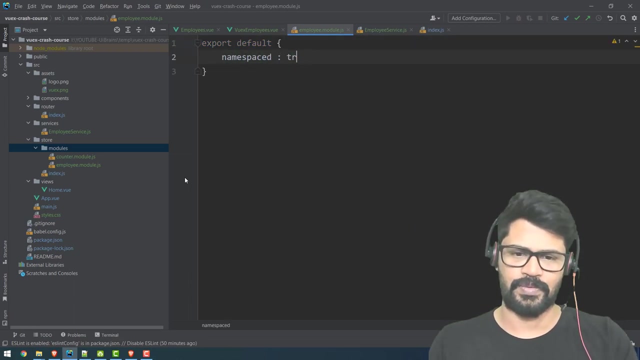 and this methods also we have to take this one method and one state data okay this one method and one state data okay this one method and one state data okay so what you have to do is you create a so what you have to do is you create a so what you have to do is you create a module for counter same like that you module for counter same like that you module for counter same like that you have to create another module so I have to create another module so I have to create another module so I create new JavaScript let's say employee create new JavaScript let's say employee create new JavaScript let's say employee dot module okay so here you write export dot module okay so here you write export dot module okay so here you write export default objects were namespaced is true default objects were namespaced is true default objects were namespaced is true comma you need to write a state and 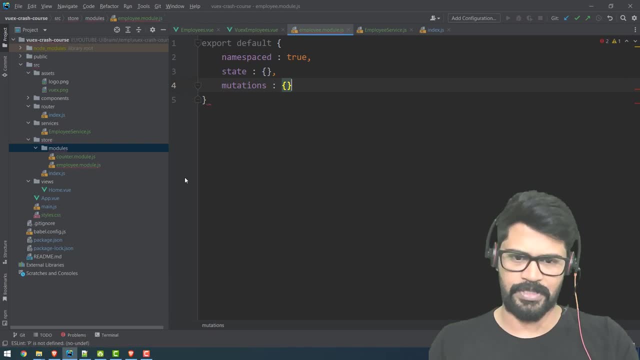 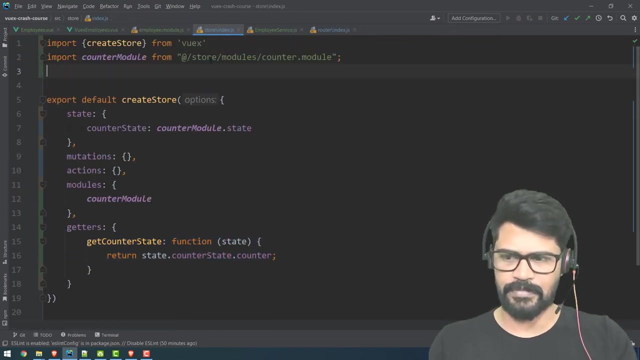 comma you need to write a state and comma you need to write a state and mutations mutations and actions okay so mutations mutations and actions okay so mutations mutations and actions okay so before I proceed with all this lets me before I proceed with all this lets me before I proceed with all this lets me configure configure configure this with my global store so have you this with my global store so have you this with my global store so have you configure import what's that employee configure import what's that employee configure import what's that employee module from my module and let's say module from my module and let's say module from my module and let's say employee state will be employee module employee state will be employee module 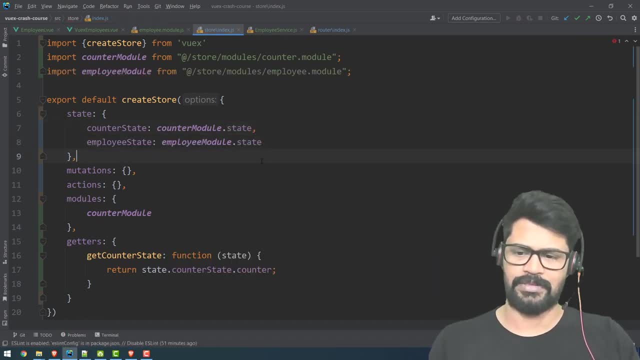 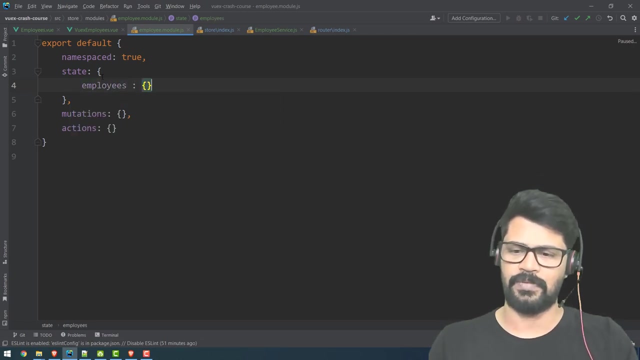 employee state will be employee module dot state okay this will come up okay dot state okay this will come up okay dot state okay this will come up okay and also configure the module here and also configure the module here and also configure the module here employee module okay you have two employee module okay you have two employee module okay you have two modules for two components let's switch to modules for two components let's switch to modules for two components let's switch to employee module yeah so what is your employee module yeah so what is your employee module yeah so what is your stator state will be employees where stator state will be employees where 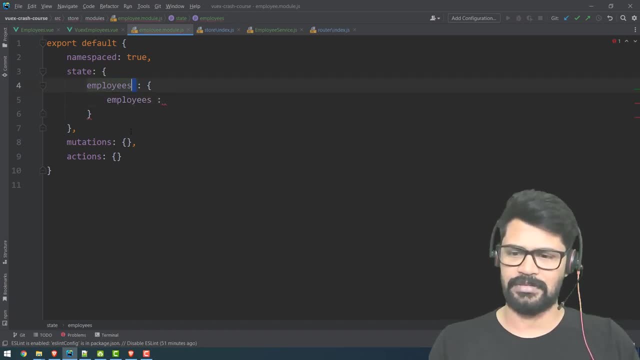 stator state will be employees where employees this just take you know for employees this just take you know for employees this just take you know for our country's an employee employee list our country's an employee employee list our country's an employee employee list you take okay employees will be 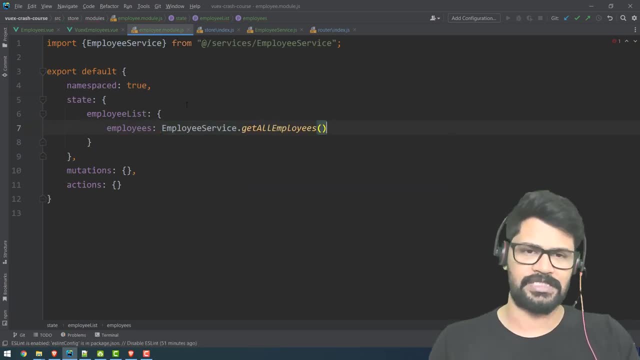 you take okay employees will be you take okay employees will be employee service dot get all employee this is employee service dot get all employee this is employee service dot get all employee this is your initial state right because it's a your initial state right because it's a your initial state right because it's a local data so I just brought it from the local data so I just brought it from the local data so I just brought it from the local service okay this become your local service okay this become your 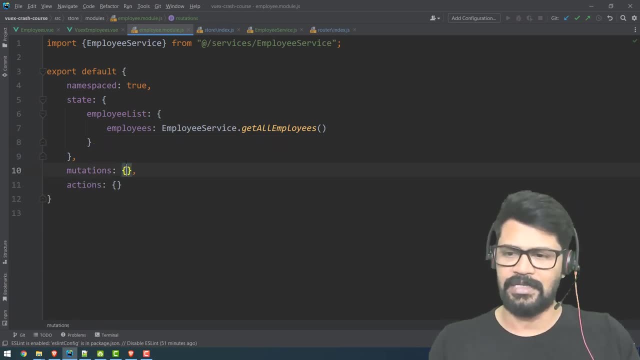 local service okay this become your stator now for mutations what are the stator now for mutations what are the stator now for mutations what are the changes we are doing here update changes we are doing here update 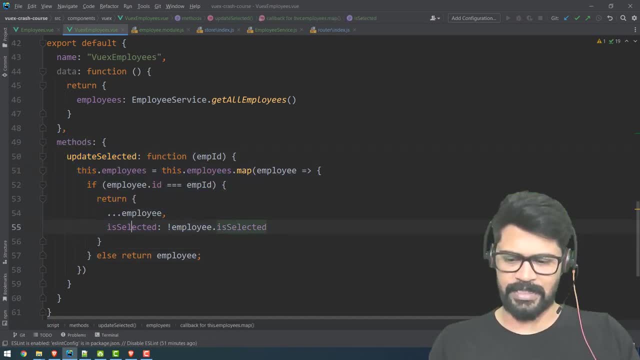 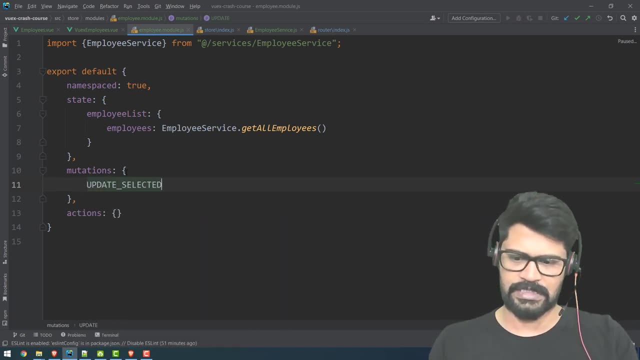 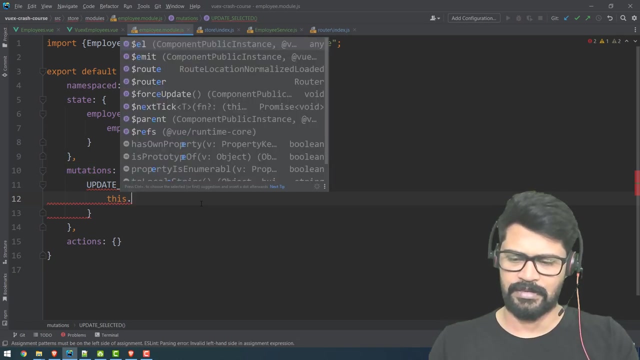 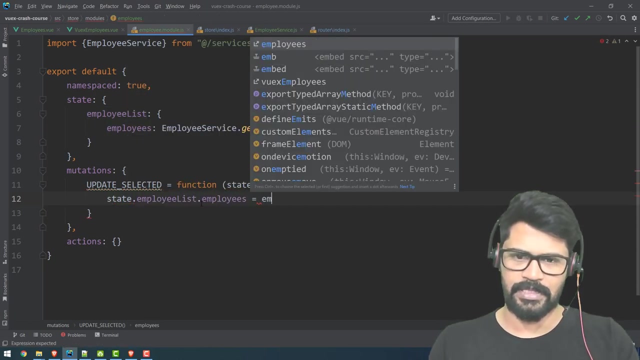 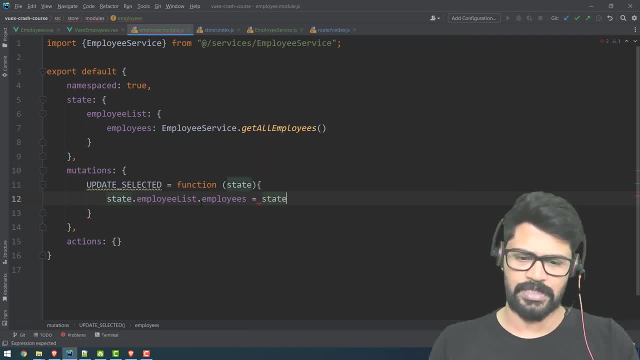 list dot employees is equal to again employee or state dot and playlist dot employee or state dot and playlist dot employee or state dot and playlist dot employees dot map each employee so the employees dot map each employee so the 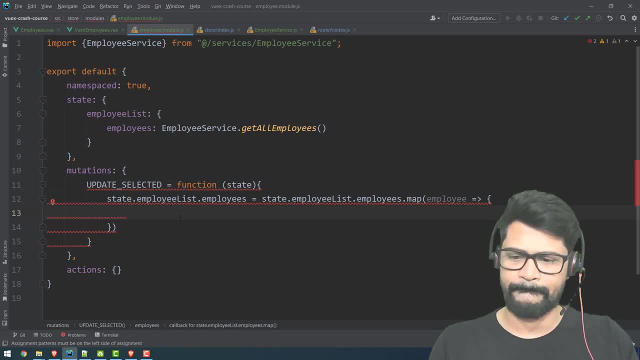 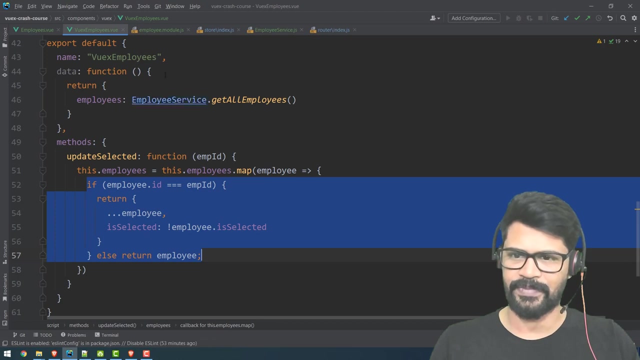 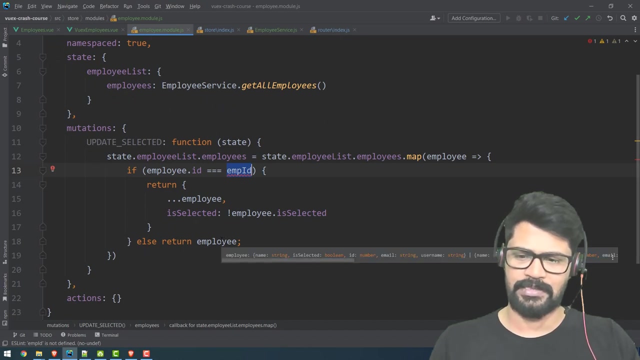 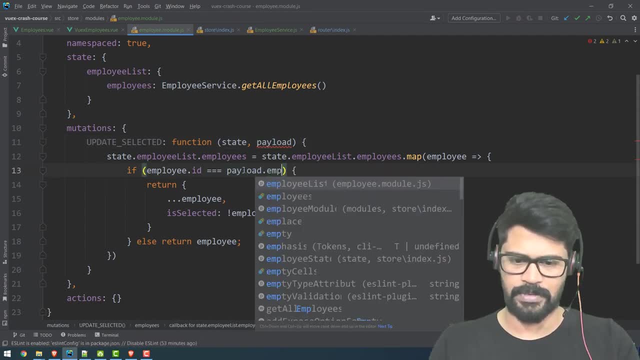 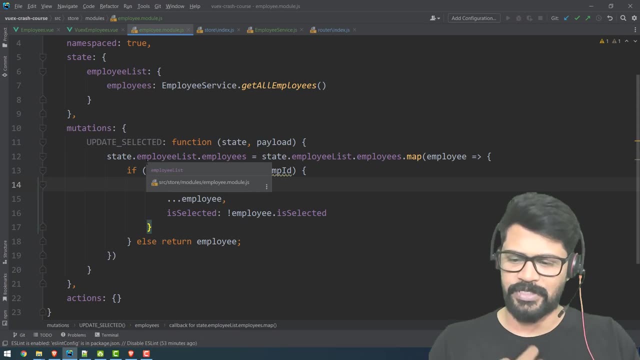 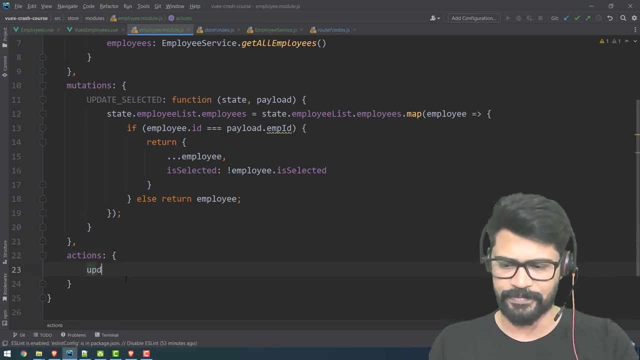 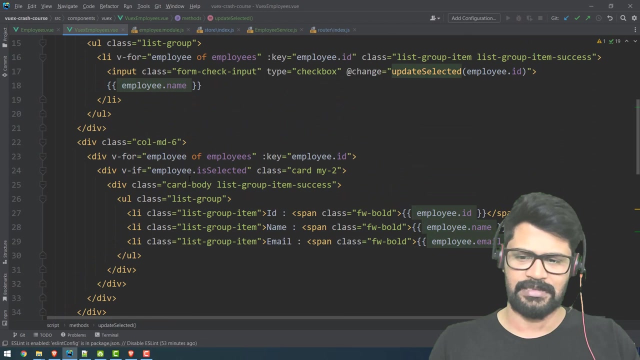 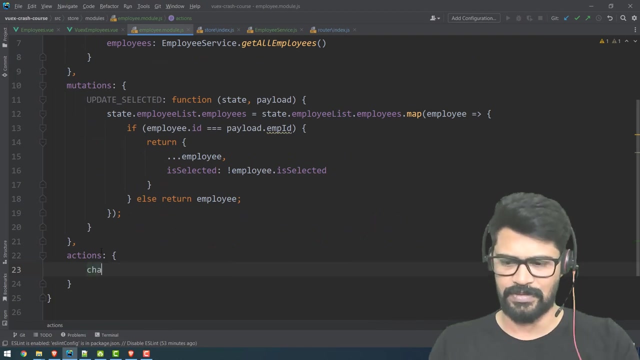 so how we get the payload payload employee ID and make sure while passing payload you pass an object employee okay fine so mutation ready correct mutations ready let's make action so I say update selected but here also update selected and the in the component also we have update selected right update selected so can we change once instead of update selected I'll say or can we change here only okay change update selected see in the place selected okay okay chain selected okay is one function okay this is my action 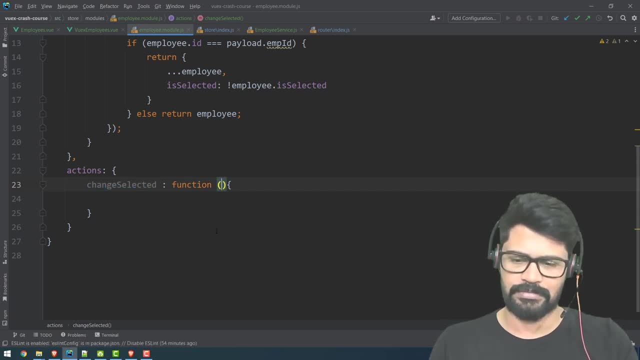 selected so what you have to do is you have to provide what the commit and also the payload 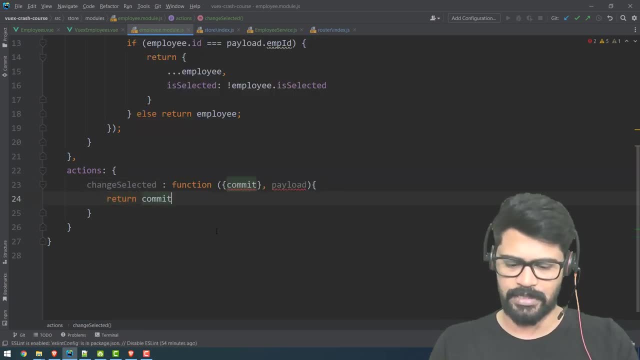 okay so here i write and i commit the update selected provided my payload that's all 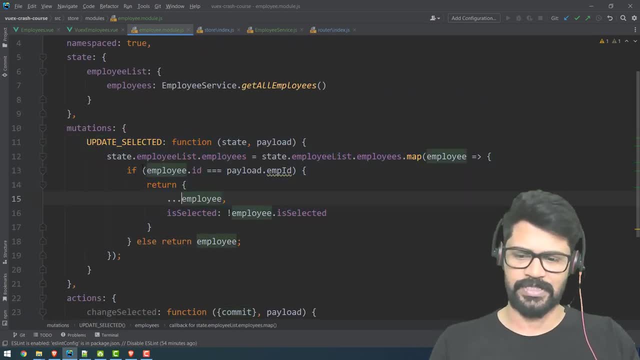 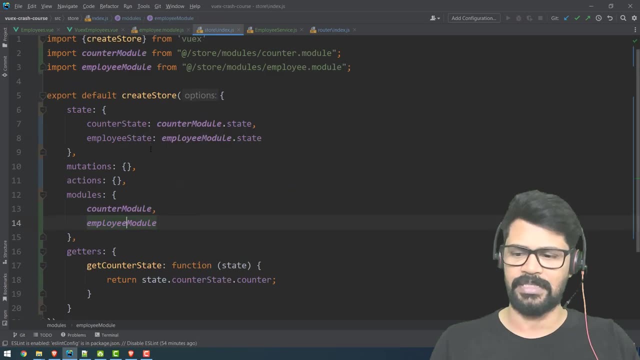 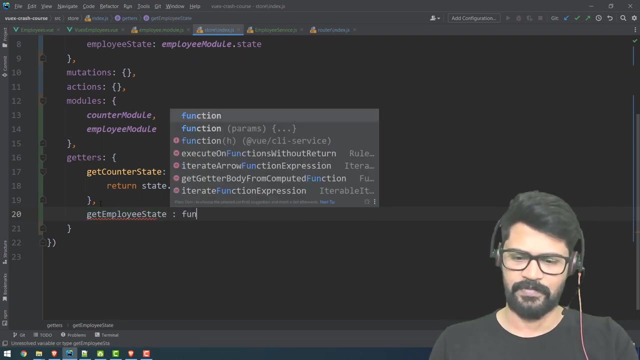 okay so action is committing the mutation the mutation is changing the state and this state i have to access how you access your data getter on the global so same like this comma get employee state will be a function which have access to the state 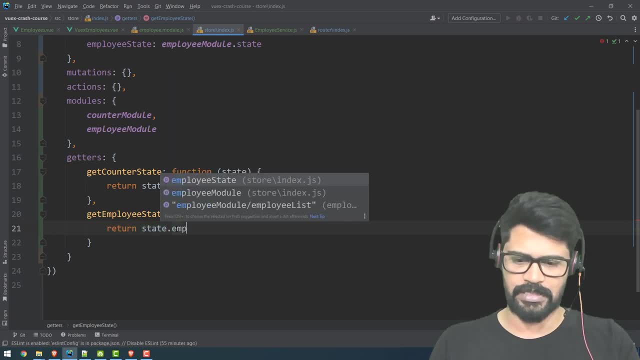 so i return state dot employee state dot employee list okay this particular data i'm going to return 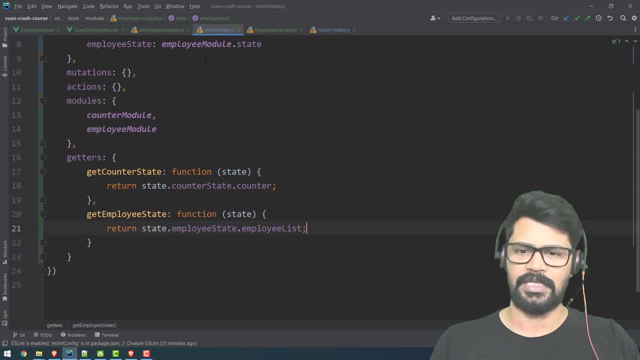 okay so what do i do so i'm going to get the module ready and get ready now jump into view x 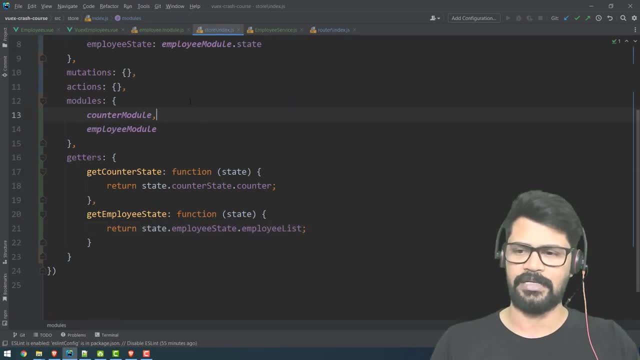 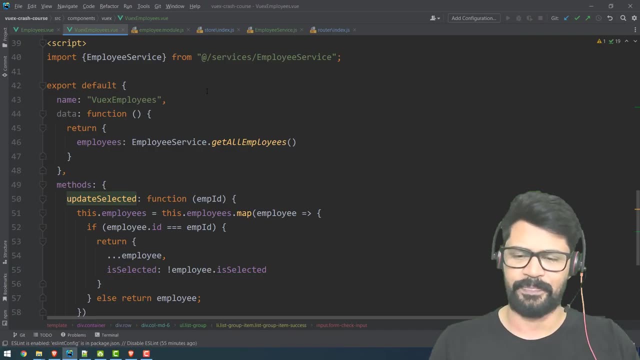 yep so first of all i make sure i don't have any error yep and you can check the configuration also 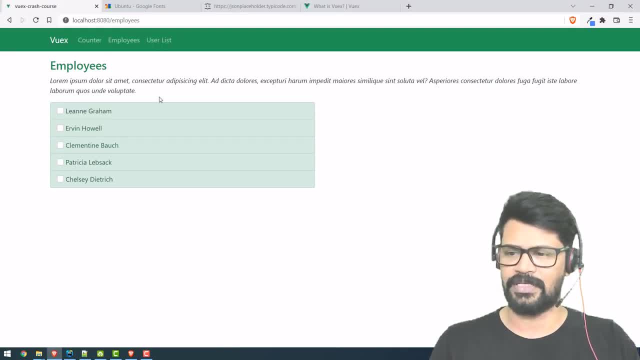 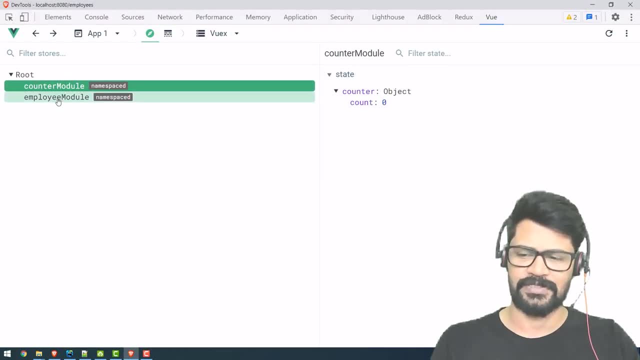 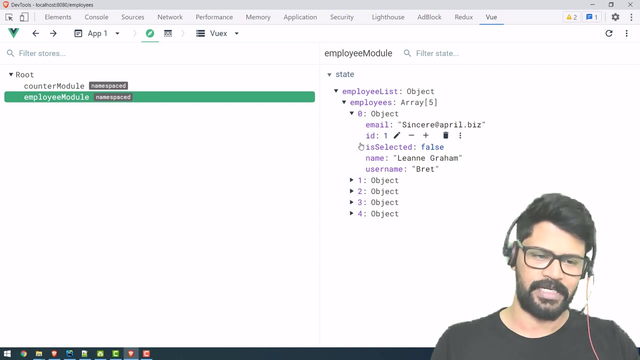 you go to here see two modules has configured now counter module have this and employee module have the array of five objects all the data okay so fine state configuration is done successfully 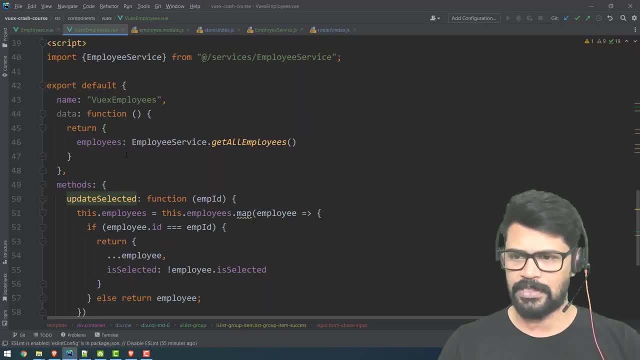 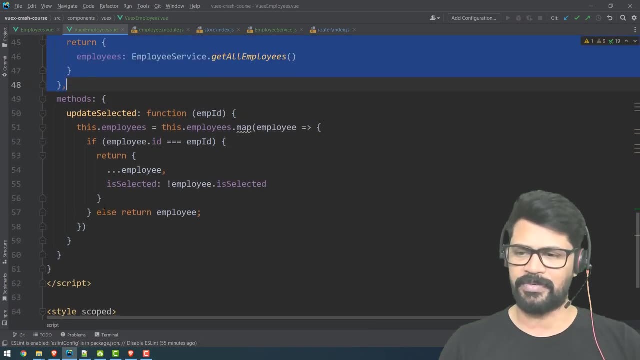 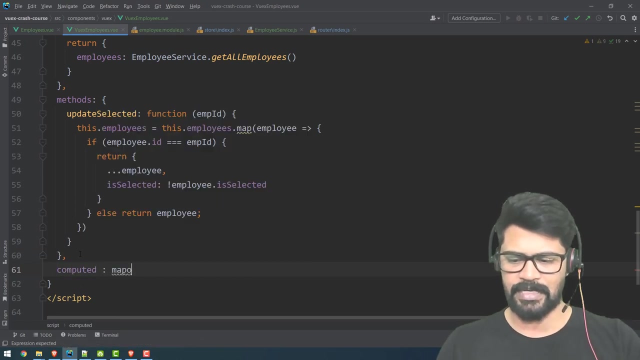 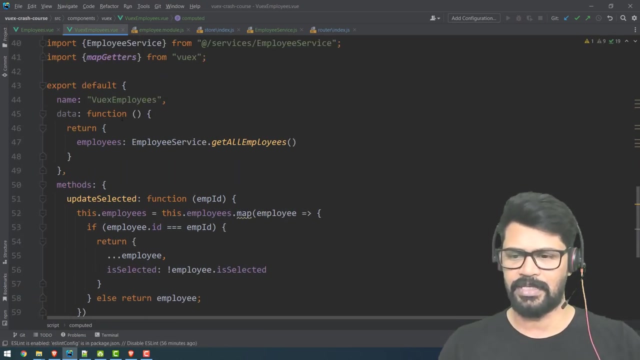 next in the component first of all data i don't need actually data i can get the data from the store with a property called computed so let's say computed will be map map the getters uh import from ux okay import from what is imported yeah map getter from ux 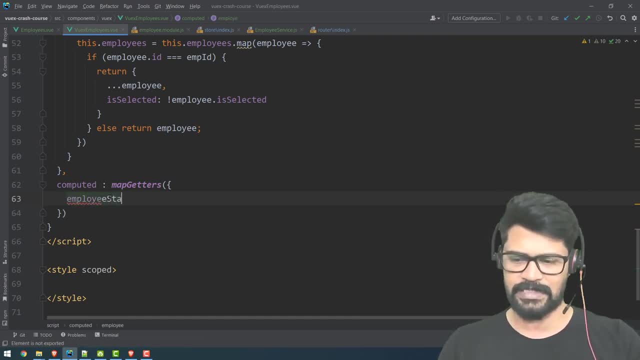 here i say just employee state one second 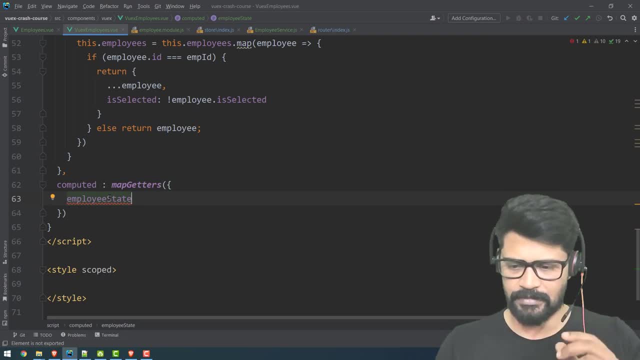 yeah employee state employee state is get employee state that's all simple yeah so this employee state from here you can access 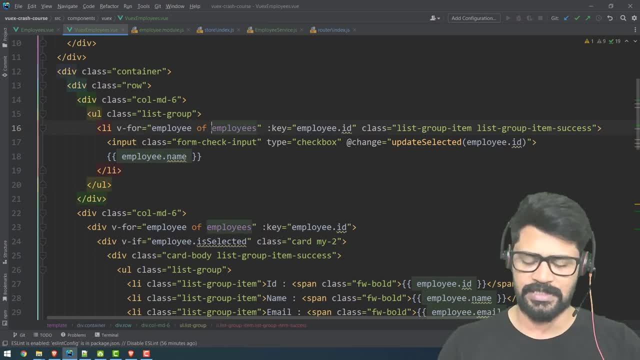 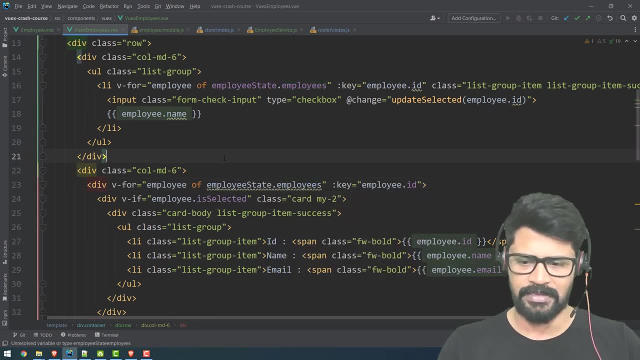 everything so what you have to loop is it's not just employees employee state dot employees correct here also employee state dot employees okay i hope that's fine you check 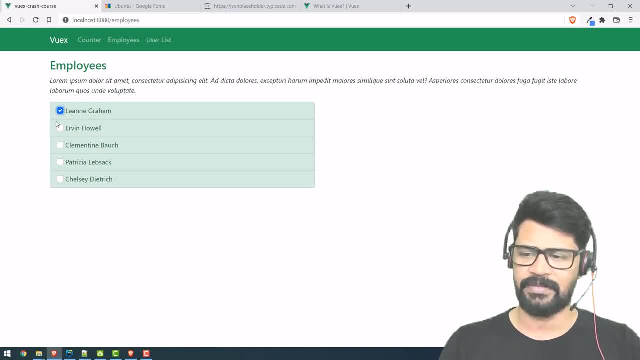 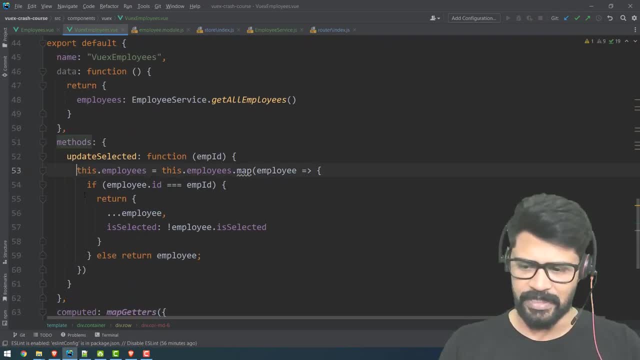 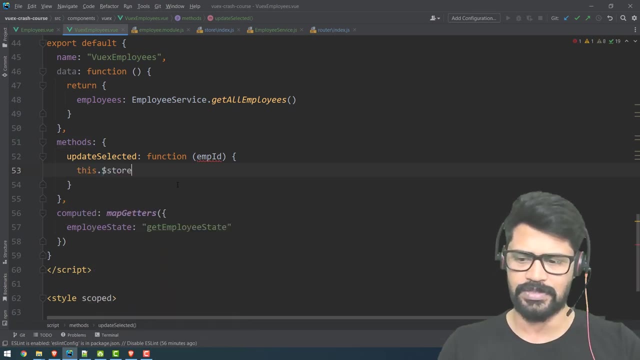 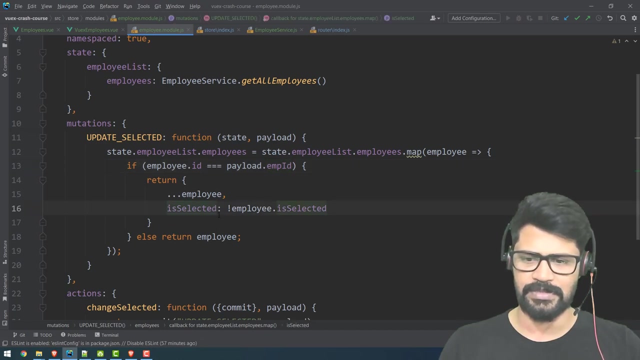 yes we can able to get the data but when i make a selection i'm not getting the updated value because when you make the selection it was updating locally i don't need that i need to update in the global store so this dot dollar store dispatch the action what you have to pass action is employee module dot chain selected and the payload will be what was that employee id is my implied okay it should be an object taking employee id and this employee object taken as a payload and here payload from payload i can get employee and this all this story happens okay so 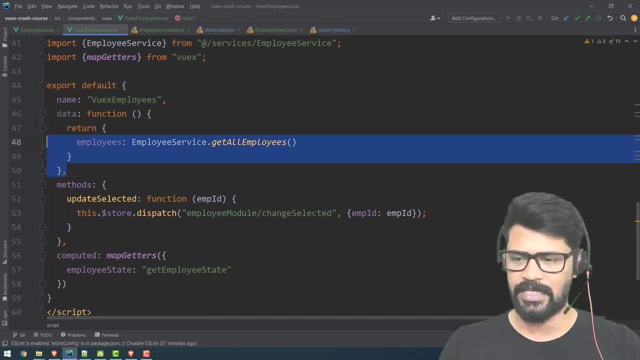 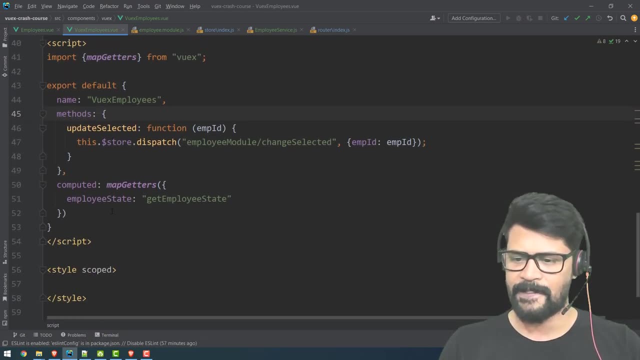 i think that's it yes we have done with this and i don't need data property anymore okay no service nothing yeah see no local state only thing is getting from the store and updating to store it's getting from store and updating so 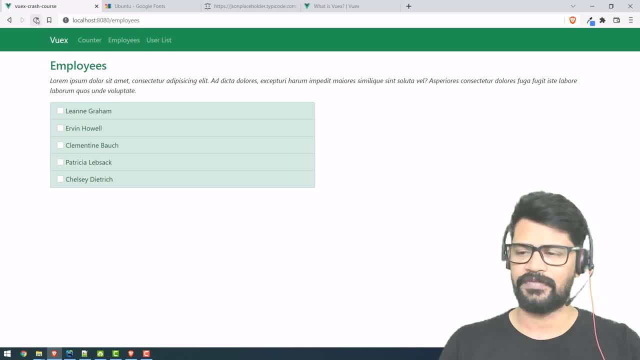 yeah now let's check it's been successful refresh yeah so here employees i select lenin and erwin so 2 date is 2.5. 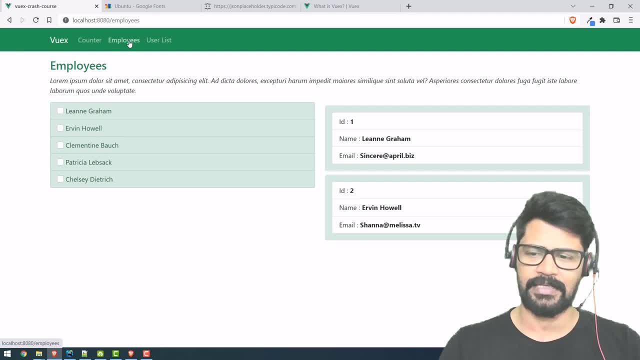 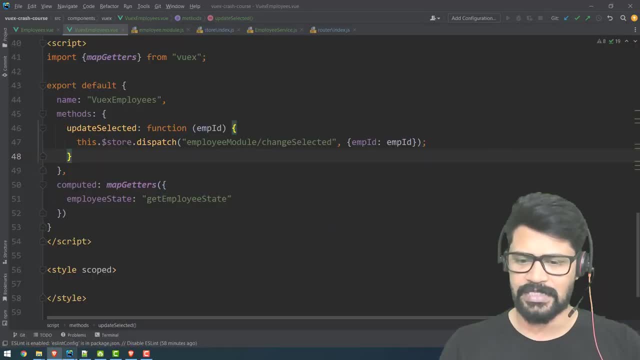 has been selected i went to user list and came back see data still there uh one problem which is the selected has gone selected how you do for input yeah so colon checker is equal to 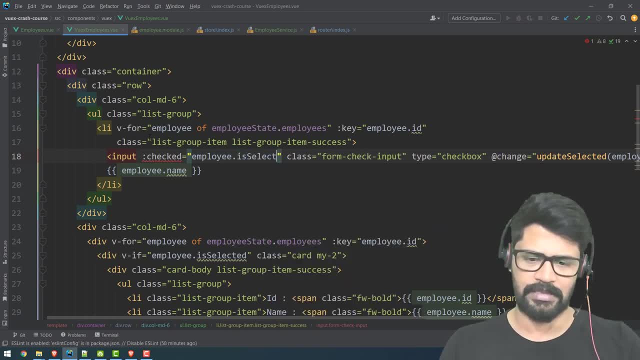 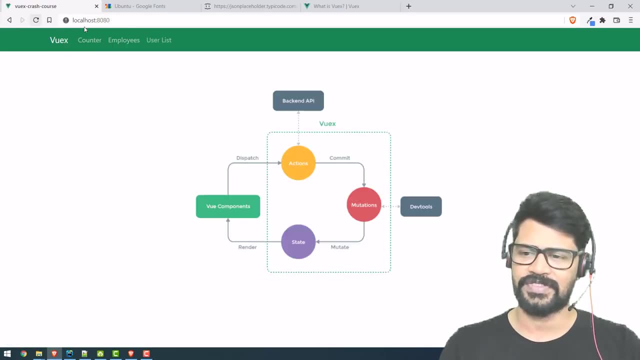 employee dot is selected value okay that's all she's there okay you wanna see refresh if we go to employees i select the two people 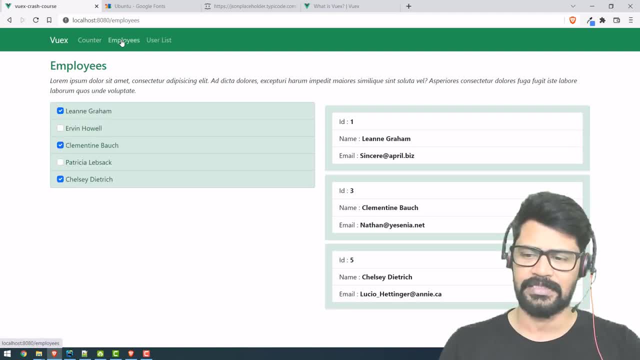 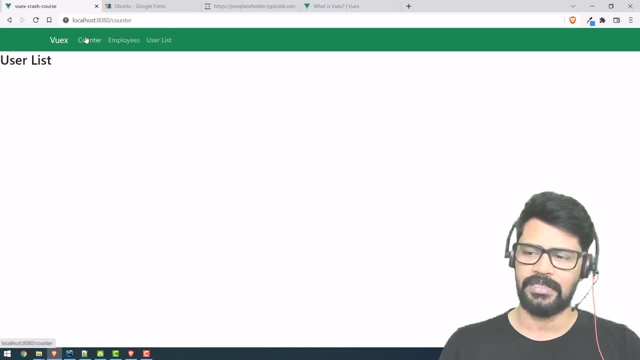 see one three five i selected i went to counter and came back still there i go to counter incremented or decremented go here came back still there and employees also still there 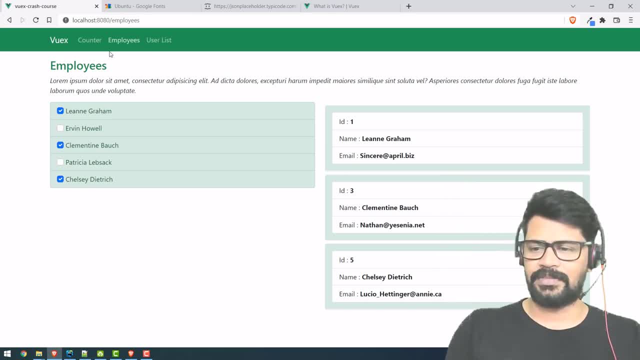 okay all right so we successfully done with uh these two components converted to ux and now let's start with the user 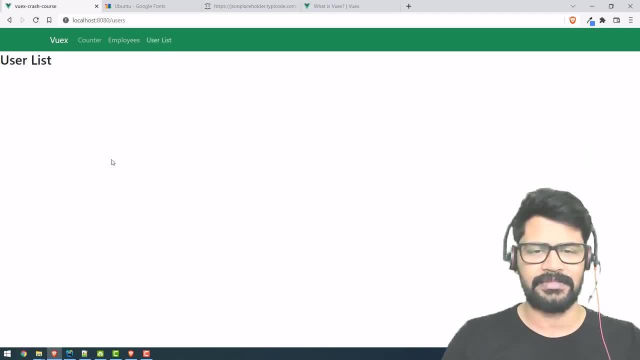 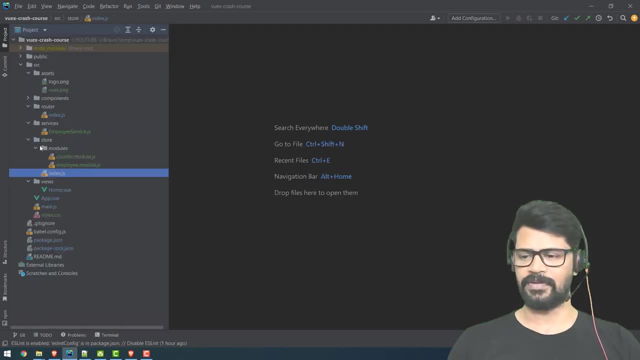 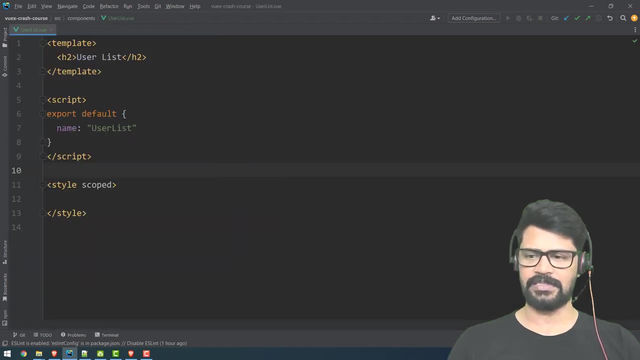 list so user list will make it a default uh data i mean local state management and we'll convert so let's start with user list so let me close all the components yep go to components user list so let's make the setup here with uh now as of now local data okay 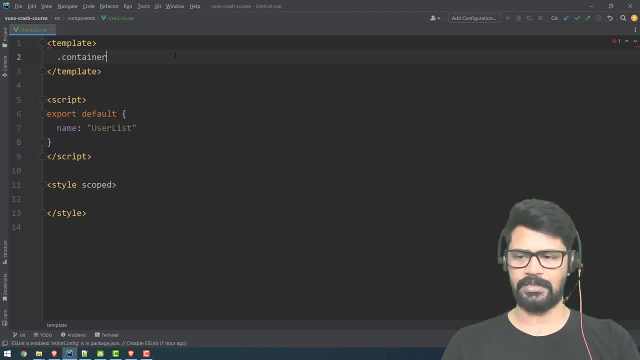 so what you do is um yeah one container one row single column p dot head three um user list so i say texture success and then a paragraph lorem 30 tab 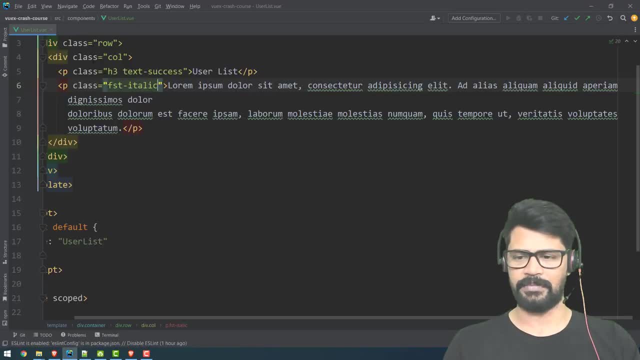 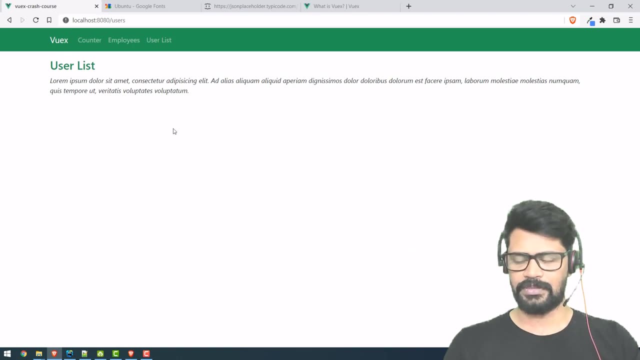 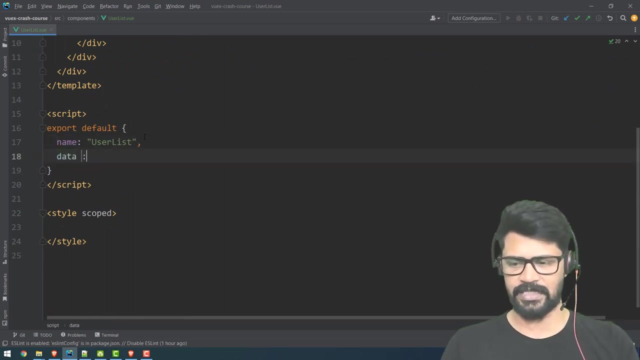 okay and let me get a class called font start italic yep and also make some margin top three okay so under that i have to fetch data from server so so that i can create a state so first data is 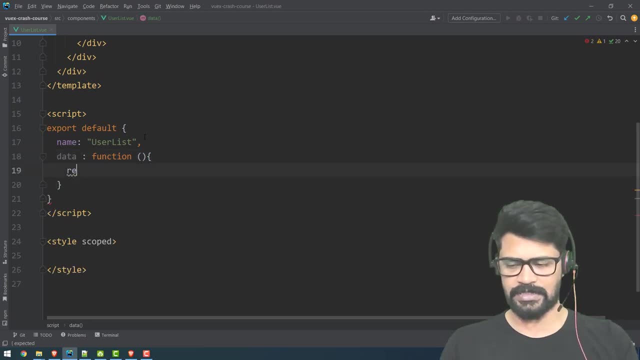 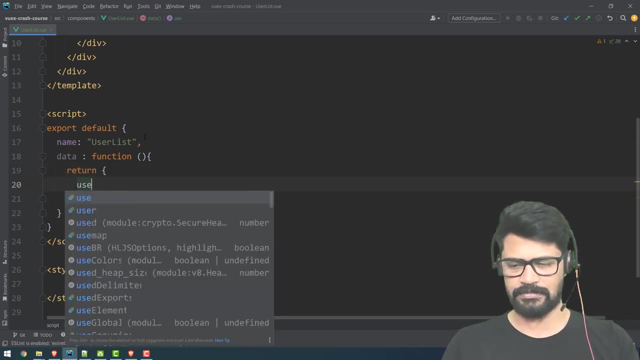 actually a function so this function returns this function written the state but is used uh what you do 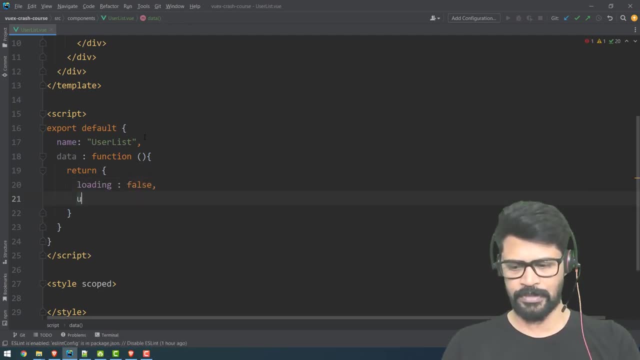 loading is false users will be mtra and error message 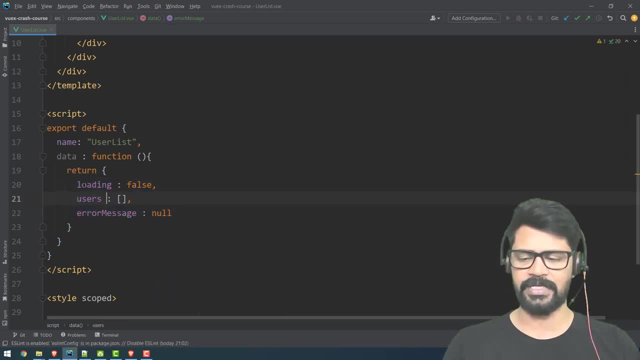 now okay so i have this my state because loading to have you know loading spinner before you fetch data from server and this is actually data from server and this is the error message and so let's make the function call created because 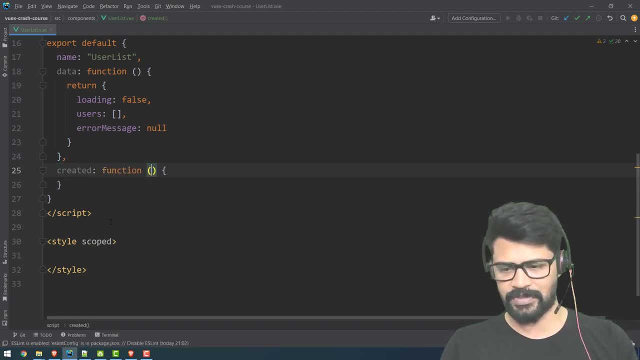 when actually the component has been created I have to make a server call so 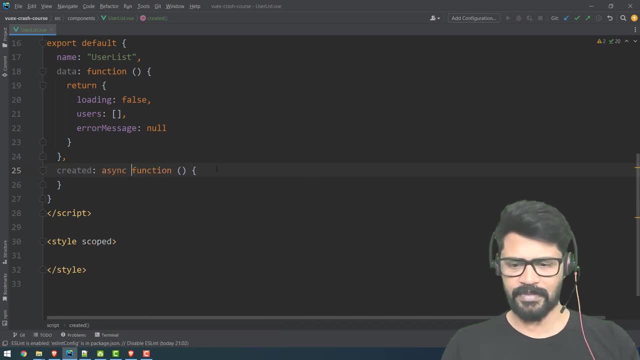 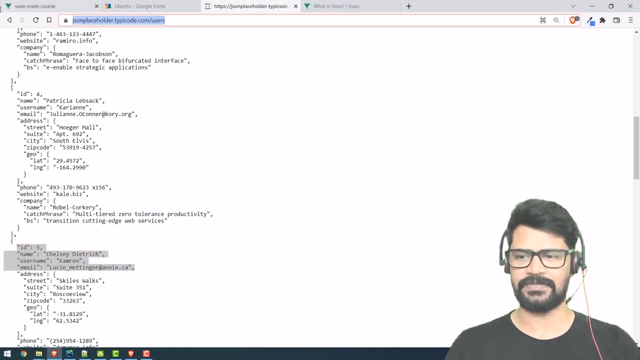 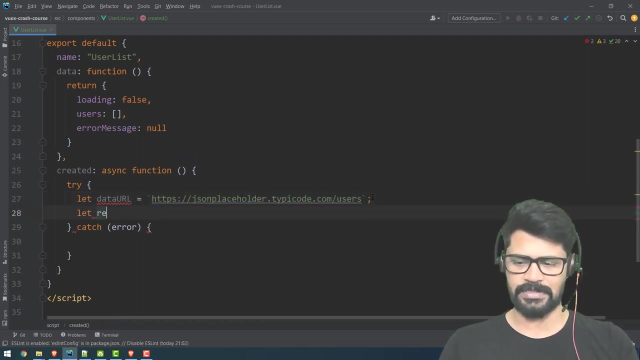 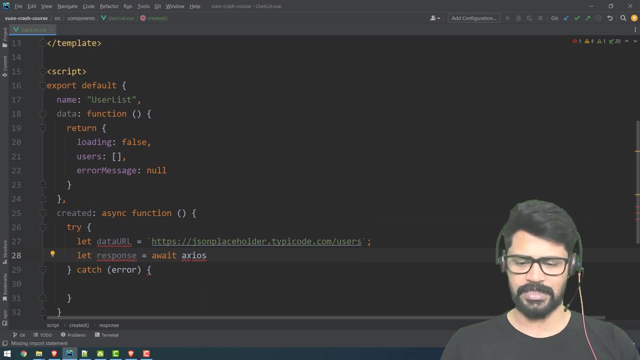 can we make this async for server call so and make try and catch this will become the error okay so here I need to say let data URL is equal to so what is the data URL for fetching data this one this one placeholder slash users okay now let response is equal to await axios you need to import axios from the library column axios so axios dot get of data URL okay you get the response and this response I 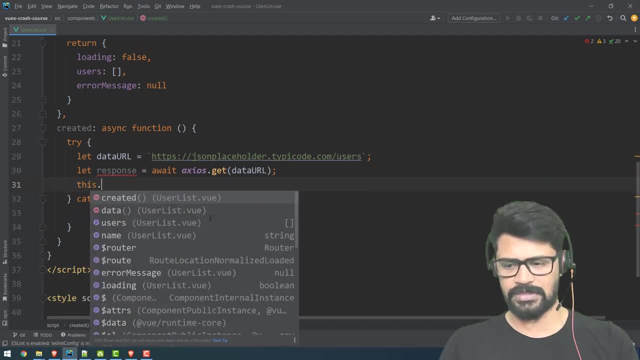 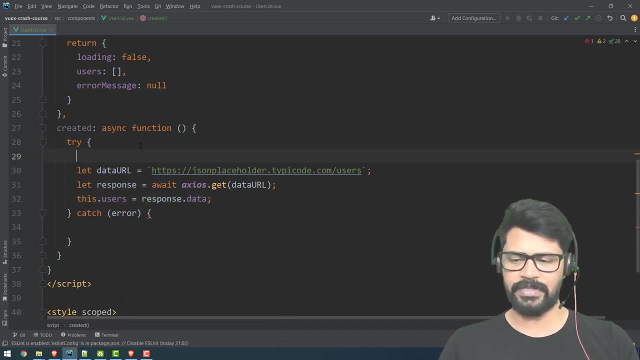 need to set to my local so this dot users is equal to respond dot data okay and I also make the loading flag so this dot loading is equal to true for loading spinner and as soon as you receive data you make this loading to false for stop the spinner 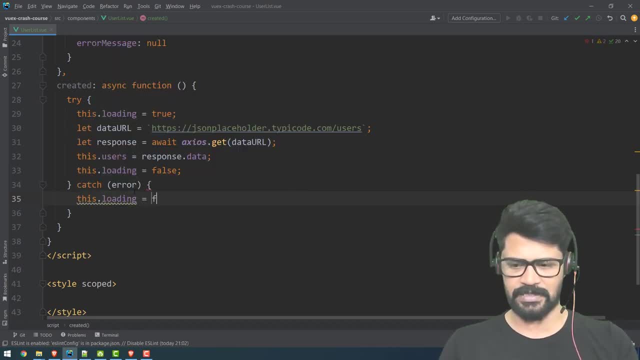 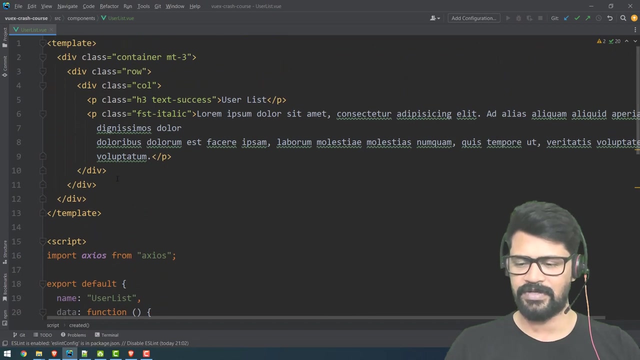 and lastly if you get the error also I'll stop the spinner is equal to false and this dot error message is equal to my error as well let's store this error data with error message okay fine now it's done so can we have a spinner 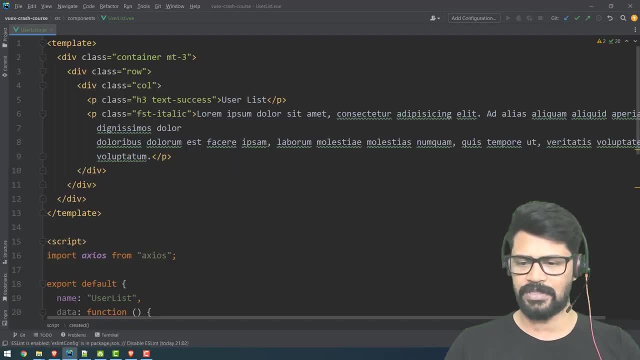 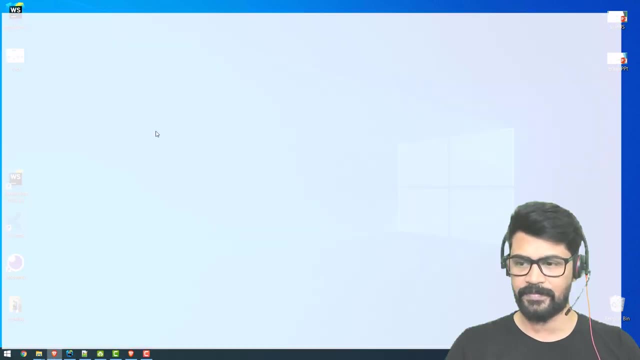 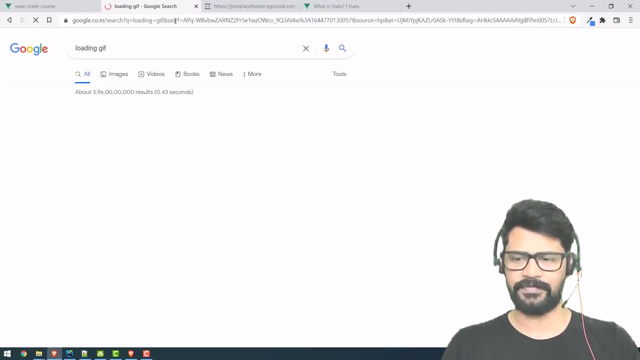 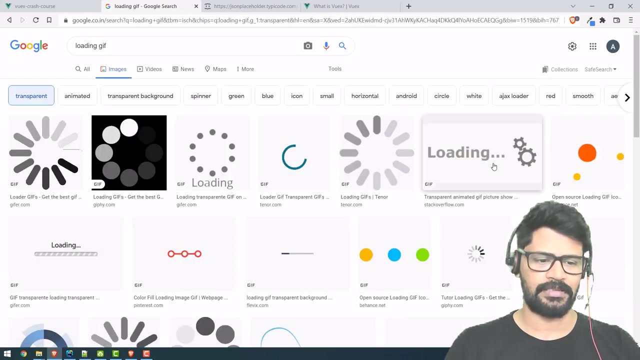 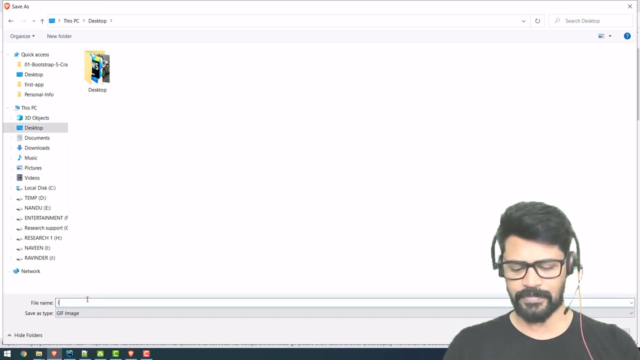 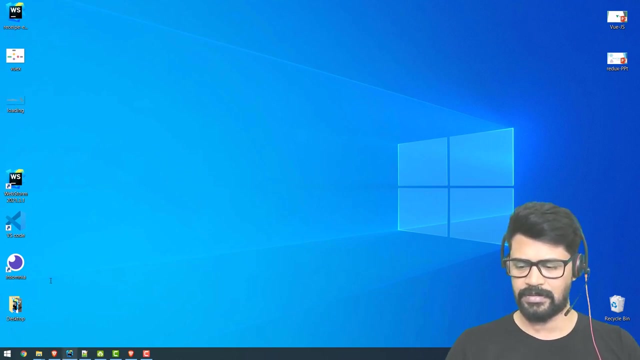 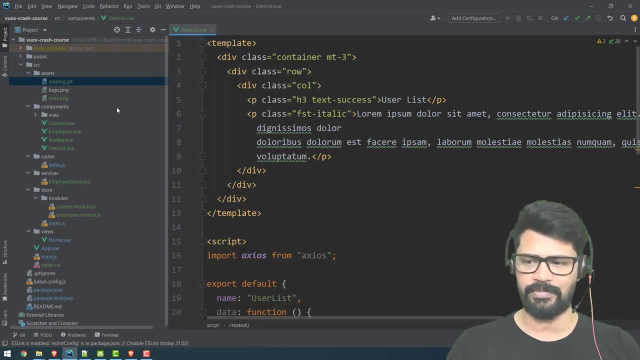 component with while for spinning okay I think we need to have a spinner you can just google search for spinner for example go to google loading jf magus transparent this one let me save images on my desktop loading let's copy this image keep it in assets folder and then paste it here so you can see see this is my image file that we made and now we need to paste it here and then we need to paste it here so the image file let's copy this image and paste it here copy this image stupid and paste it here and let's have this loading with one component so in components i create one more component 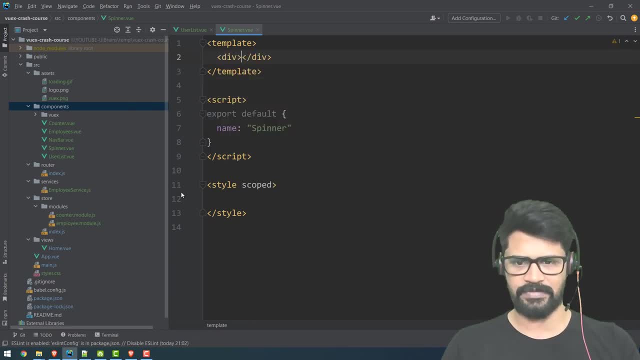 called spinner so i say a division with image src will be uh loader slash asset slash loading jf and let me give the class called margin auto and uh d block display lock okay so this is a spinner uh you want to see the spinner how it looks like 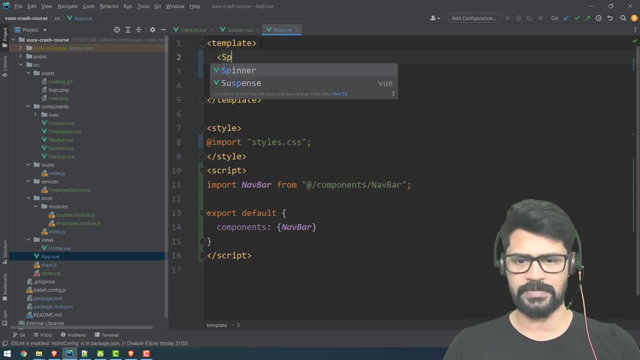 you go to app okay above the navbar you write a spinner so here is the spinner it looks like 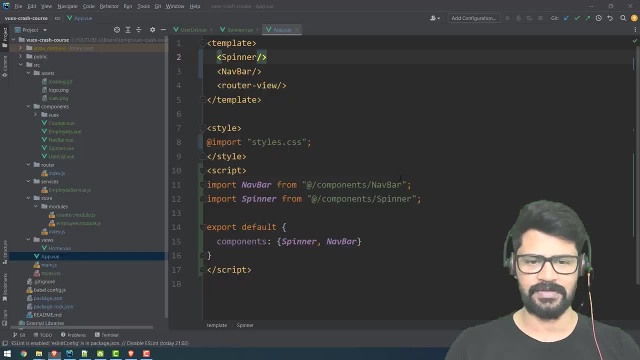 okay this spinner to display while fetching data from server so i don't need this 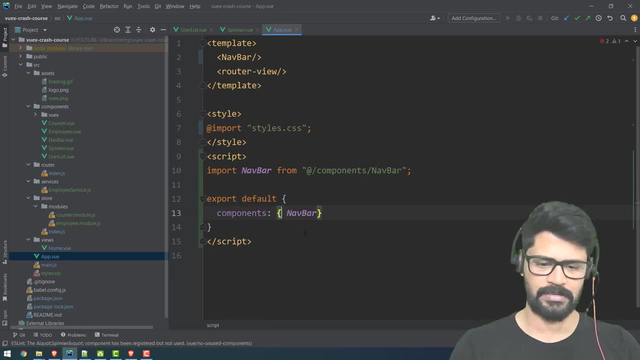 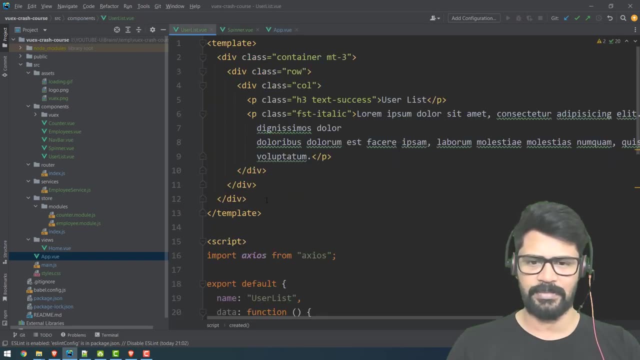 okay no import statement okay so for user list i have to display the spinner also yeah um this is one container 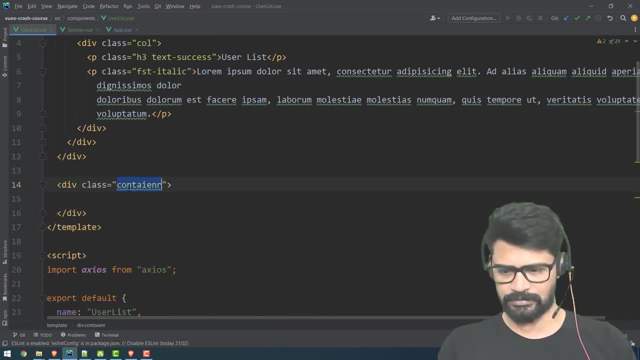 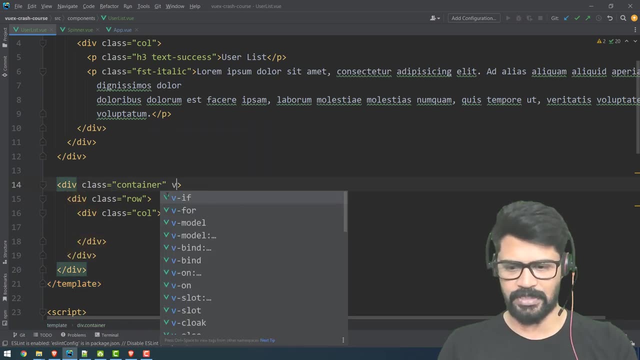 so one more container one container one row single column i write here v if 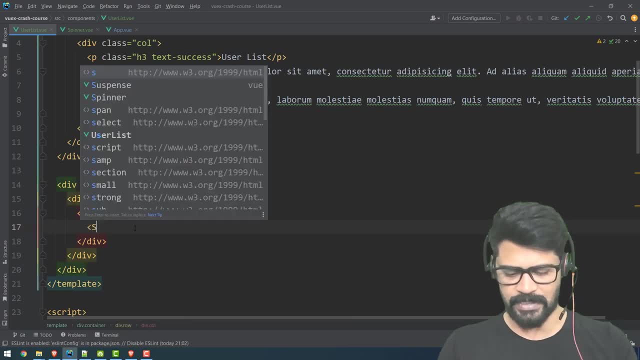 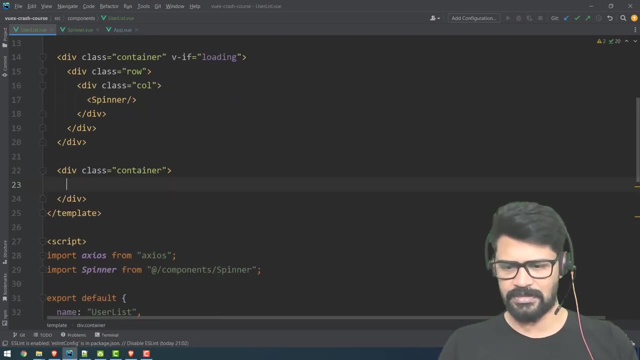 if it is loading okay if it is loading i'll display the spinner okay nice and for error message okay i write v if condition if not loading and there is an error 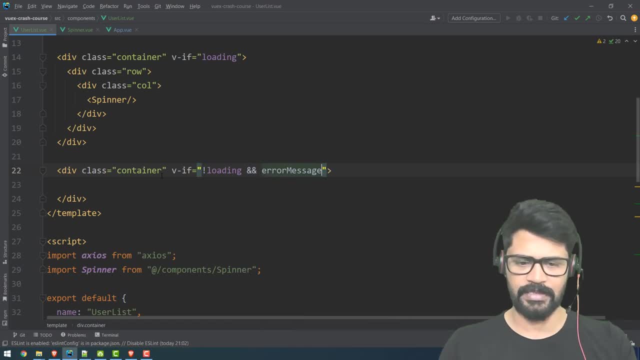 message if there is another message so um row column let's say p the class want with bold and text danger let's say the message okay so we got loading error message is also loading error message error message let's on that if if let's take a look that's running top of that range yes let's say this one error message now let's see let's say p all custom AP and field unid Infinix 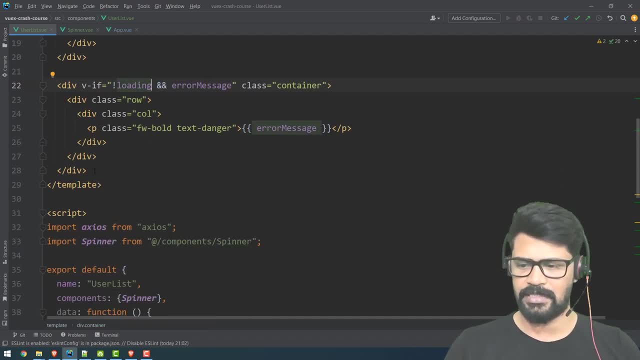 okay so this is to monitor if there is an error message if there is an error message i've typed this message I don't know i don't know very well there is a message for error message if it is going like this error message is done and then now quickly write your data to container one 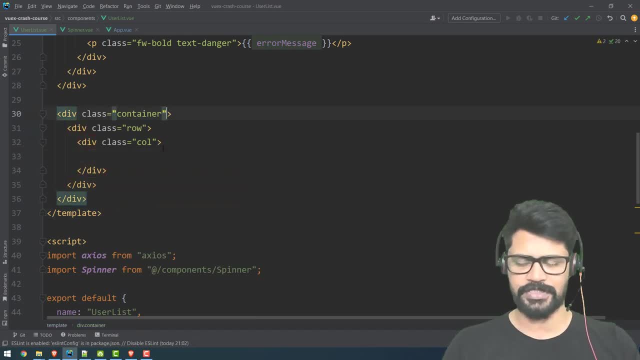 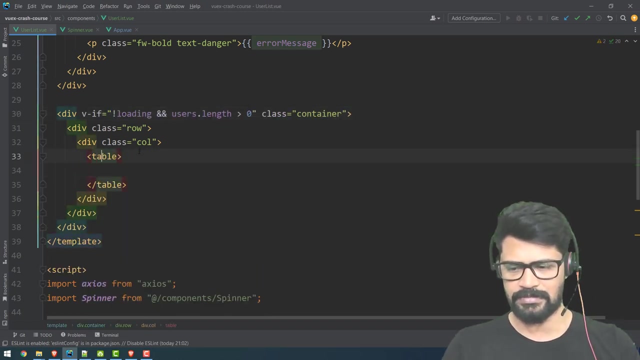 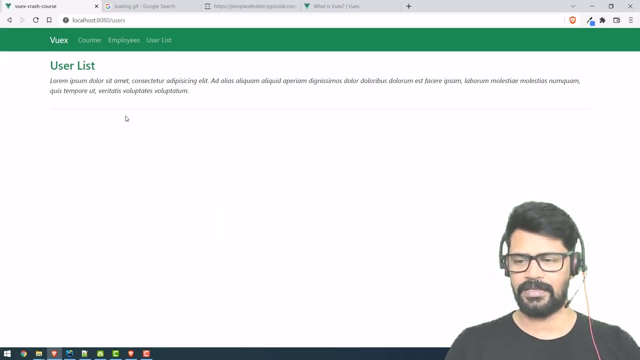 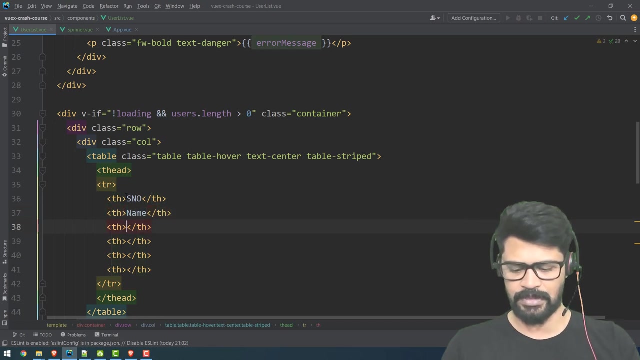 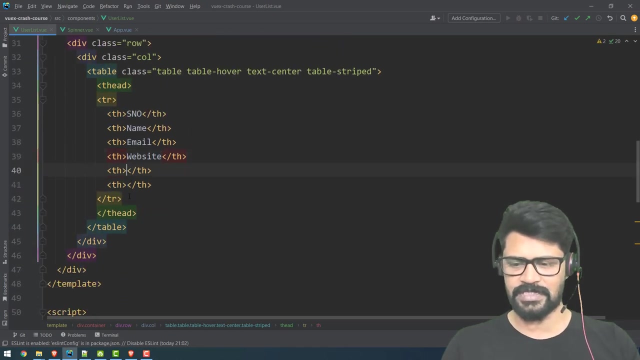 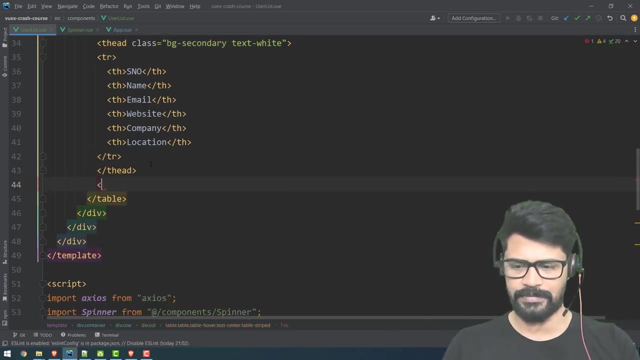 more row single column here I write a condition is we if not loading and users dot length is greater than zero okay more data then display so let's start with a table table table over text center and table striped okay yeah I wrote the head T T T table row th star sit staff okay so I need to have this serial number and name of the person email of the person opinion a table I want to leave that table so I need a table go and go with progressively I noticed tabcial but we want to create a table so we need walking table table tab run consider elements which is in order to야 get knew I guess website of the person website of the person and company of the person and location okay this data was there in here okay so for T head I'll give the class or BG secondary and text white okay and let's have data have you have data I have two bodies table row that we loop it so vi4 an employee is a user in 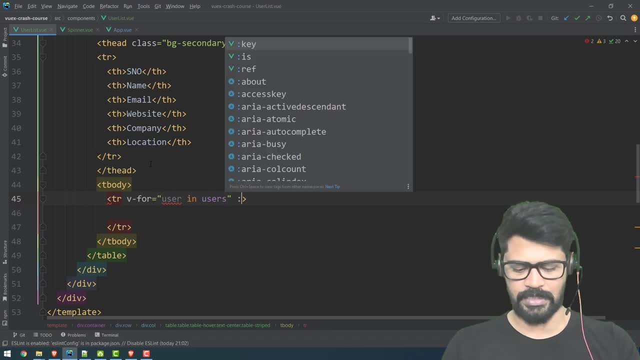 users and the key he is user user 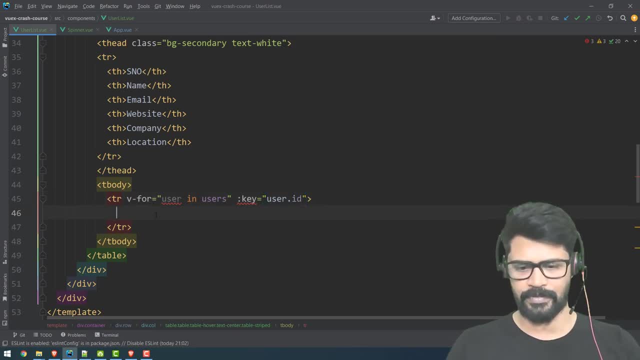 dot ID okay so can I have TD expression let's say user dot ID okay so you get 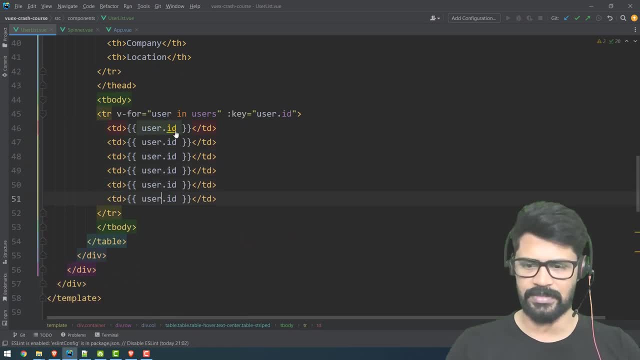 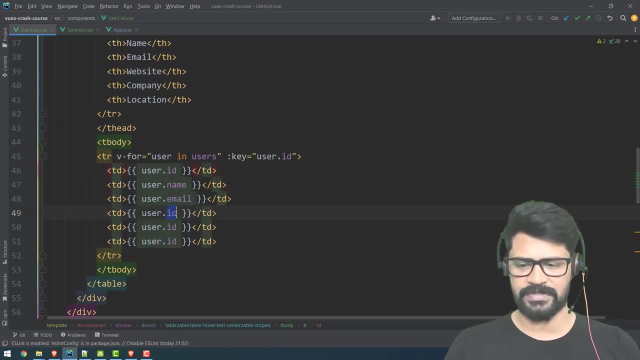 all the user IDs and let's make name and on so can we write name email website 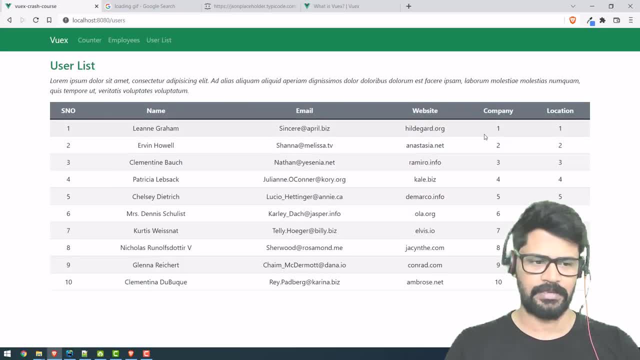 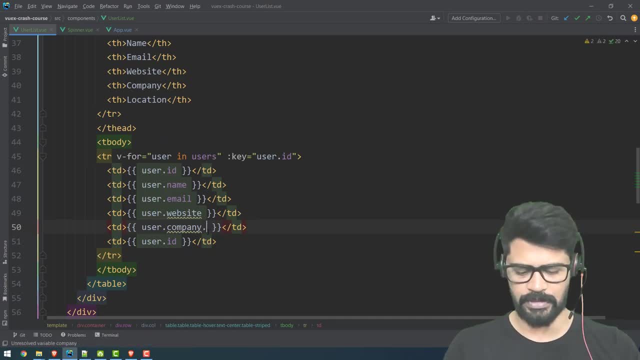 website and company what company is actually an object so I need this name of a company dot name and location I think it's address address also an 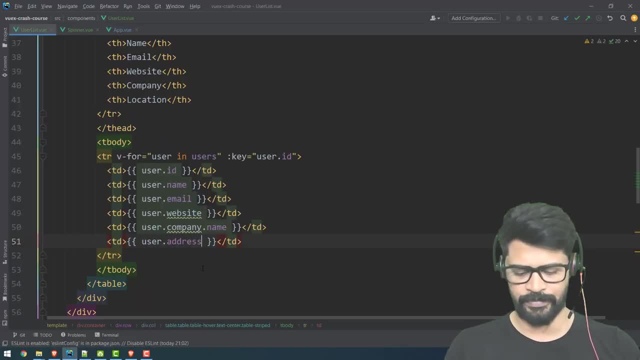 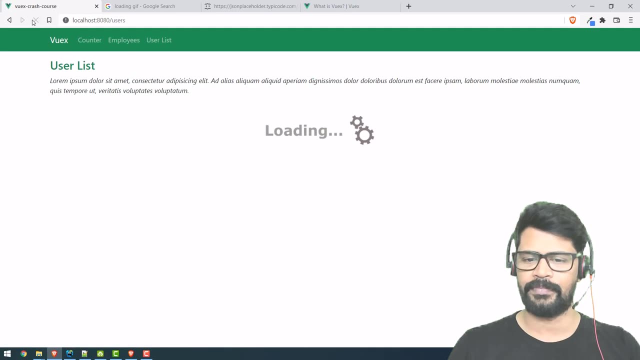 object address dot city get us all okay fine see you get the loading flag see you get the loading flag see you get the loading flag see 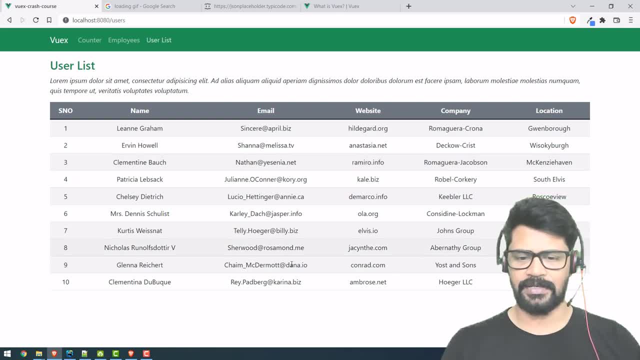 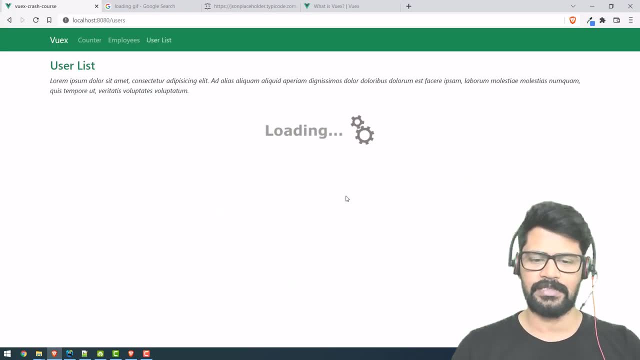 i got loading flag and also the content and also let me check the error message so can we have this some wrong url so that see you get the error message also if something goes wrong so 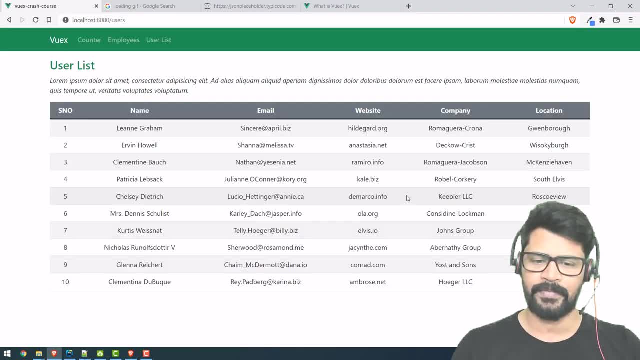 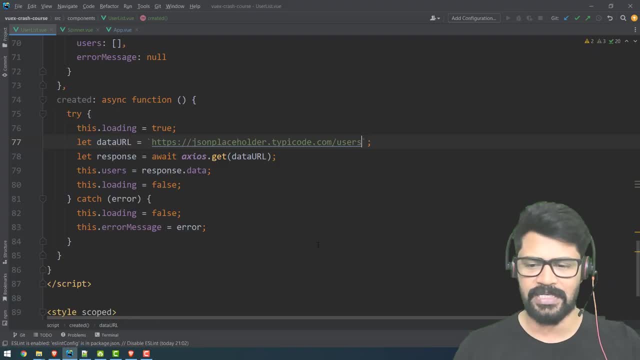 this properly works yep so this component is ready with the regular server connection and fetching data that a local because my have my data is still local okay now so now the concept 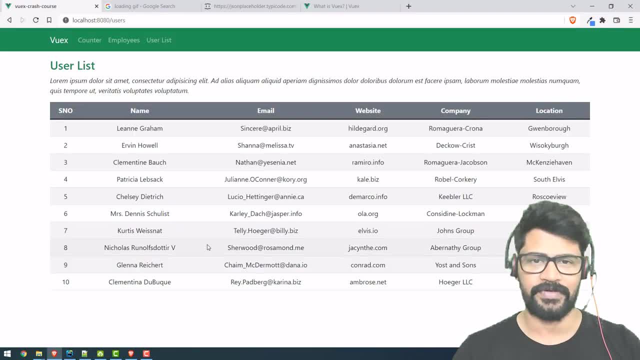 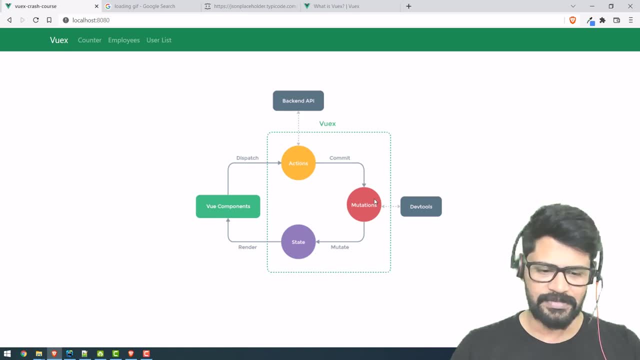 is how to make the same example for fetching data from server because the complete flow will see now okay from the back-end API to the action mutation state and your component so how to make this 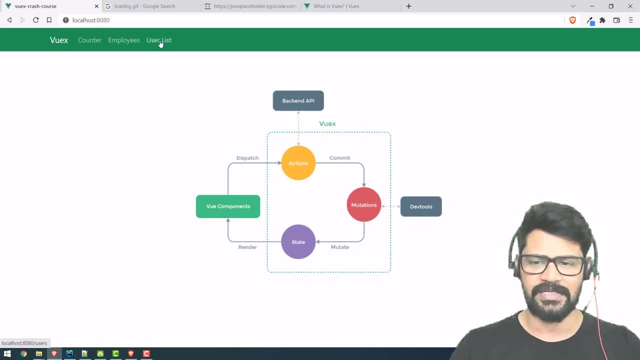 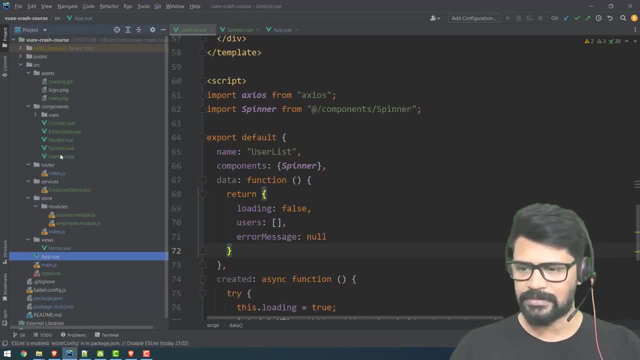 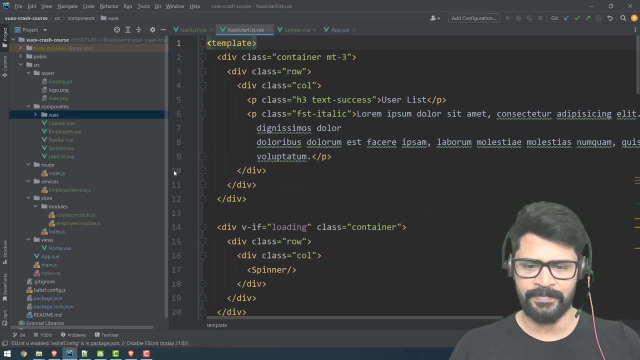 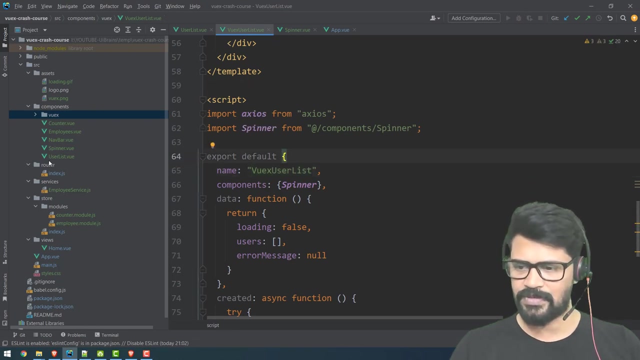 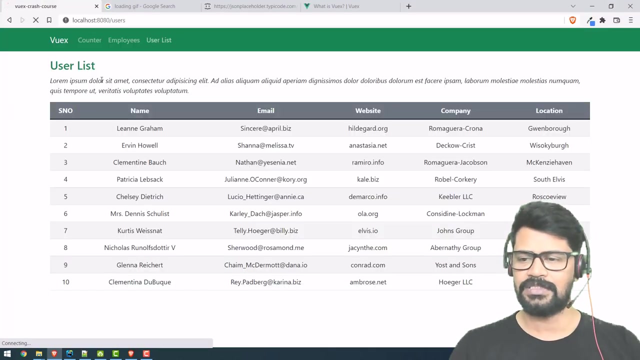 complete story with user userless so to start with that I just take a copy of the same component copy userless paste it in the UX with the name called UX okay I'll change the name to UX userless and I go to the router once and saying this also UX userless okay so now this is become a view X userless data is is perfectly working fine so now let's 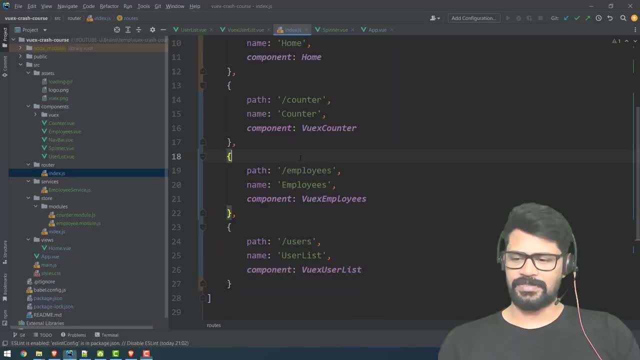 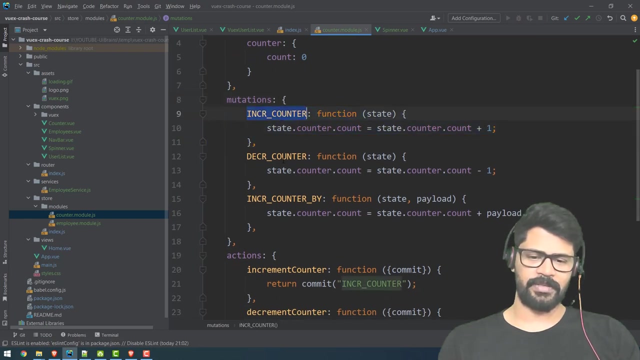 make this to happen with a view X configuration so to start with UX for this server connection see when you when you look at the previous example of employee or counter that was local state change so we just have only a function for increment counter decrement counter the actual mutation right but for fetching data from server you have three set of mutations okay so one is 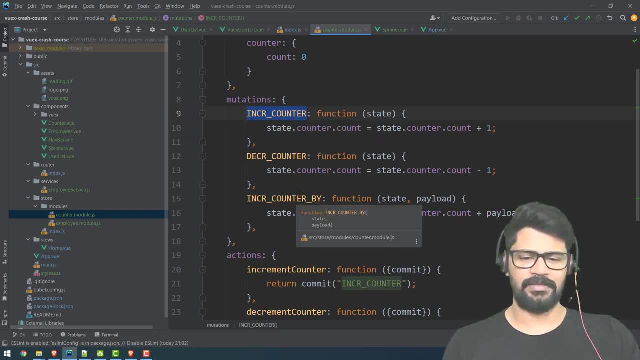 for normal request and one is for success one is for failure because we need login flag and we need data we need the error so three things required so three set of mutations required for every API call okay so I'll I'll start with that so let's close all 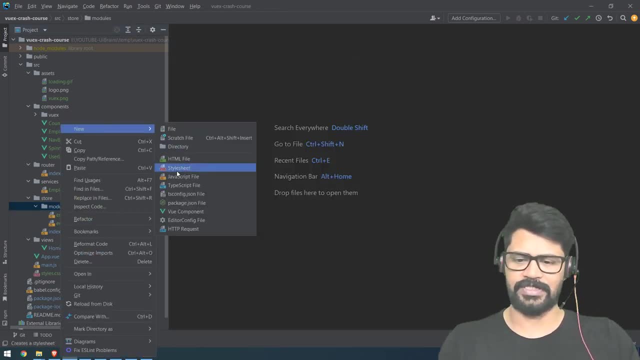 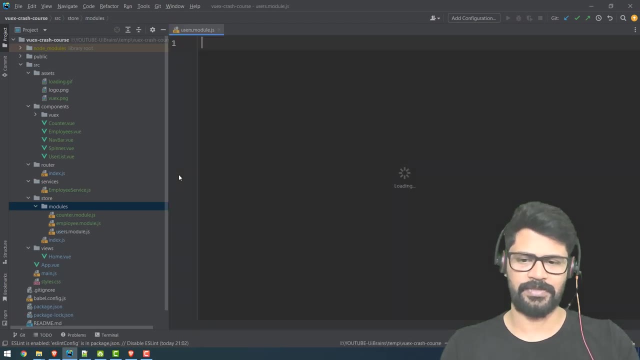 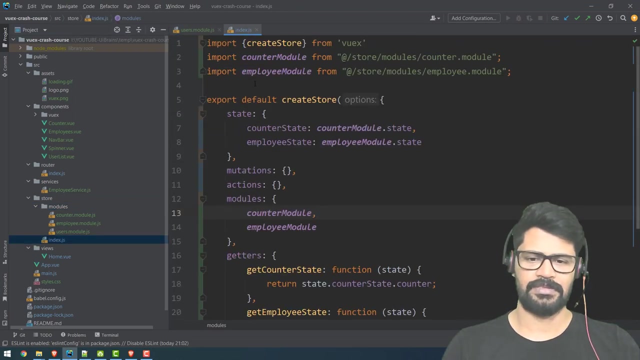 the tabs yeah in modules I create one fresh javascript that is users dot module not user list dot module so export default something so in that I need name space it is true okay so you to have a state and actions sorry order doesn't matter mutations state mutations and actions okay so let me just connect with the global store same like here 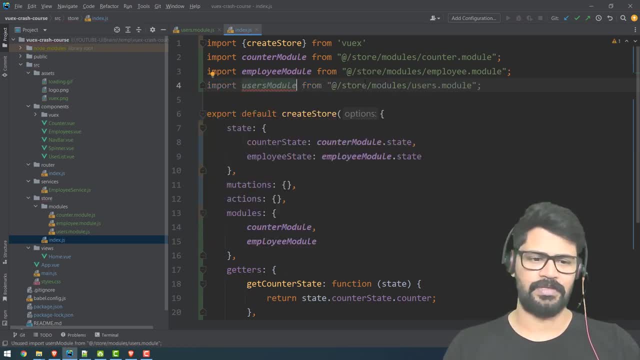 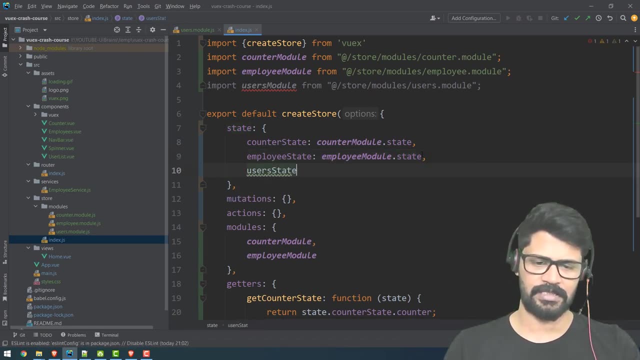 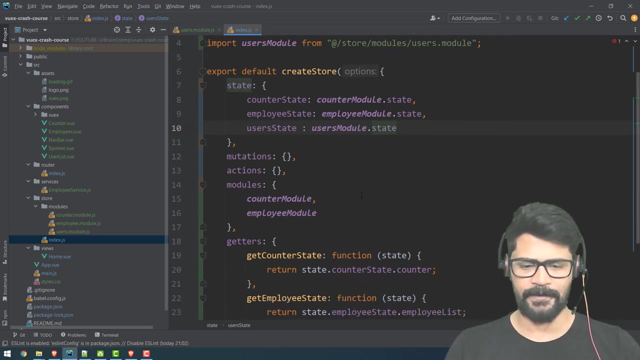 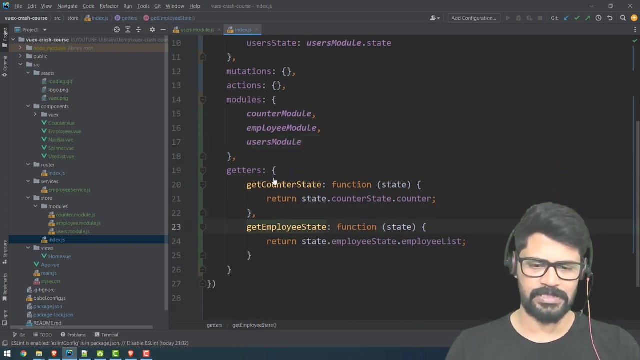 import user module from users dot module and let's say users users state will be user module dot state user module dot state okay and let's configure the module users module okay getter will write in future because we don't have anything now okay so for state I'll say use 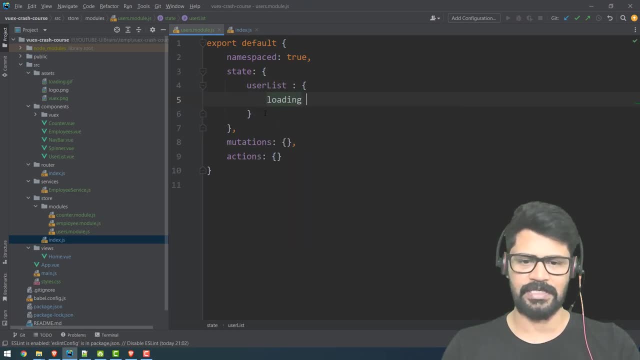 user list will have three things what is that loading okay loading users and error message it should be null okay so when you start with mutation I have three set of mutations just for fetching 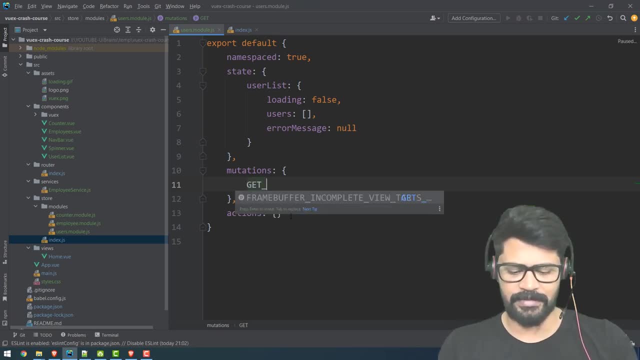 data only but three set of mutations so what is that is get users request is one mutation 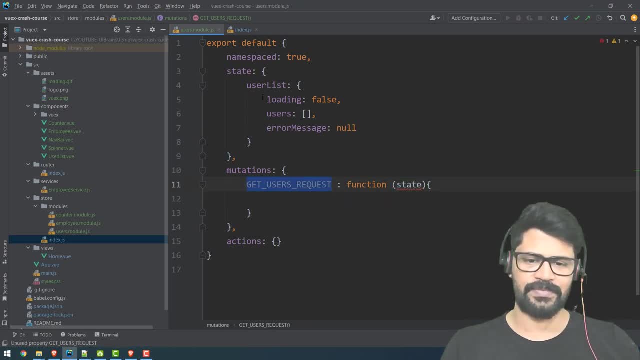 what is does is it just take the state this is just for loading flag okay so it's make state dot user list dot loading is equal to true 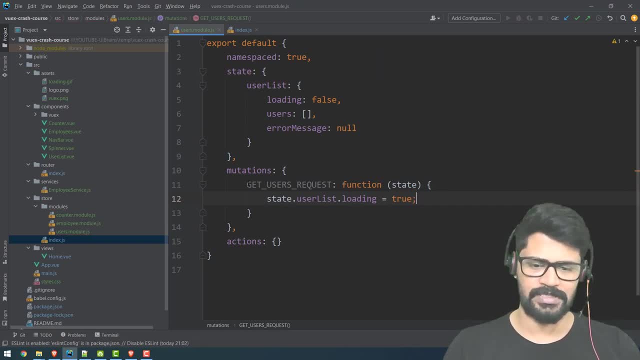 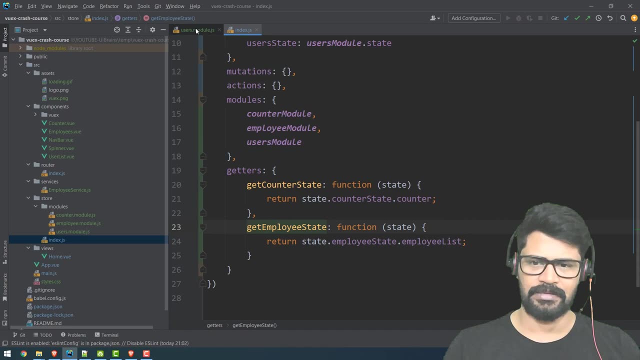 that's all simple nothing much okay this is your one one mutation okay next uh uh yeah 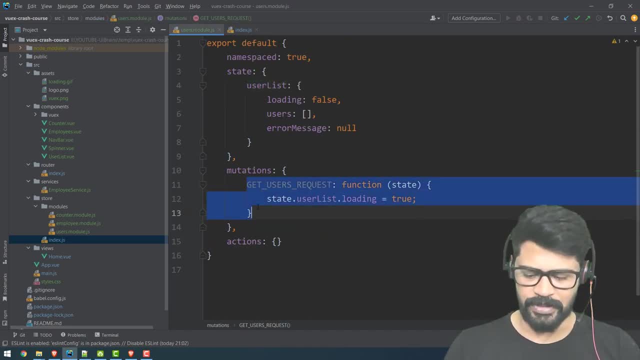 so next thing is for success so I'll copy so get users 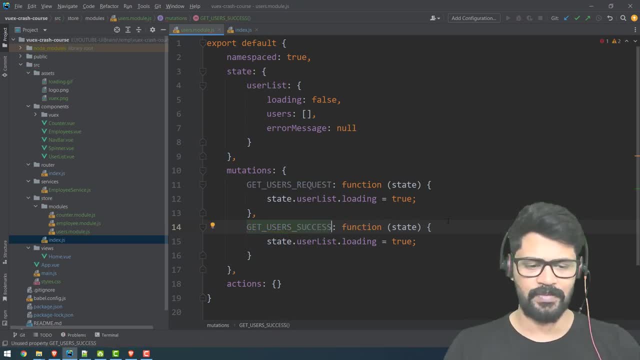 success when you get successful data what you do you get the payload from successful data so first I'll make loading fall to stop the 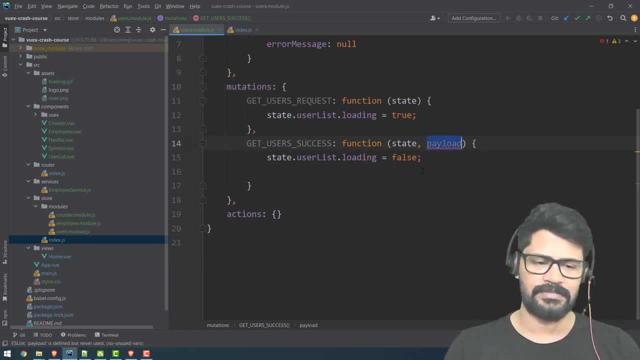 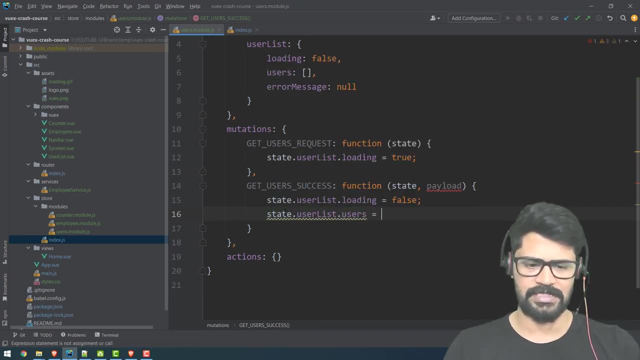 spinner and I see the payload data that I need to add to users so state dot users list dot users is equal to payload dot users okay payload must be an object which contains users which 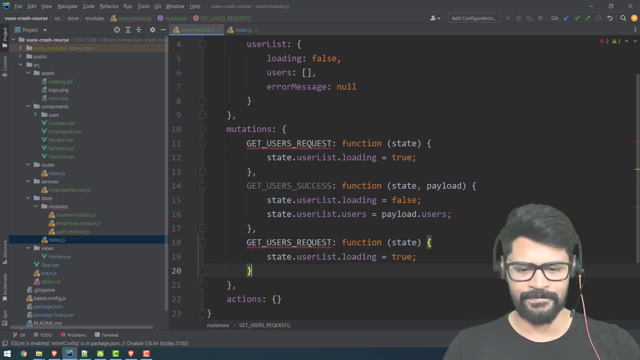 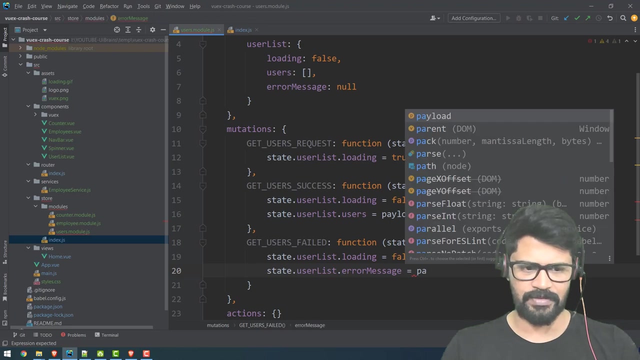 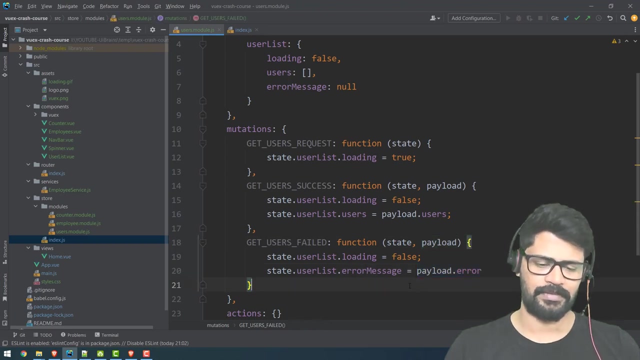 your data and one last thing get users failed okay request success failed so if it is failed i need to have a error message so i also have payload okay loading become false and the state dot userless dot error message will be payload dot error okay payload now this time provide the error okay 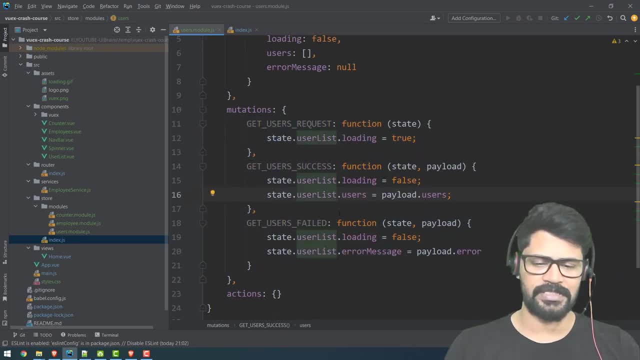 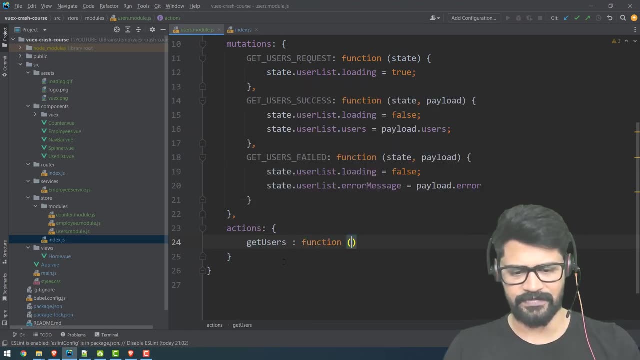 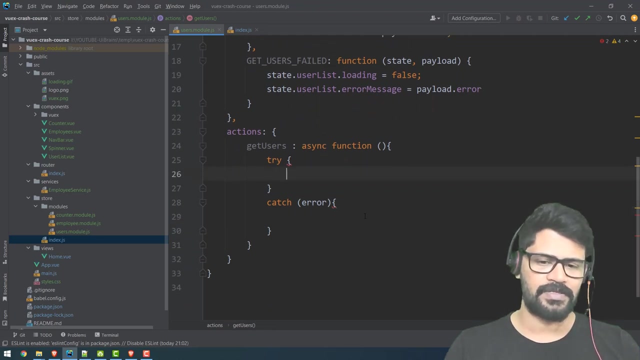 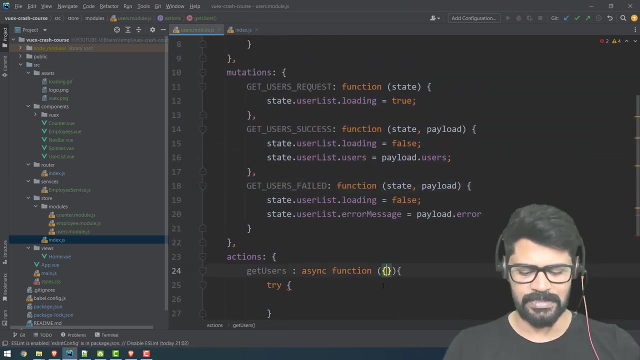 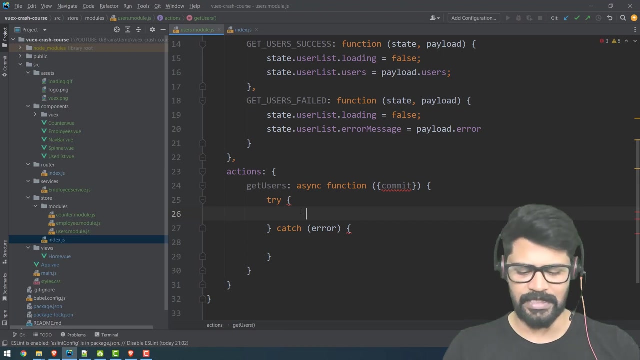 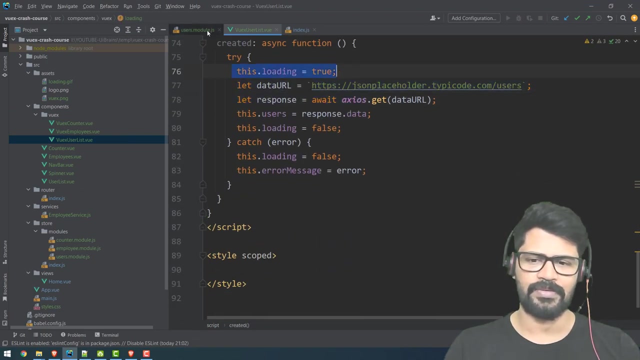 fine so three mutations is done so all the three mutations i'll make with only one action okay let's see get users is one action which contains a function so this is asynchronous okay in this i have some try catch yeah here i'll make a server call based on the result of server call i'll i'll commit these uh you know these mutations so let's take the commit commit okay so first of all i'll commit the regular one see generally what happens is if you go to the component here in in user is what you are doing before i make server call i make loading to true right so same thing i'm i'm doing 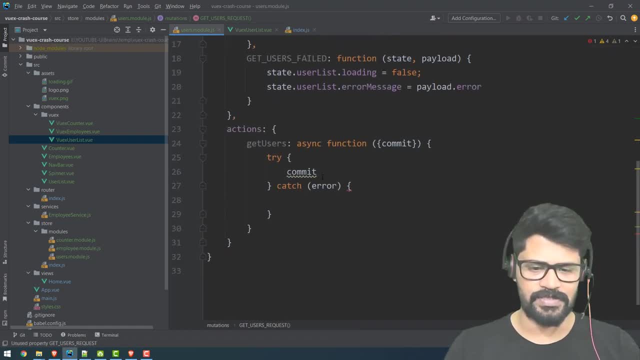 see that loading true happens with this mutation so i'm committing that mutation first 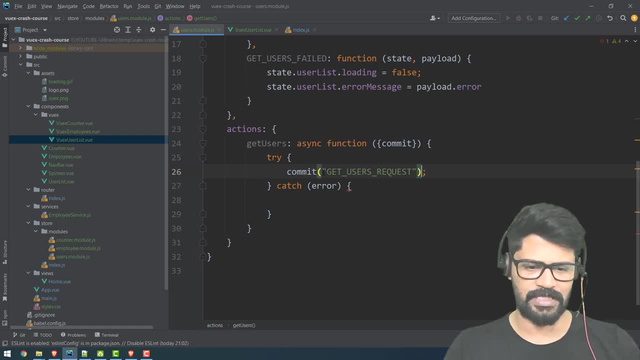 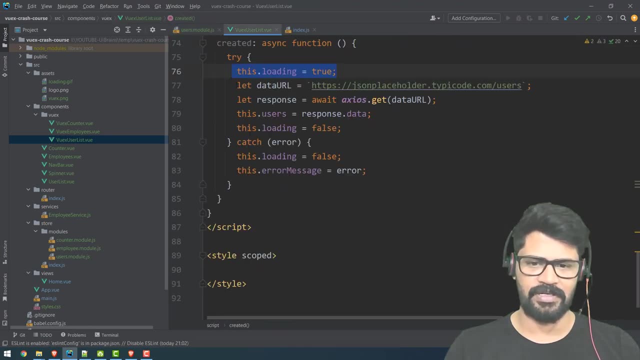 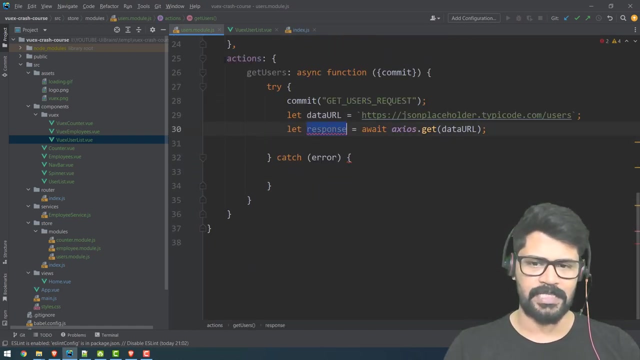 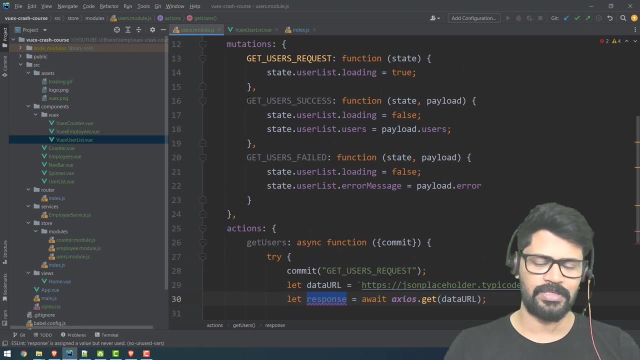 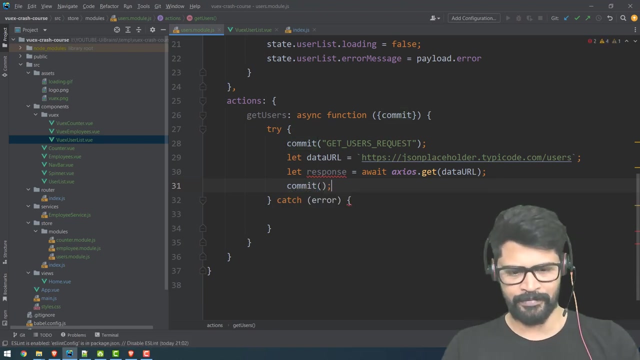 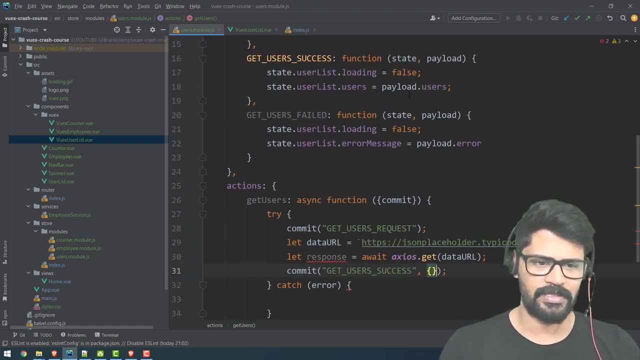 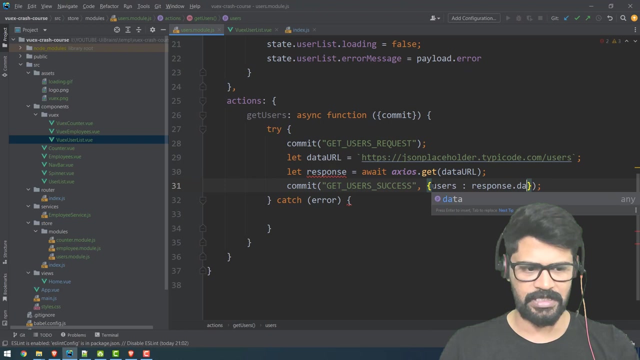 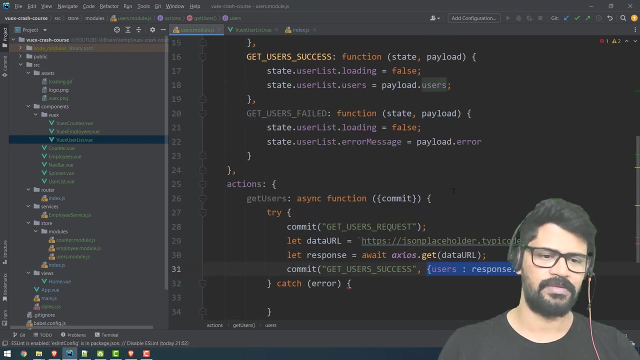 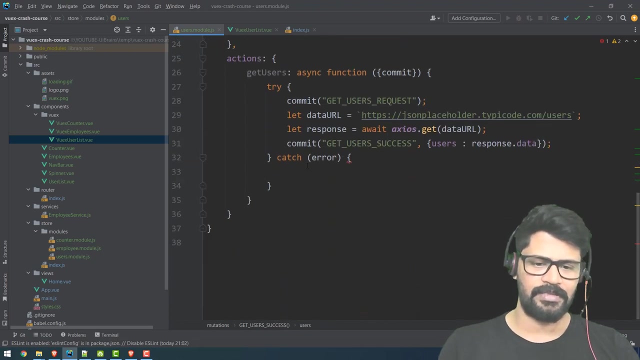 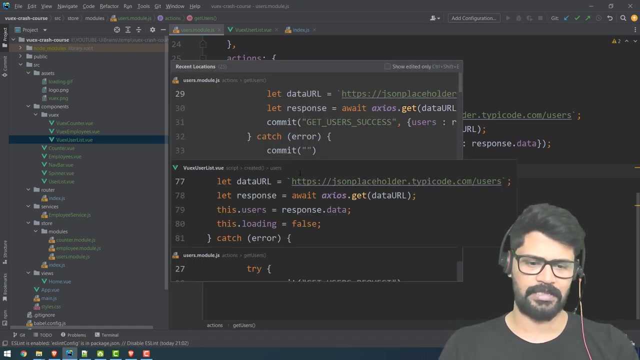 so get users request okay then and after that after that let's make a server call how you make a server call let data url and response same story you get the response and this response.data you're adding to users right but how i'm adding you can't add here you get this need to invoke or commit this action so payload will add so i'll make like this commit commit get user success and the payload will be an object because you are looking for an object with users so users will be respond.data the data which you get from server response.data i am just adding to the object with the property called users and this whole thing is payload and that payload will receive here and payload dot users i'm retrieving the property and adding to the state data okay and lastly when you commit the error say commit uh get sorry get users failed 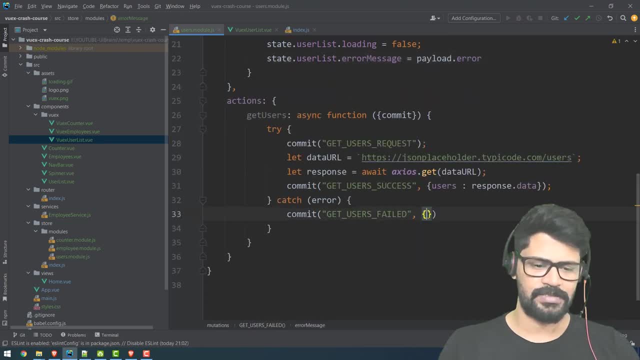 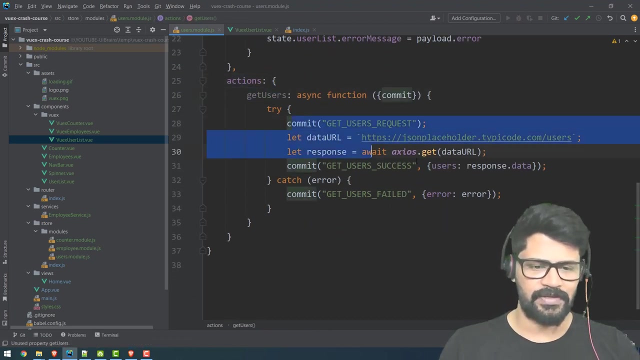 and here also see it looking for payload.error so i make this is a payload and here error will be my error that's all okay this error will be taken payload.error and to the state okay that's all so now just only one action which internally calling a 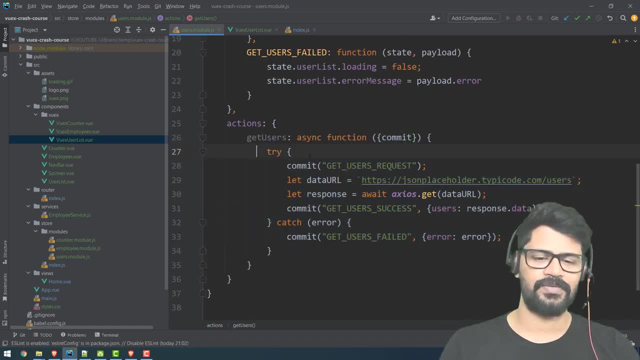 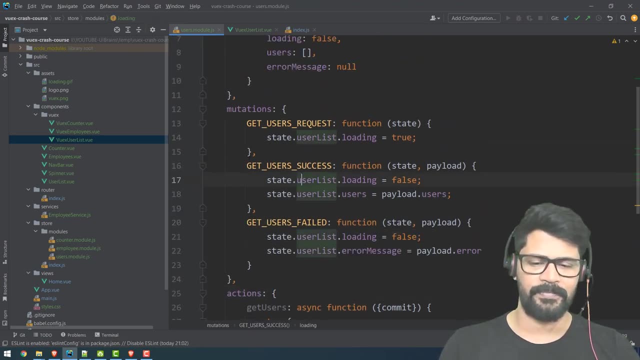 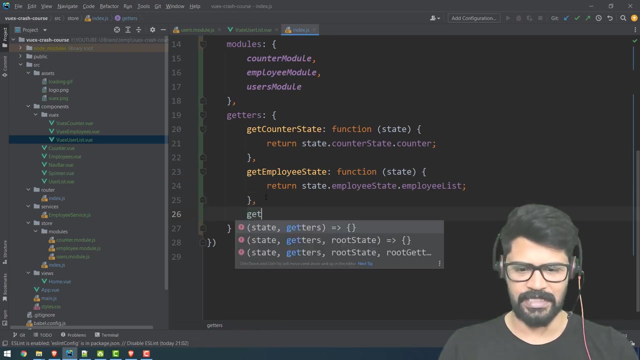 three set of mutations okay this is the way you have to call uh um for fetching data from server especially for api calls okay yep so this file is done but i need to make getters yeah so let's say get users state get user state is equal to a function which access to the state 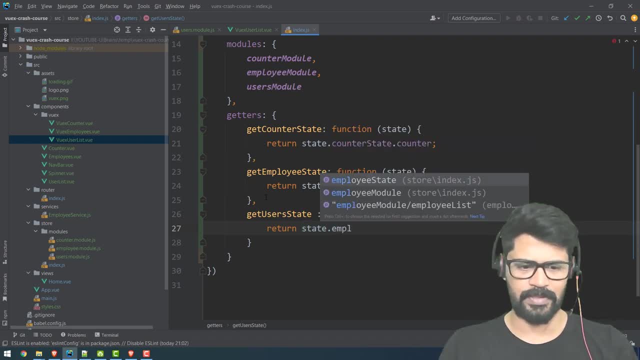 so return state dot employee not employee i think it's user state dot user list yes that's all 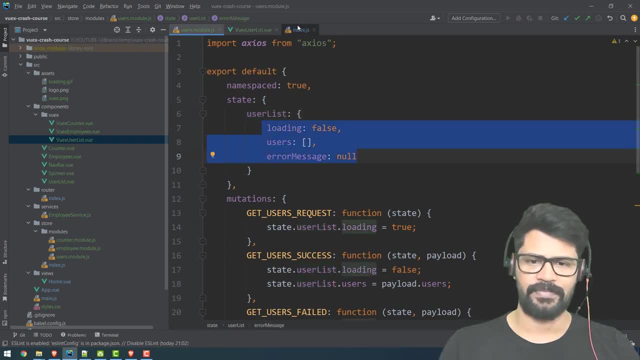 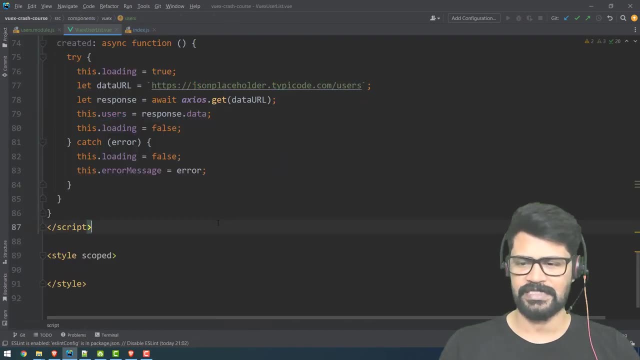 you go to user list you have all the three okay so getter is ready uh file is ready move on to user list view x yep so here um i don't need data for yeah how you get data from server data okay so i'm going to use data from server data 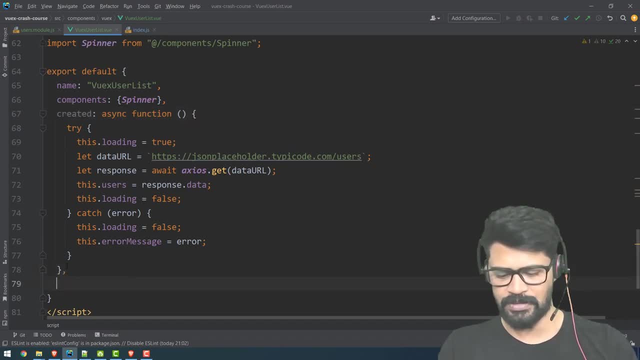 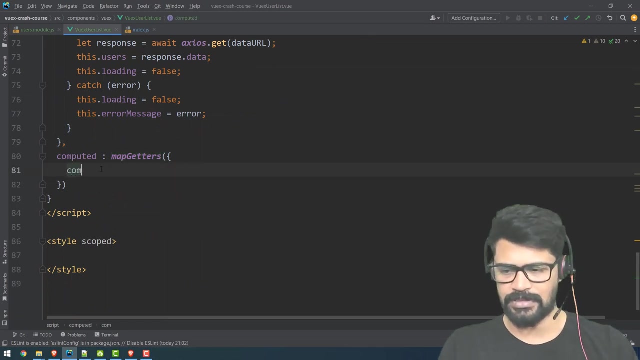 get data then you need to compound the completed property of map getters from view x so here i'll say so what is the property you have to map uh some your own uh let's say user state will be that's a user state or users state whatever will be uh the method name should be proper what is that 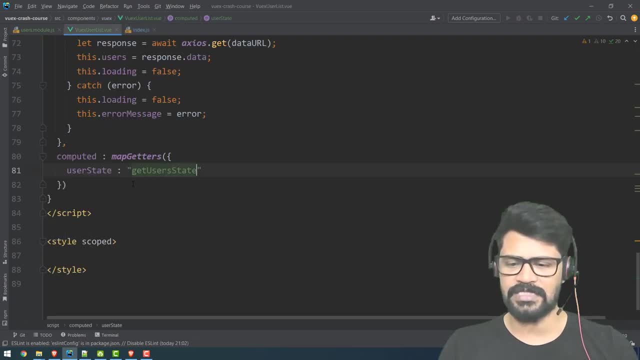 get user state get users state you can access the user state and which contains everything 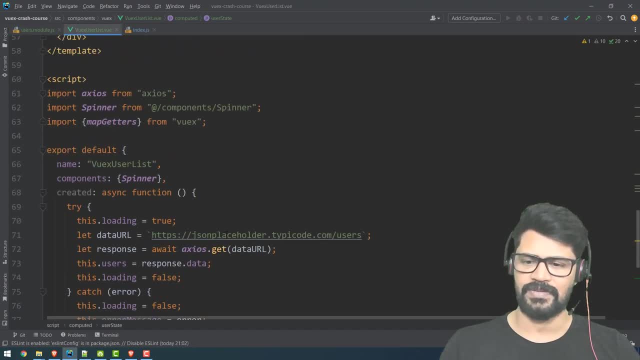 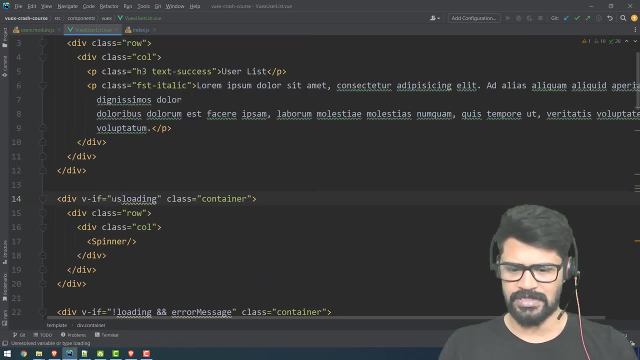 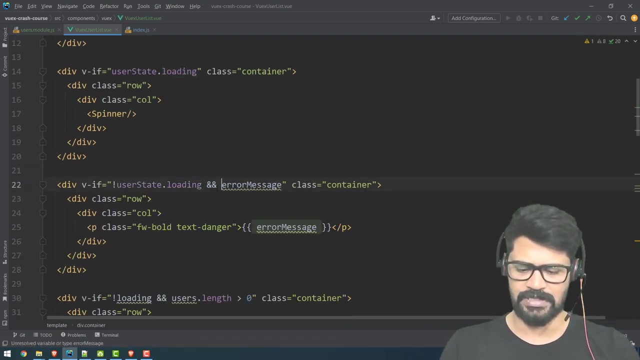 loading users error message so when i go back here this is what yeah loading this is user state dot loading this is user state dot loading and user state dot error message 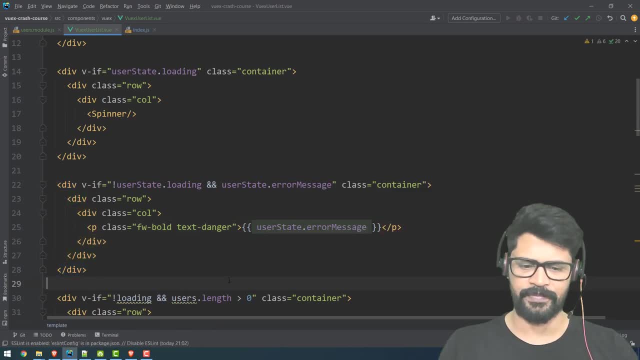 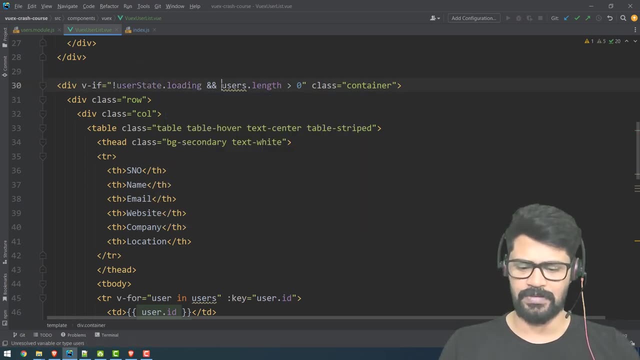 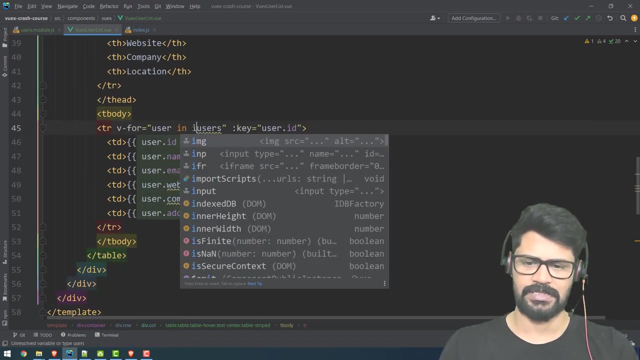 display also user state dot error message and lastly here user state dot loading again user state dot users what else here also users uh user state dot users okay that's all 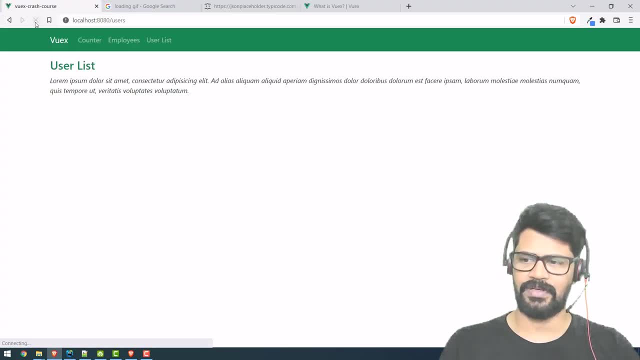 so now check oh uh you don't have data problem why you don't have data because users module is there 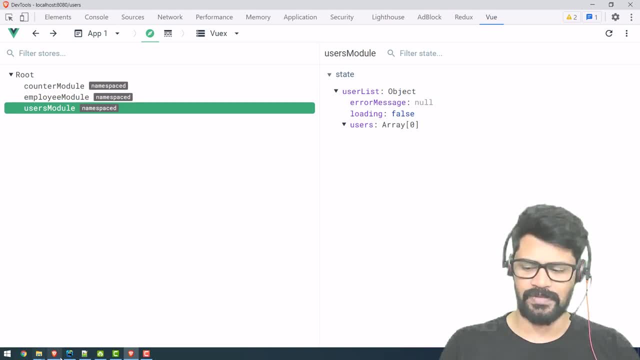 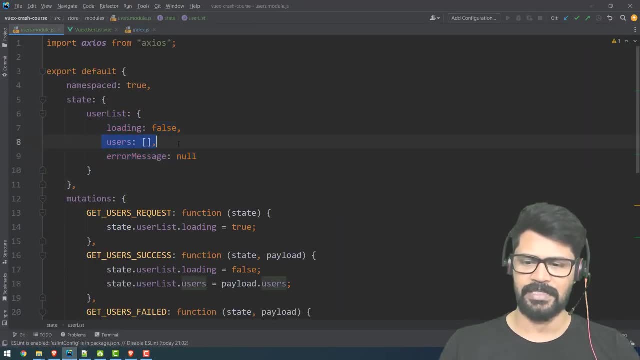 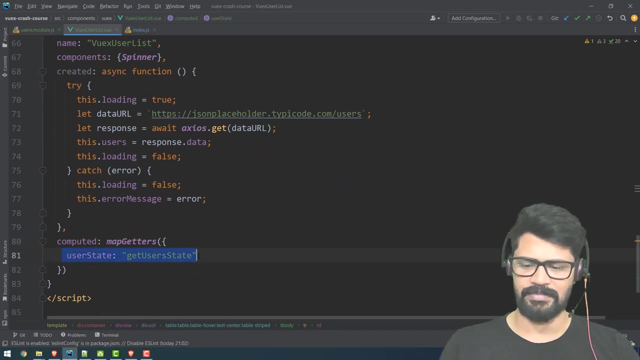 array with empty because why you know you are only fetching empty data because in my store i have this empty array i have this empty i i fetch i just brought data right empty data but you know dispatch an action for fetching actual data right you know dispatch this action for pitching actual data so simply what you do is you just dispatch an action for fetching data and you 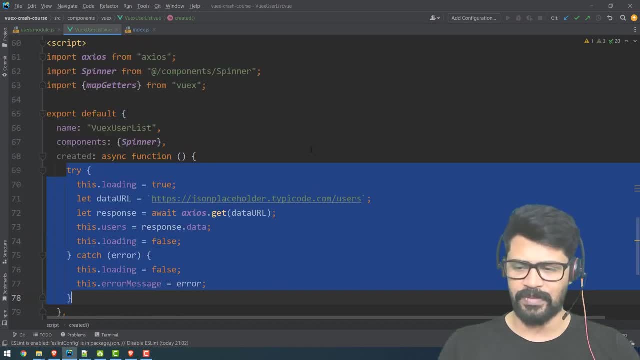 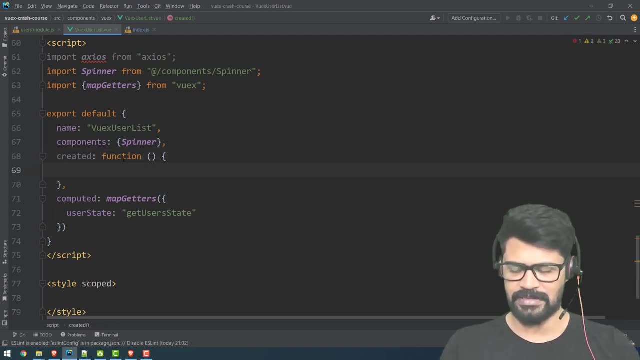 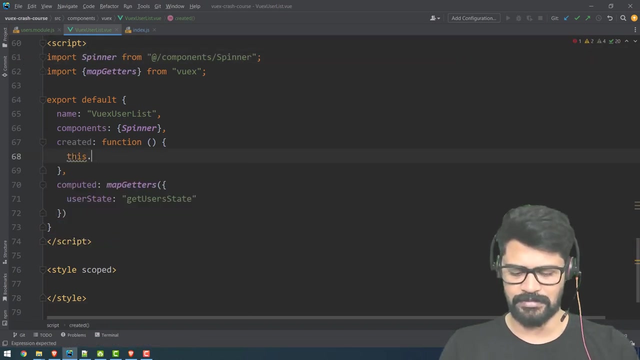 it is created when this is created I'll dispatch okay simply I'll dispatch the action so say relax use yeah here this dot dollar store dot dispatch my action what is that users module dot get users that's all simple the moment you make a 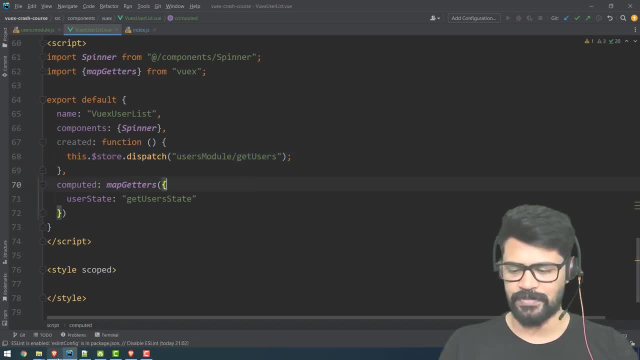 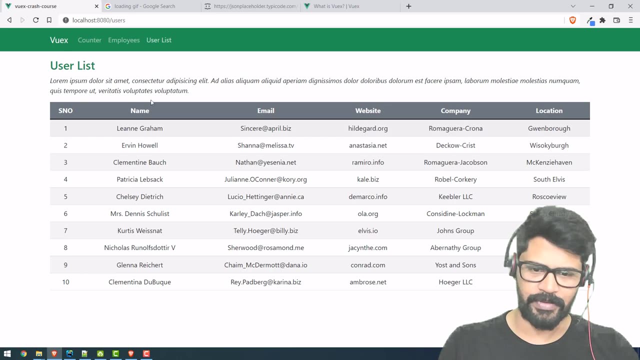 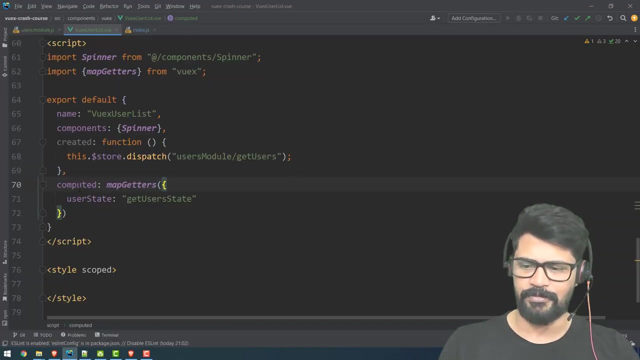 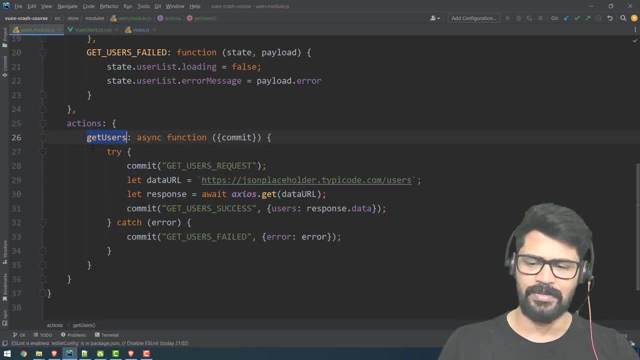 dispatch then it will see what happens I'll show you complete diagram now see they got data see from the component this is my component okay yeah see see the flow components you are dispatching an action see from the component component I am dispatching one action okay go inside the action what action does this action is committing this action depend on the back end of the action this action depends on the back end of the action base after the13th mutation what will the data is filed according to or 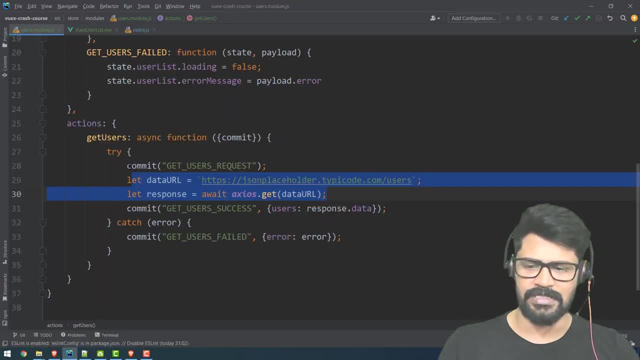 whatever the back-end API is have a connection with C my action have a 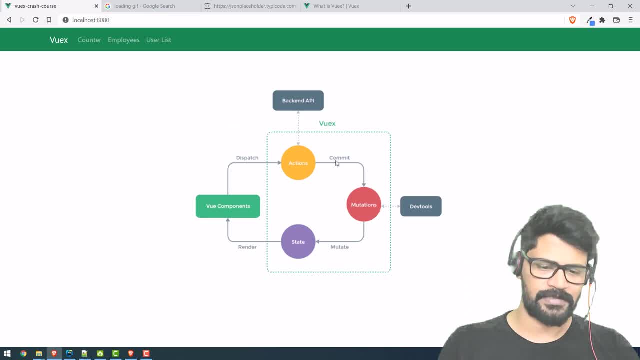 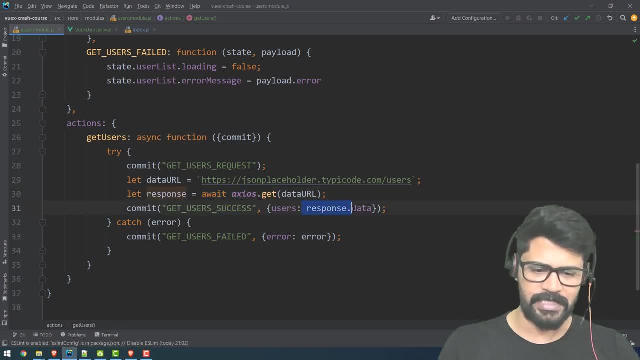 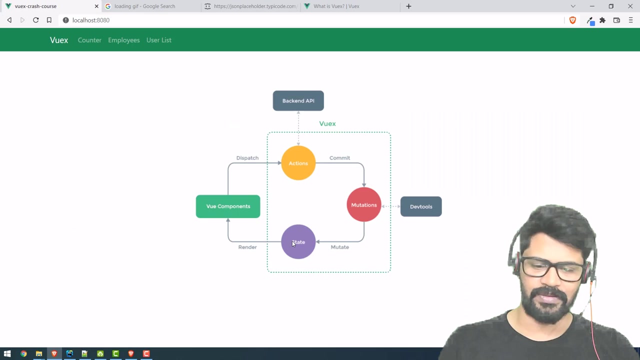 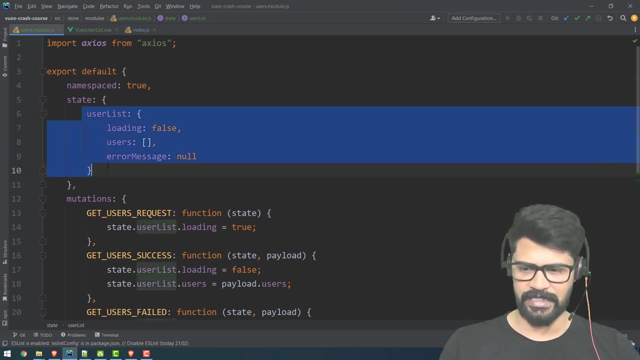 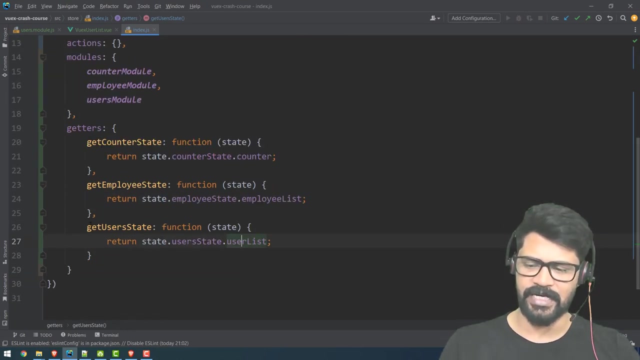 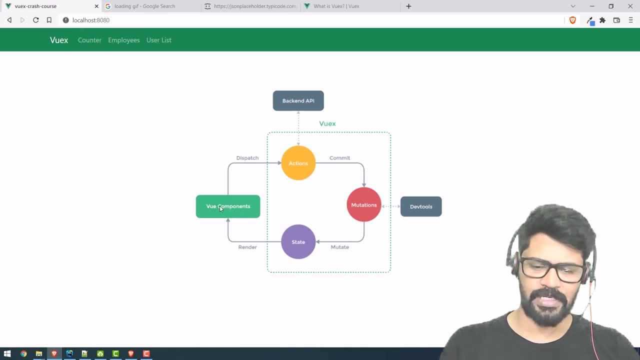 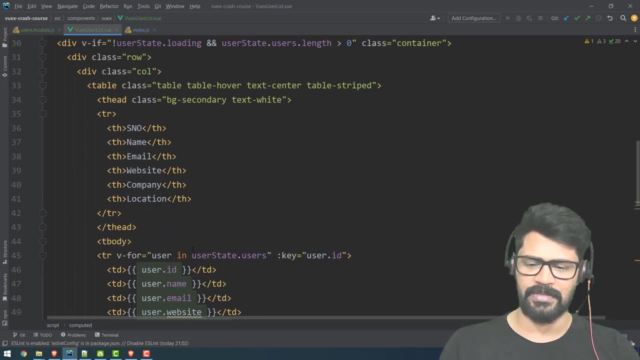 connection with the back-end API depend on that it is committing the mutation see it's committing one mutation to mutation third mutation depend on the responsibility it is committing the mutation and what happened for example you get successful data it is committing success and data so this mutation is the stator okay this is your global state okay it is updated and this state data how it is being injected to view component is this state data the whole module is configured to global store where you have a getter this is access to the user list stator and through that getter in the component using the map getter i am connected to my state so your component has connected with stator so through map getter you got a state and from that state only i am retrieving all this data so that's just where it's being connected so the complete flow has seen okay 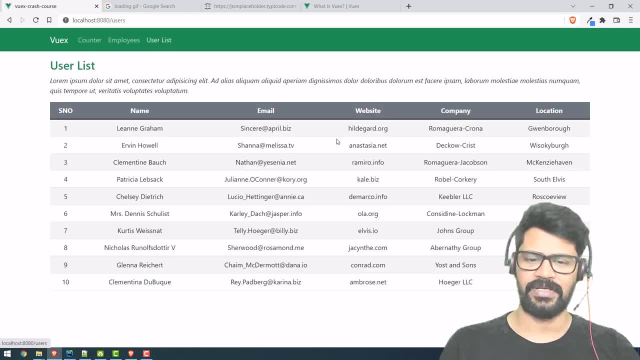 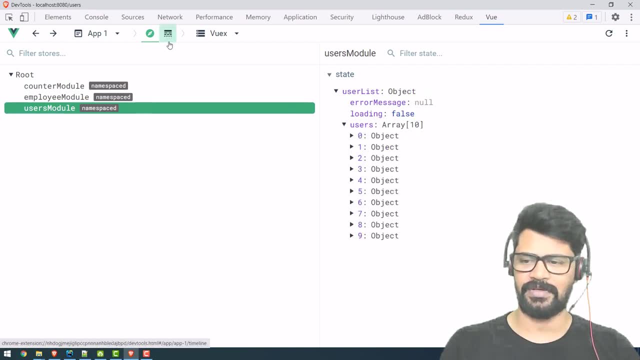 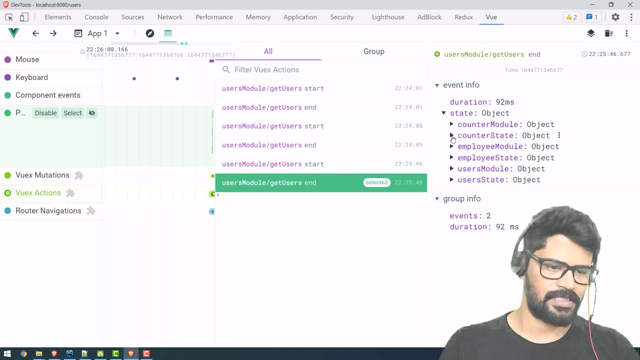 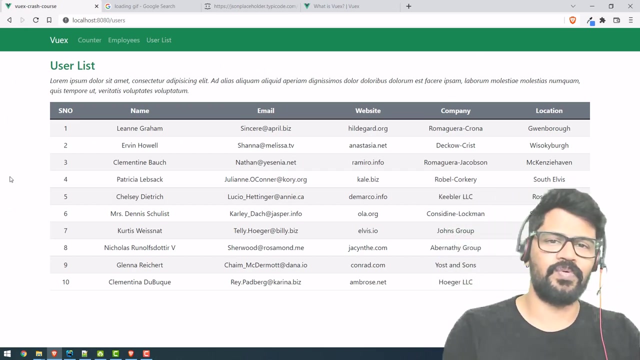 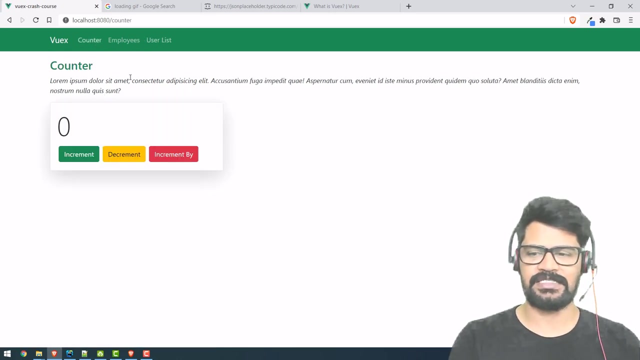 so now when you go to a user list loading flag and data when you go to dev tools also users module you have all records and you can even check the view js actions so get users start and you got the data okay users state user list all the list of users you have okay so this is how actually you can make a view x with view js application i hope you got this okay because we understand local state changes okay with regular you know you know